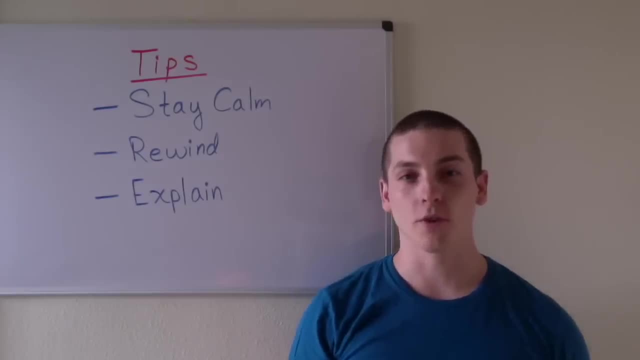 duck debugging, which is where programmers go through their code line by line, trying to identify bugs in their code by explaining it to a rubber ducky. So, similarly, if you go through the material of the videos subject by subject, you will soon be able to identify. 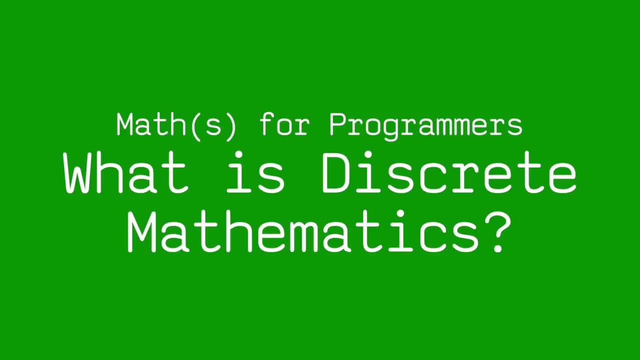 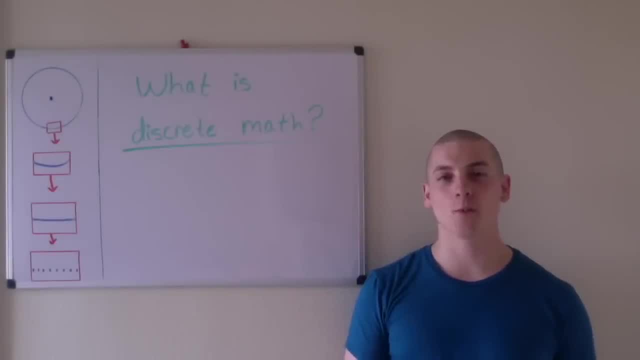 any gaps in your understanding of the material. In this video, I'll be explaining what discrete mathematics is and why it's important for the field of computer science and programming. Discrete mathematics is a branch of mathematics that deals with discrete or finite sets of elements, rather than continuous or infinite. 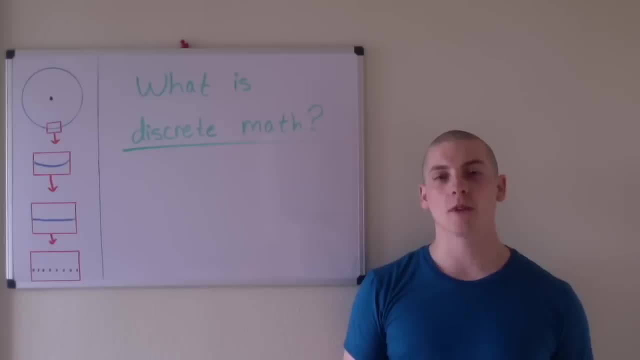 sets of elements. Imagine trying to run a program that requires an infinite number of executions to complete a task. It's obvious to say that the program would run forever and the task would never be completed because there are an infinite number of executions. In order to avoid this problem, we approximate the continuous sets with discrete sets. Now. 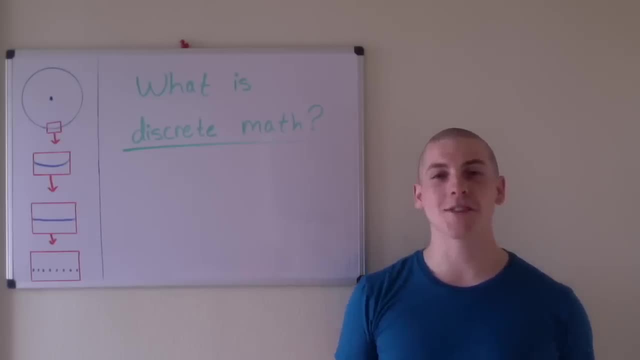 you may be thinking I never use math that involves infinite sets, but I promise that you do. The simplest example is with a circle. A circle, by definition, is an infinite number of points equidistant from a fixed point, And the problem with this is that if we have 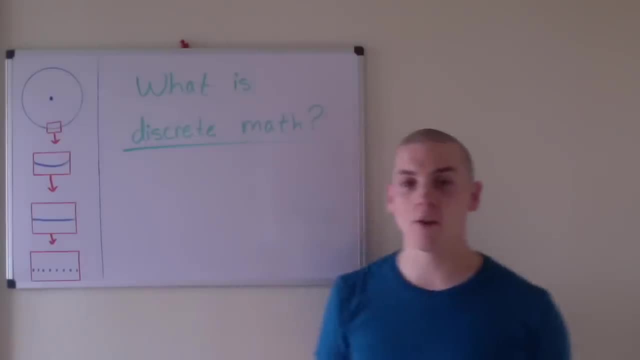 a circle on a computer and we try to write a program that prints out all of these points, it will run forever because there are an infinite number of points and therefore an infinite number of executions. So this is physically impossible. That's why, if we zoom in here, 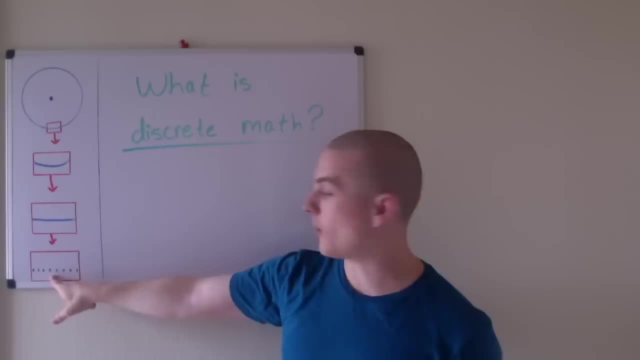 you can see that when you come down to here, there are all these points, but in reality we should have even more points between these points And then, if we zoom in on those, we'll have more points between those points and we can never complete the task. Now we've. 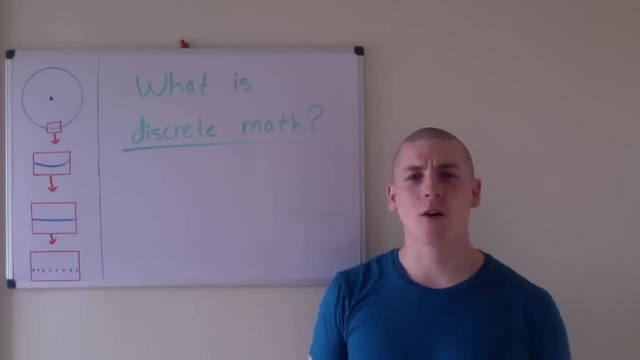 all seen circles on computers. So what's going on? How is this possible? We just established that it's impossible. Well, the answer is that they're approximations. For example, consider regular polygons. Regular polygons like a triangle or a square or a pentagon- those don't really look like circles. 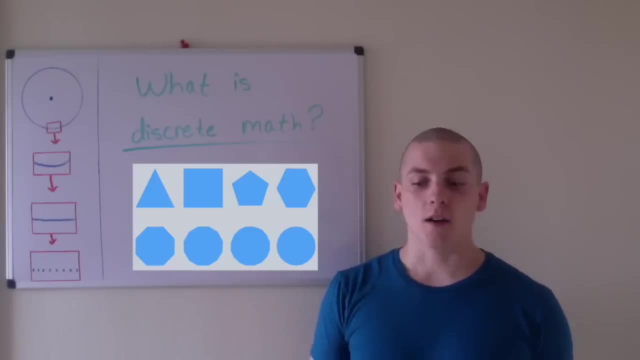 But if you keep increasing the number of vertices, eventually you'll start getting hexagons, octagons, dodecagons, hexadecagons, icosagons and so on. So if you keep increasing the number, 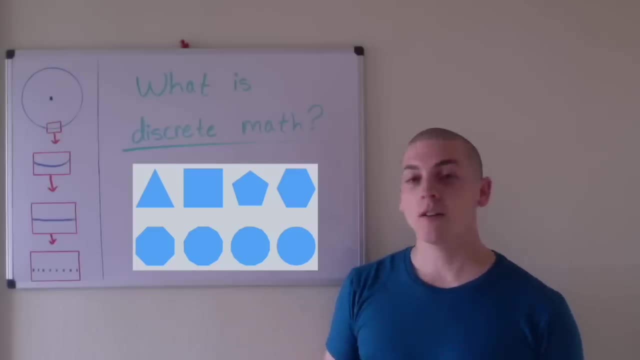 of vertices. eventually you'll start getting hexagons, octagons, dodecagons, hexadecagons and so on. You can see that, these regular polygons, the more and more you keep increasing the number of vertices, which the vertices are equidistant from a fixed point, they will. 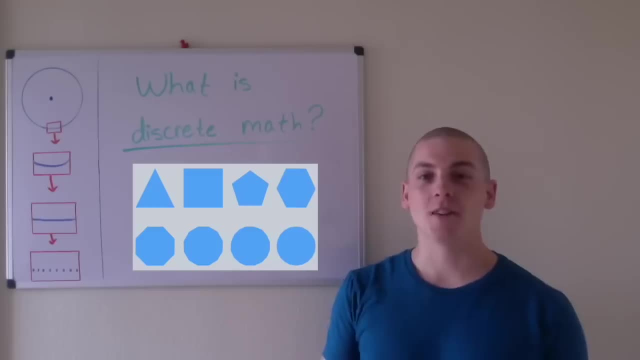 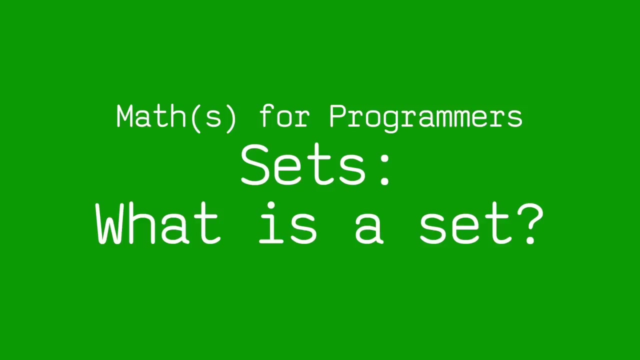 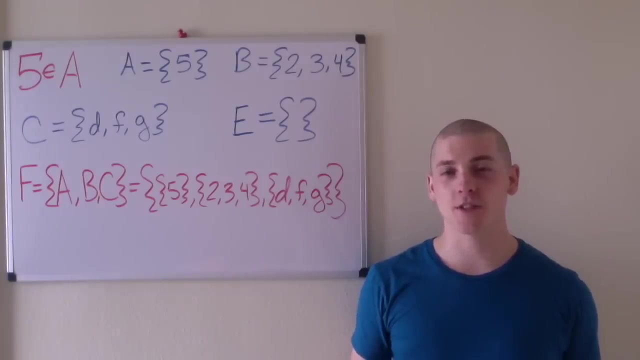 eventually approximate a circle. Eventually they will be indistinguishable to the naked eye and will look identical to a circle. In this video, I'll be explaining what sets are. A set is a collection of distinct objects called elements or members. Subtitles by the Amaraorg community. 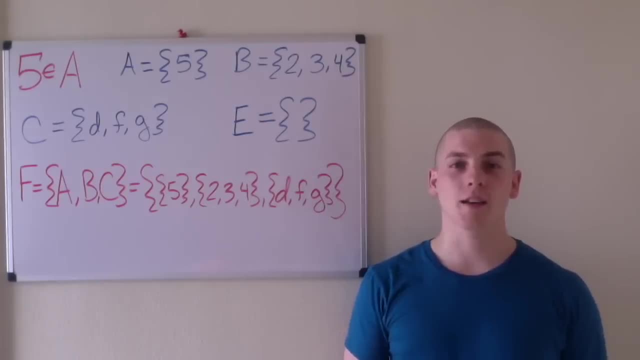 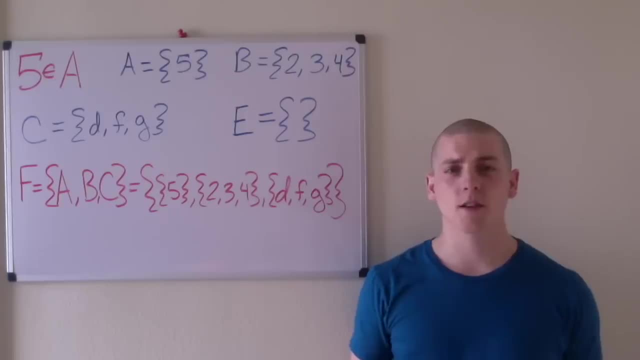 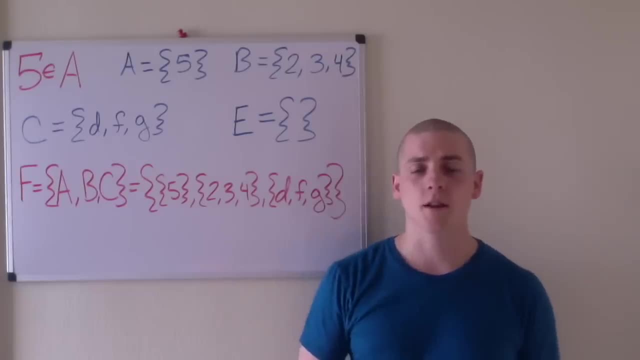 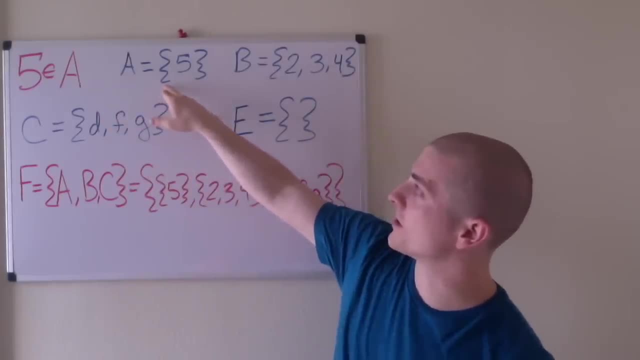 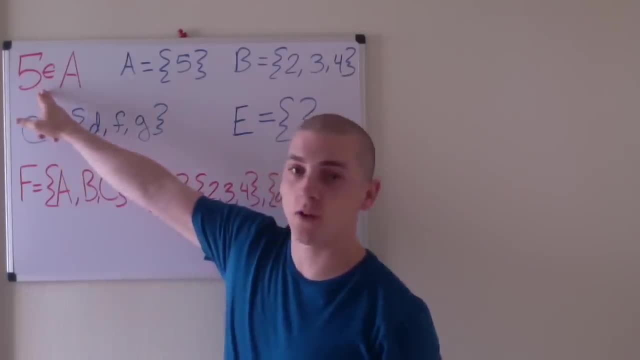 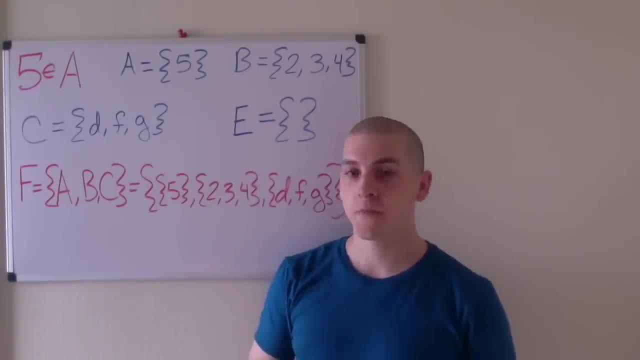 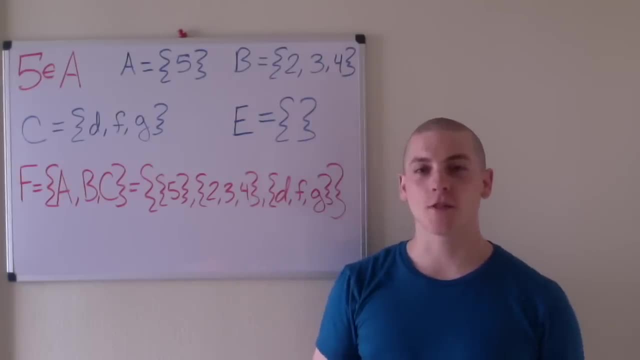 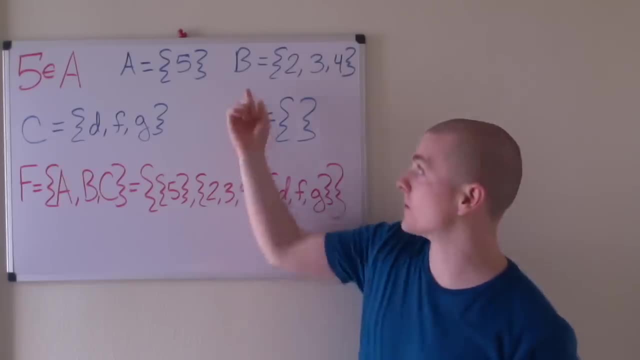 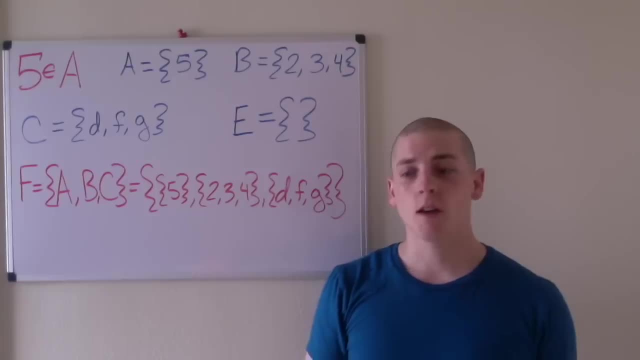 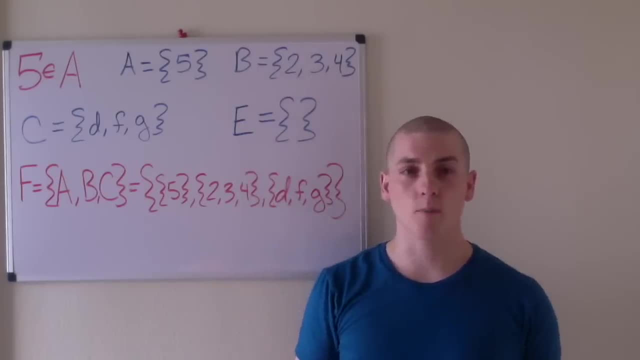 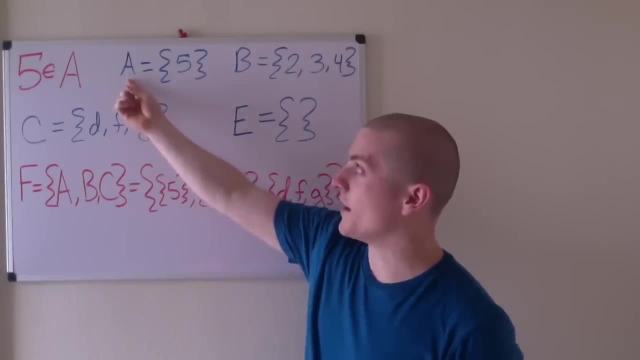 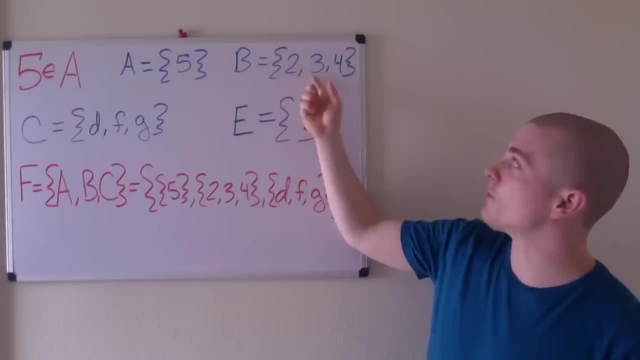 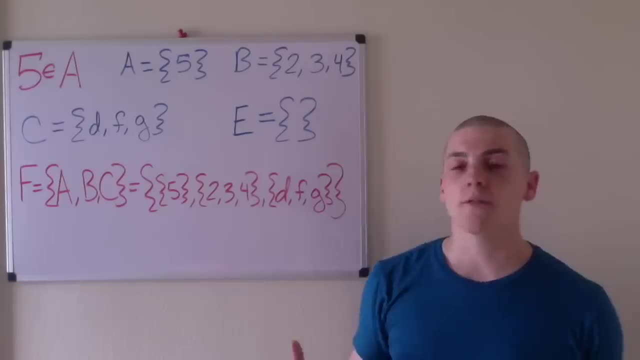 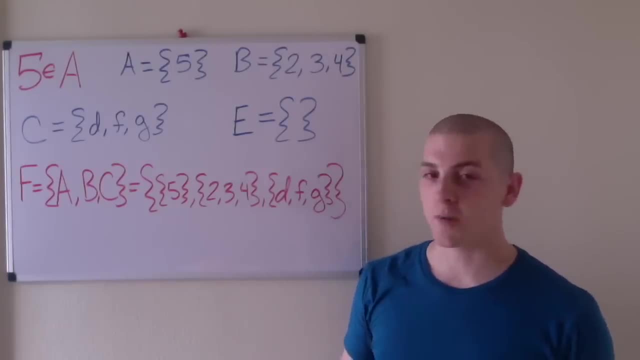 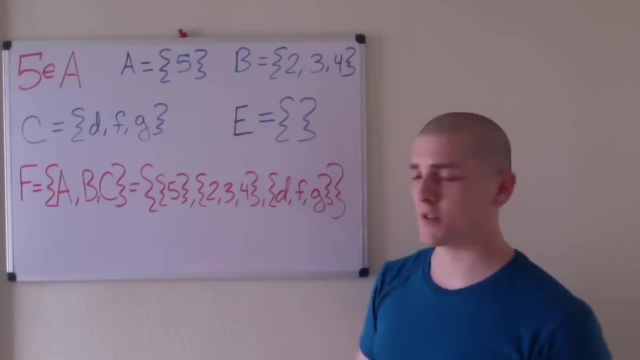 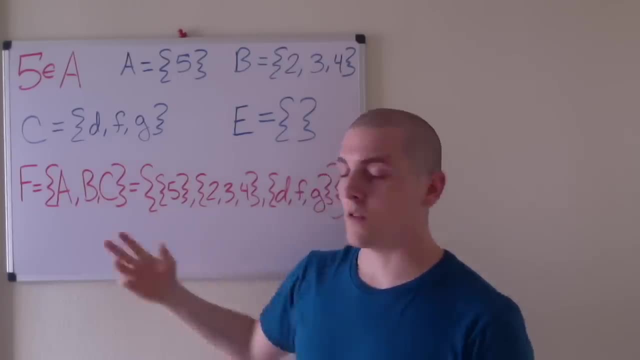 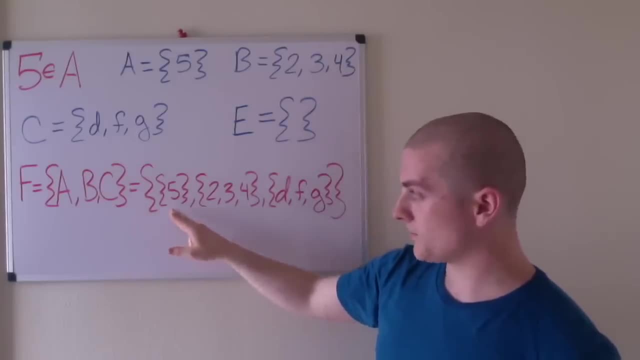 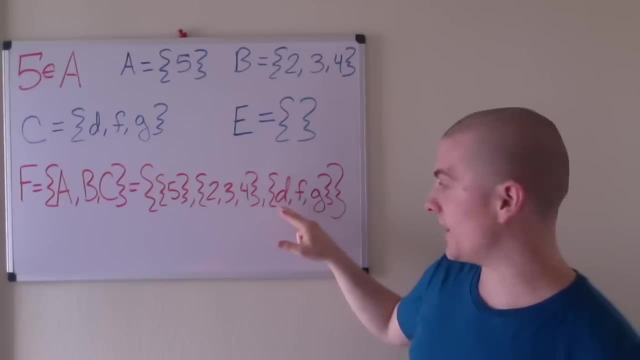 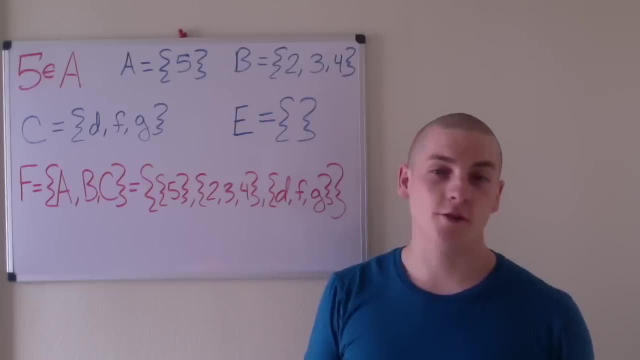 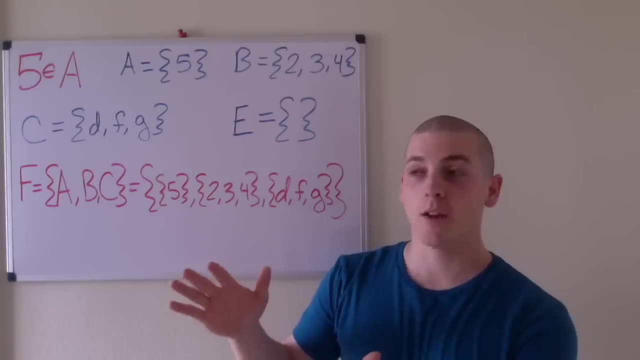 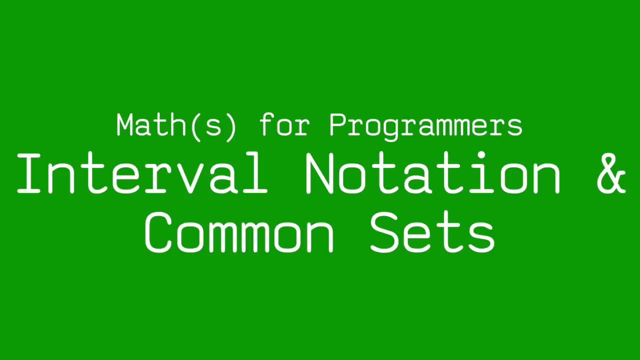 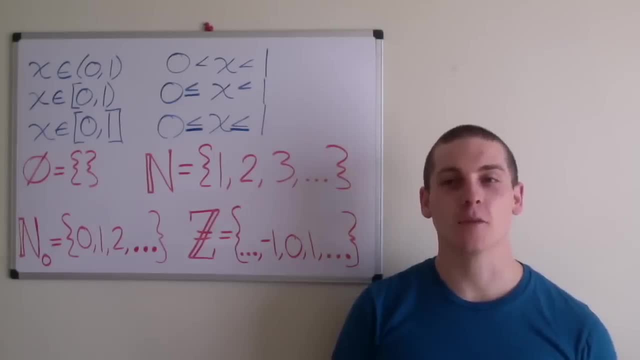 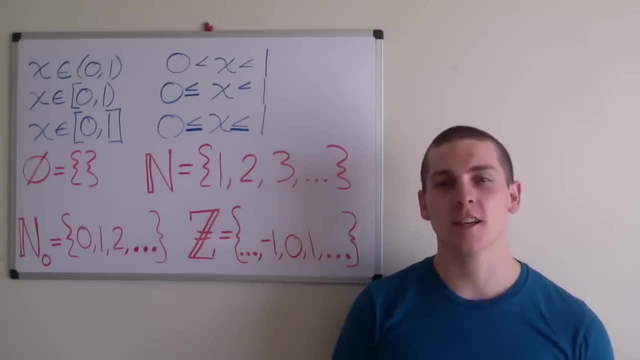 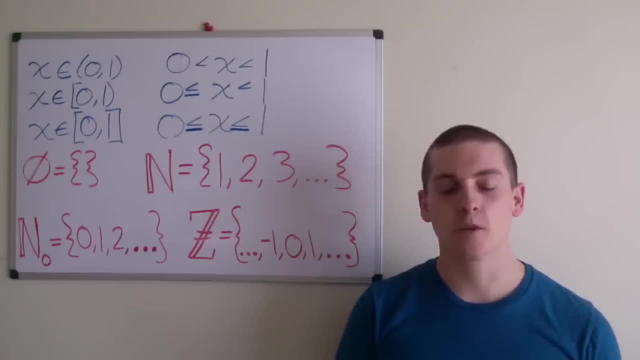 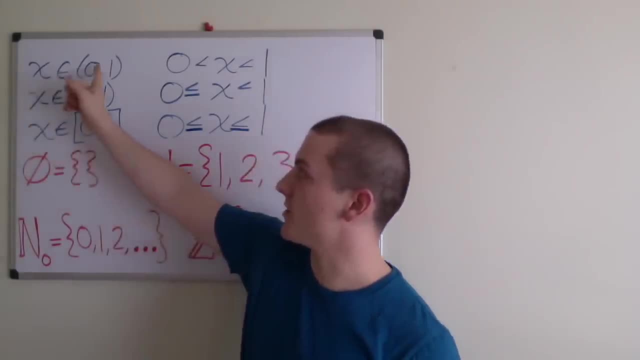 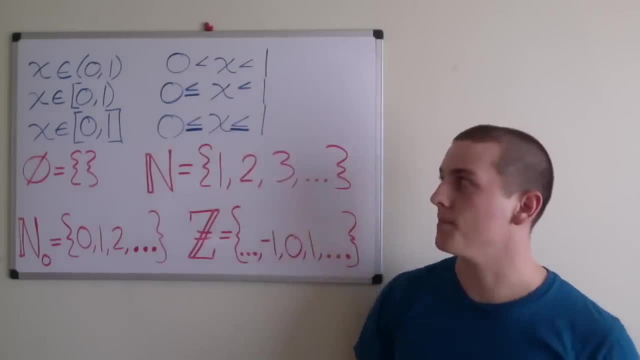 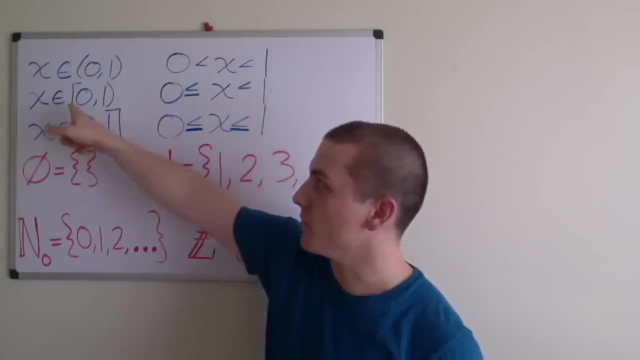 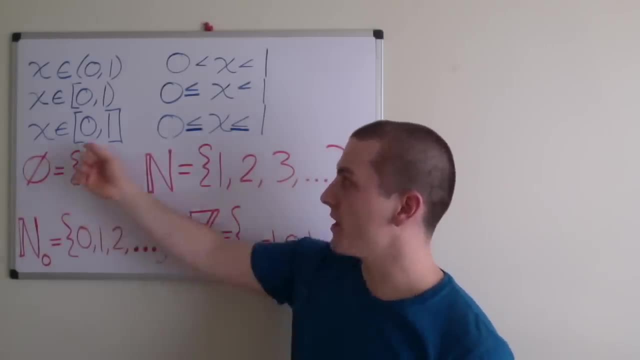 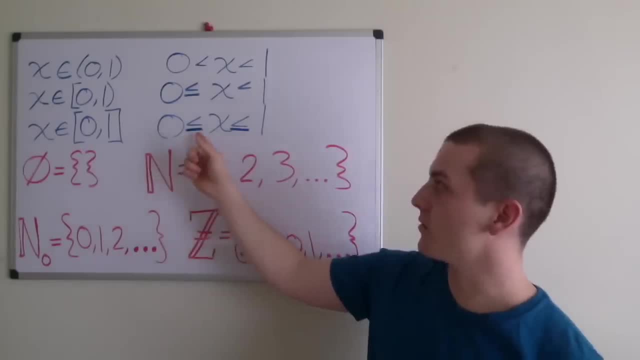 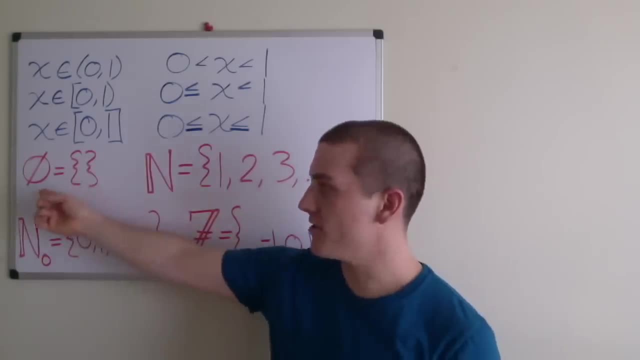 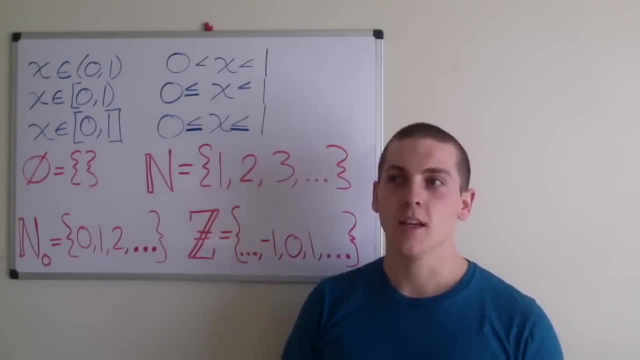 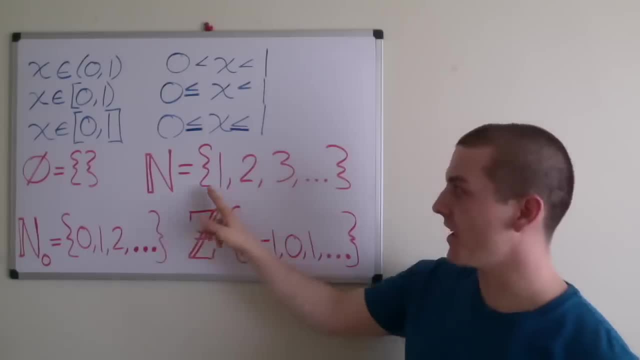 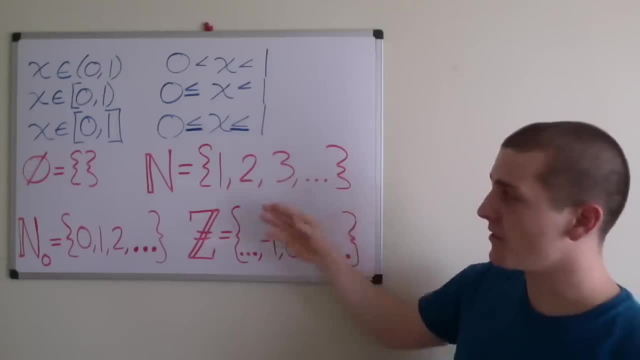 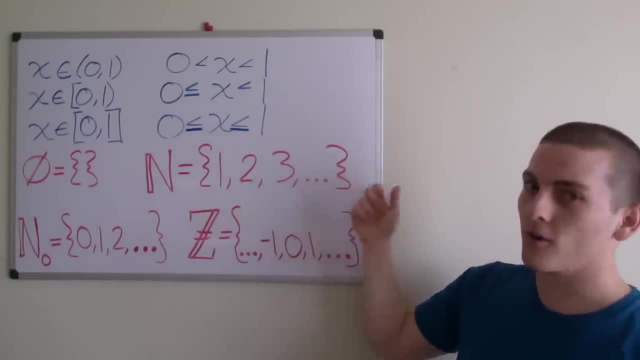 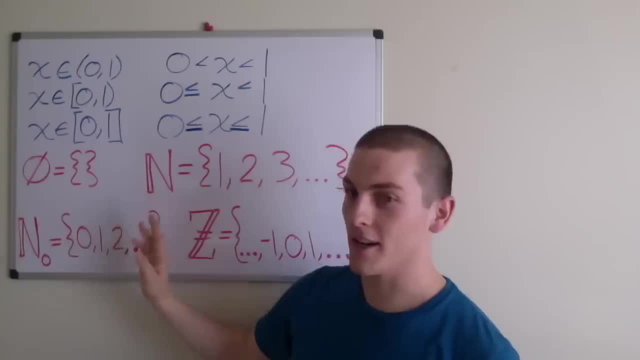 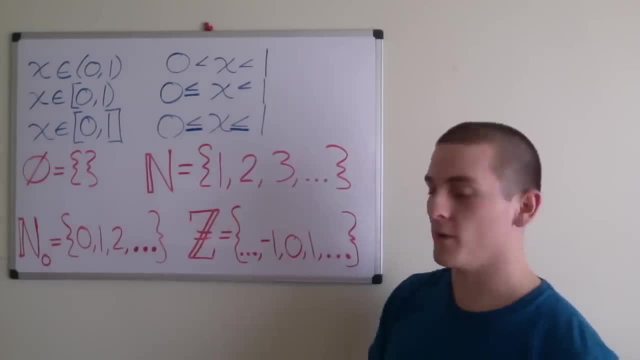 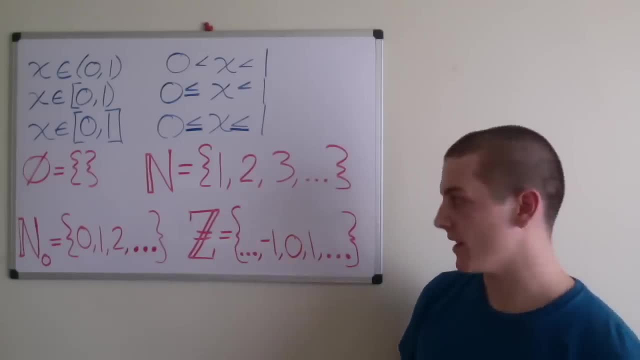 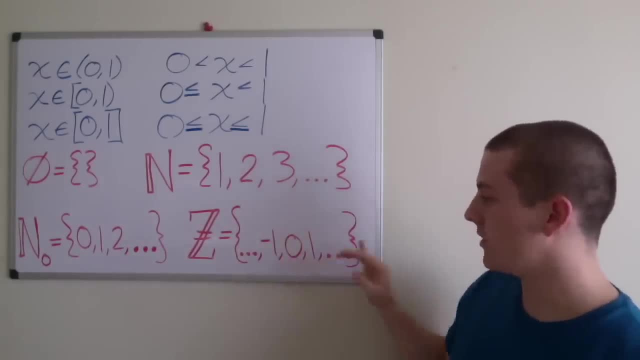 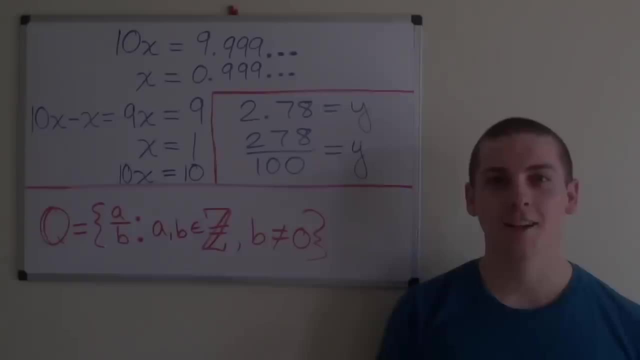 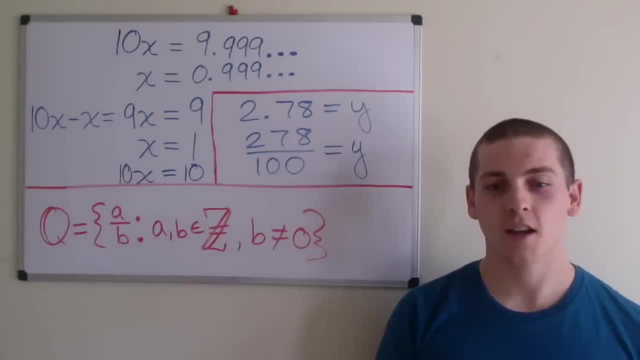 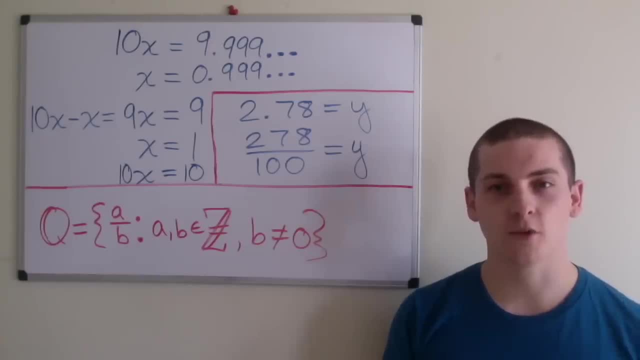 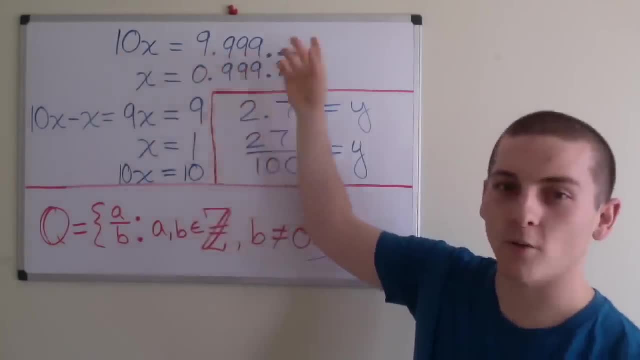 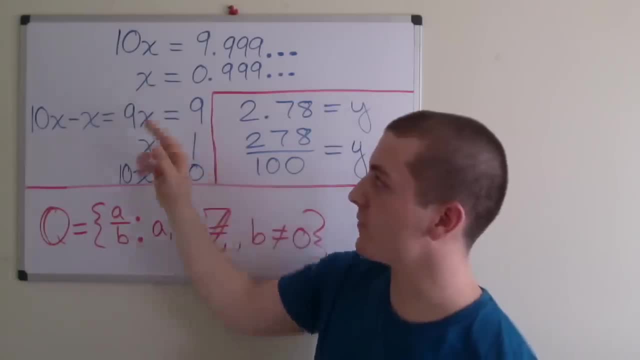 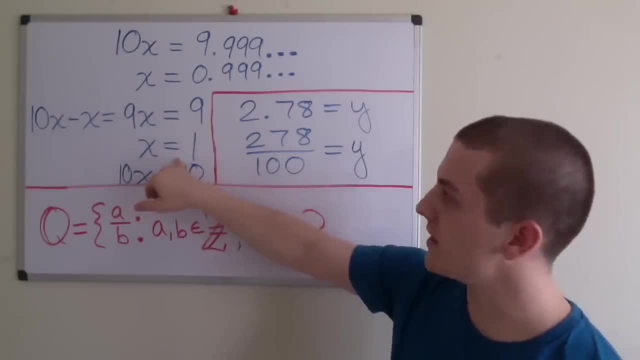 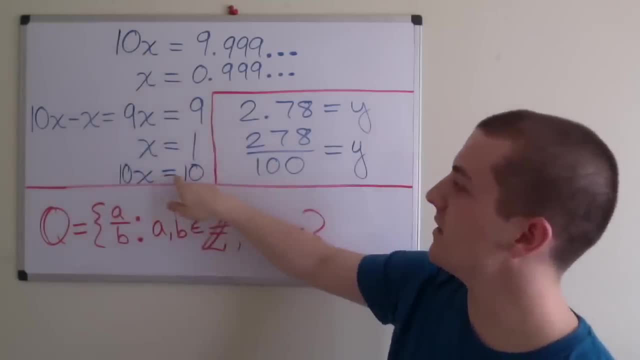 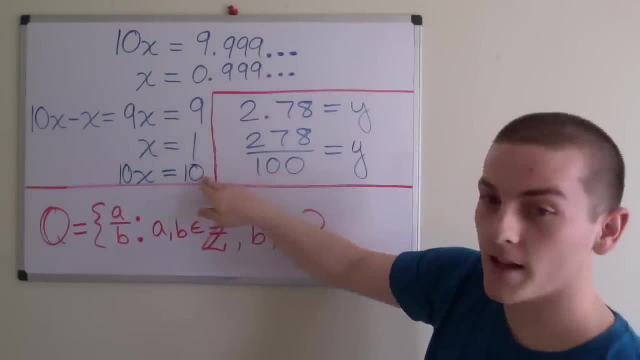 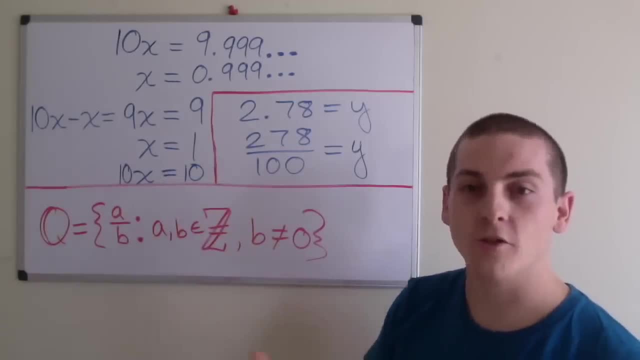 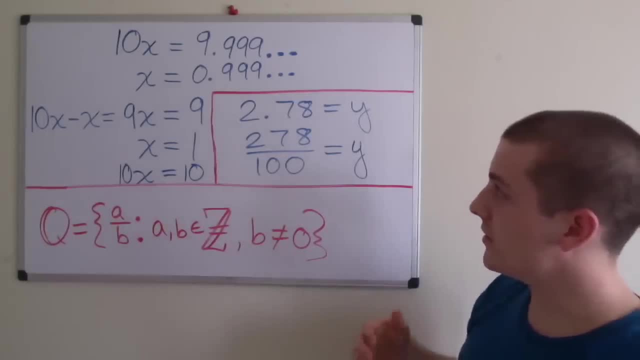 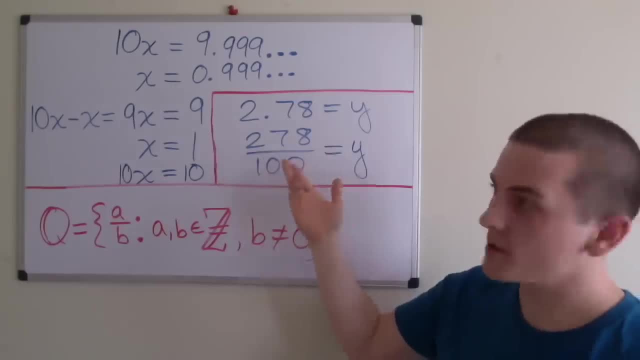 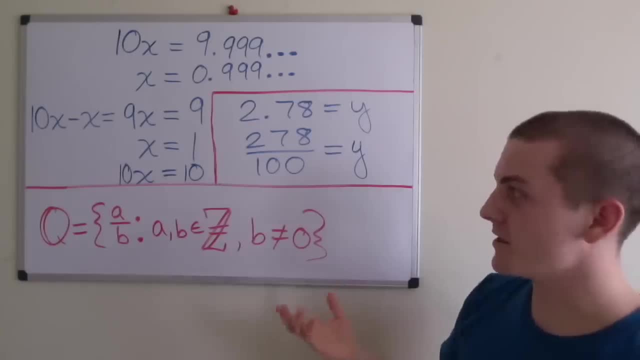 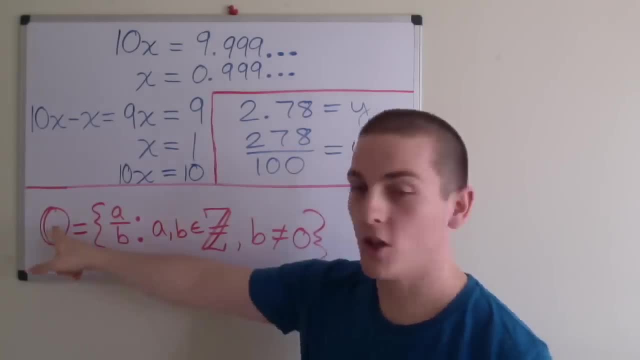 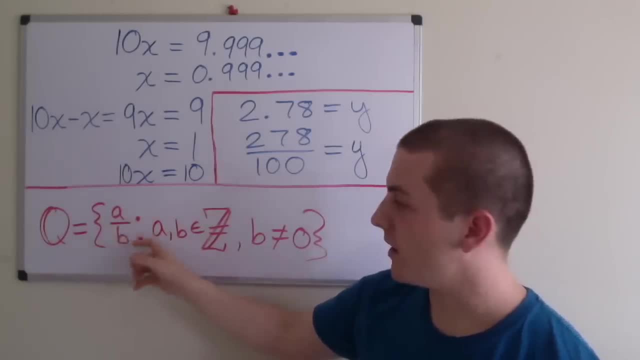 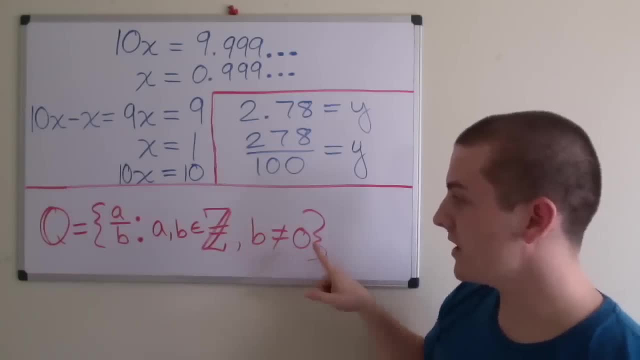 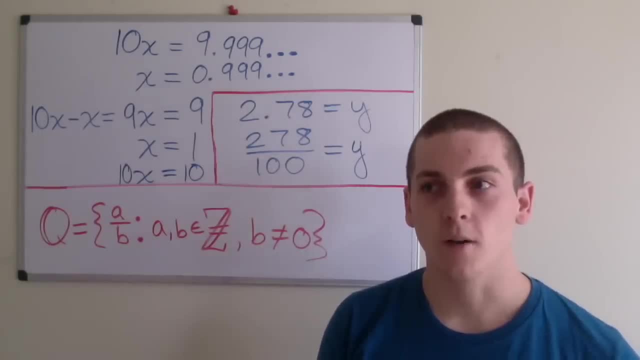 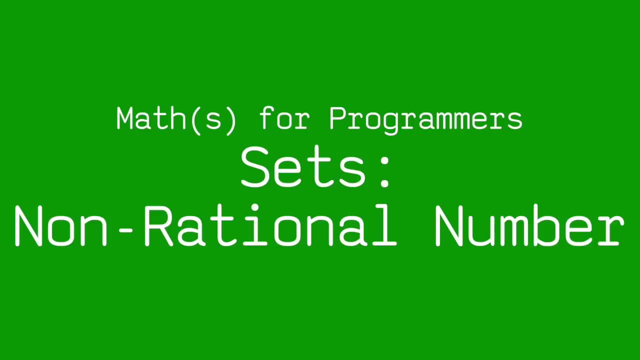 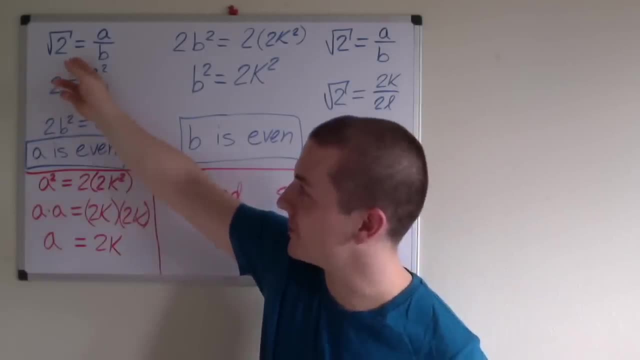 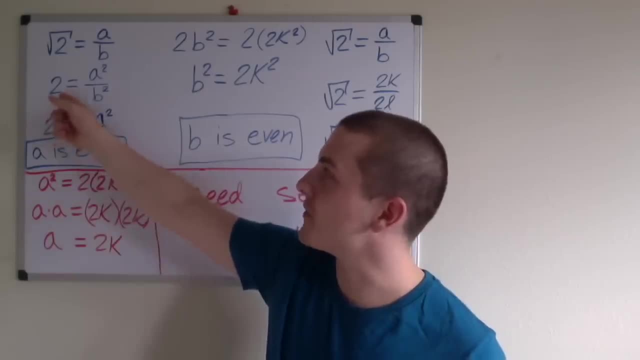 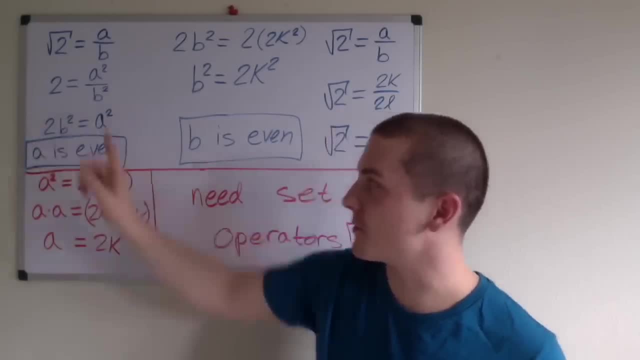 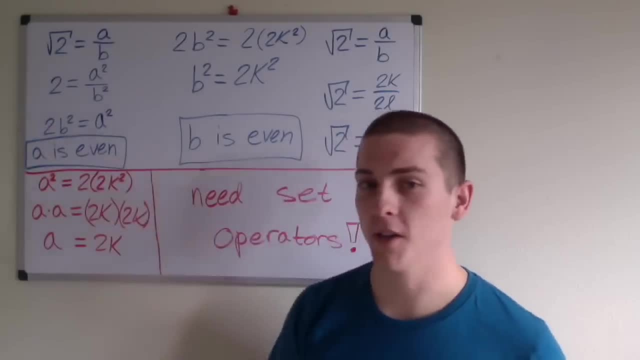 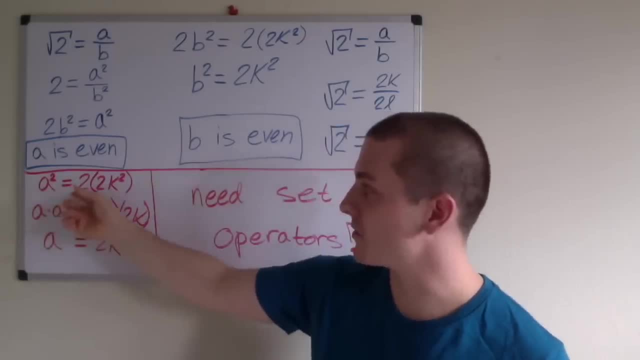 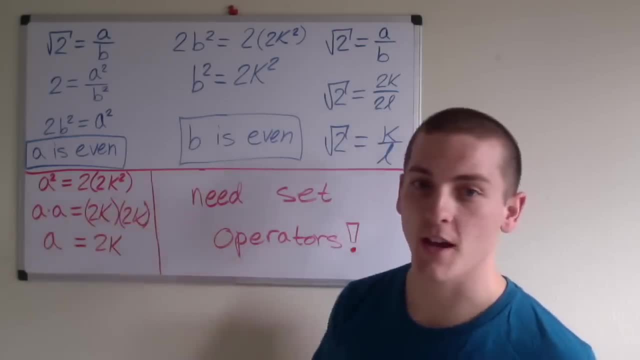 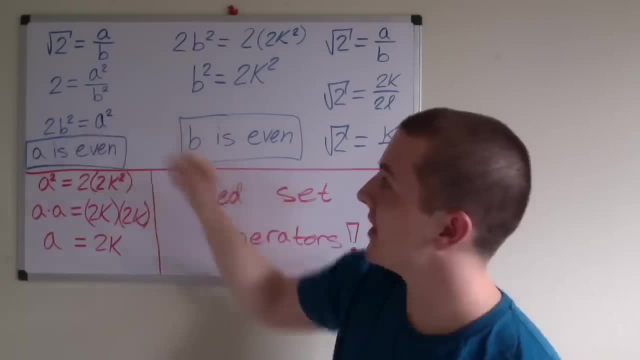 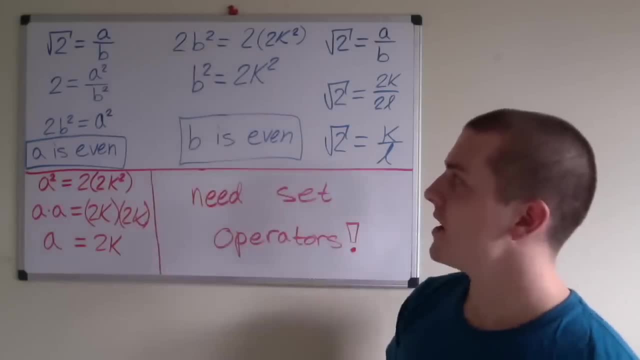 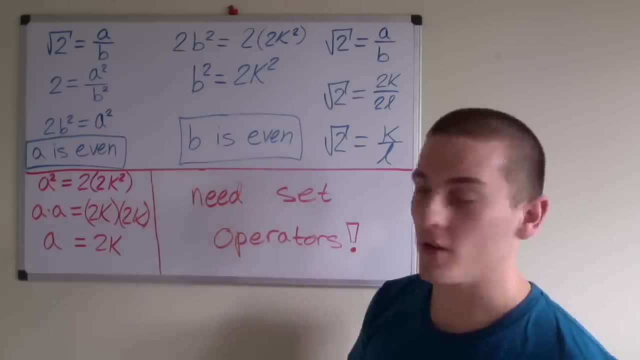 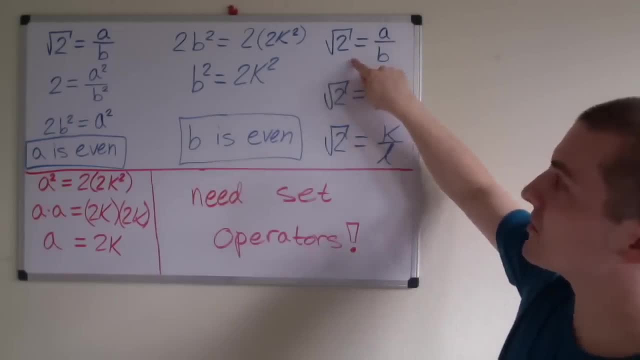 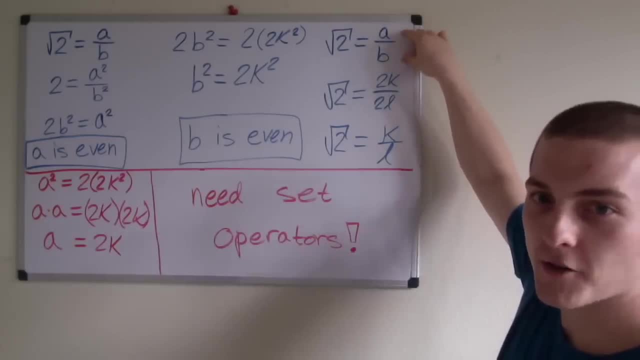 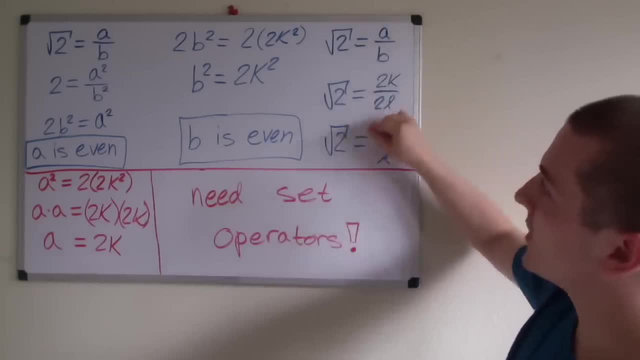 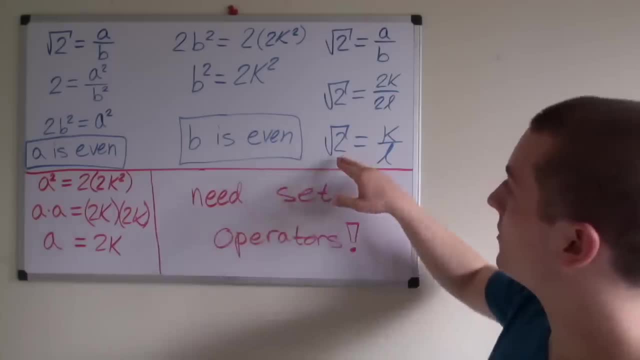 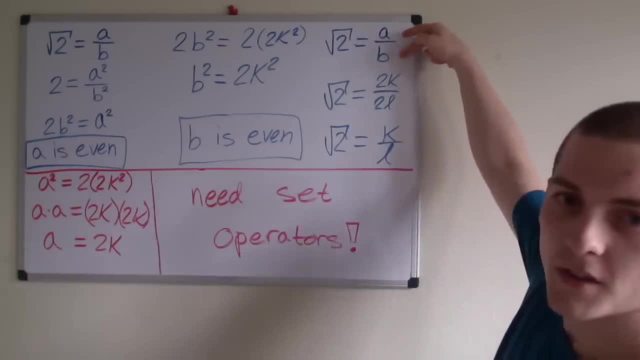 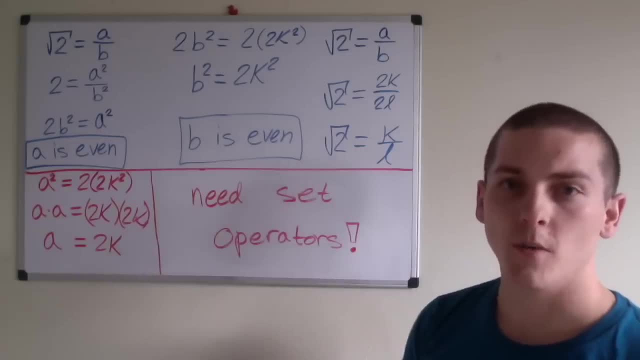 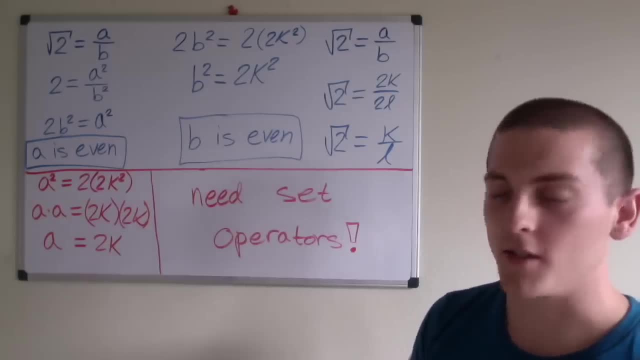 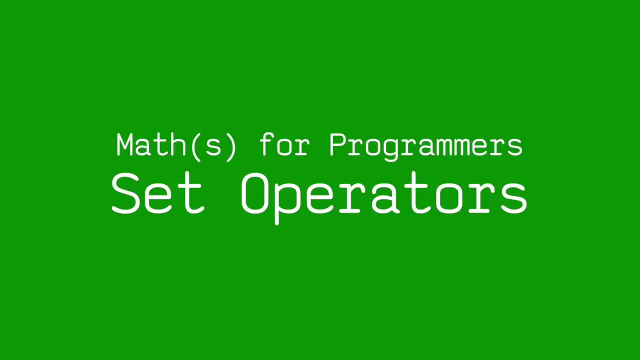 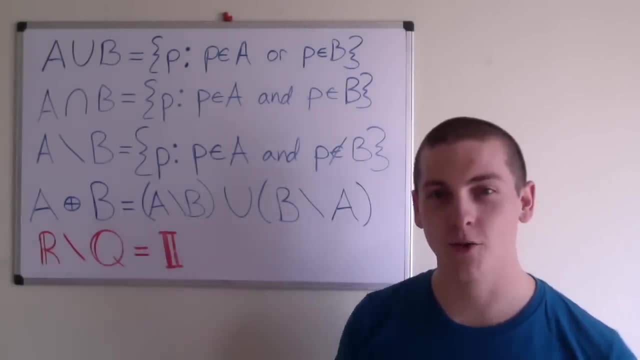 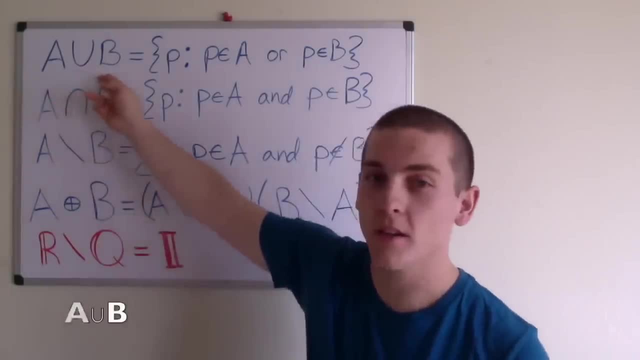 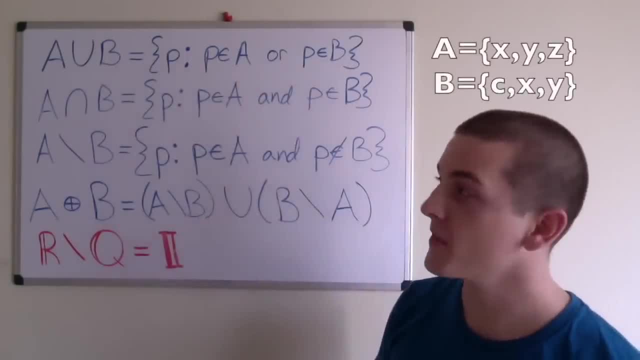 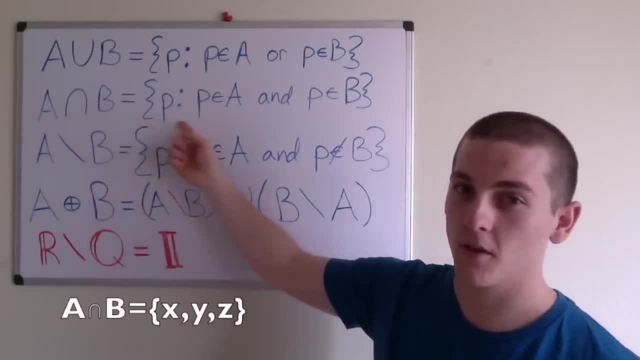 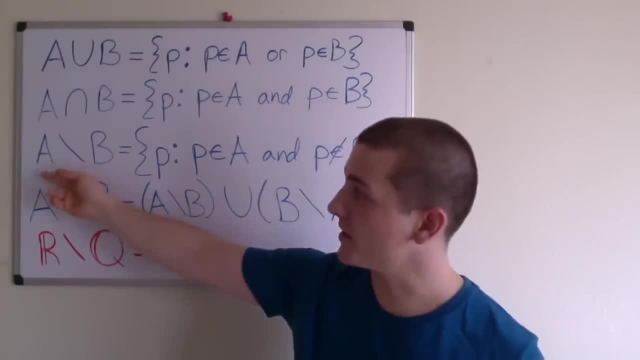 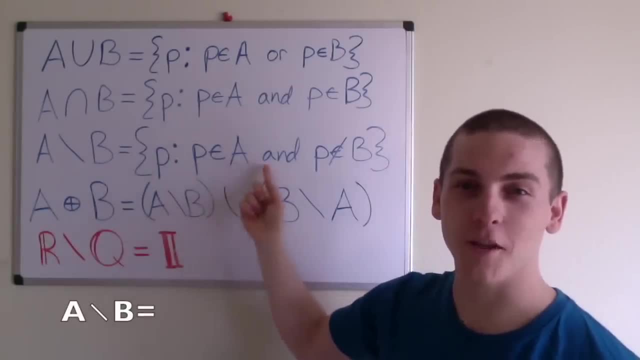 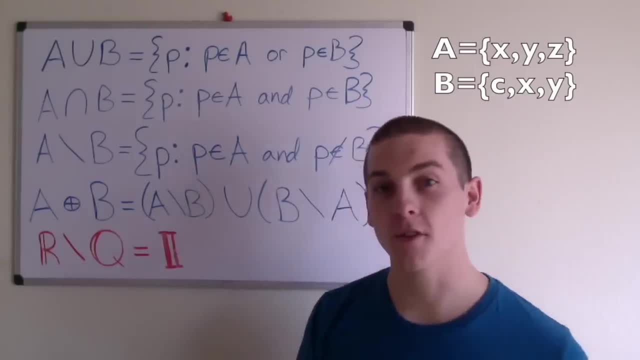 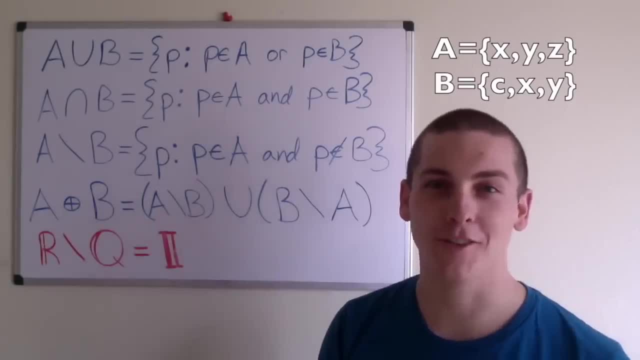 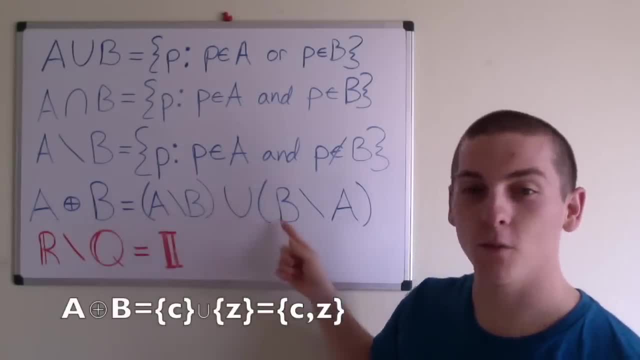 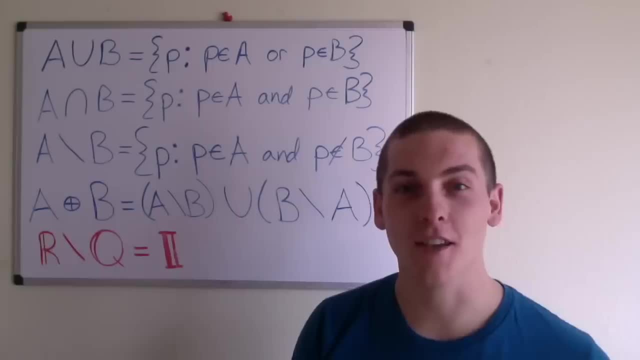 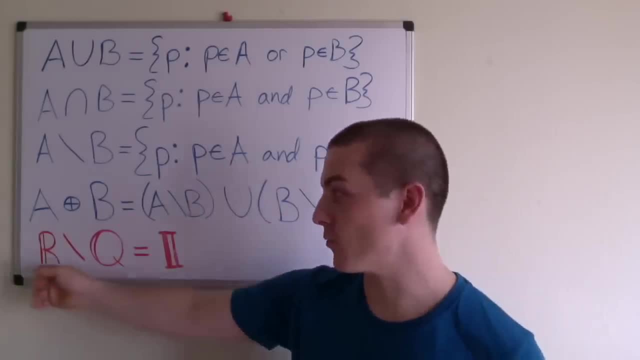 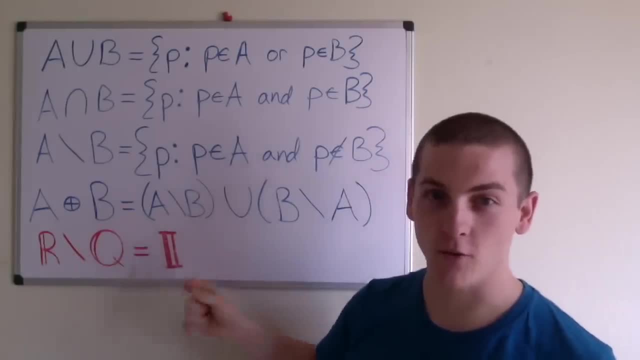 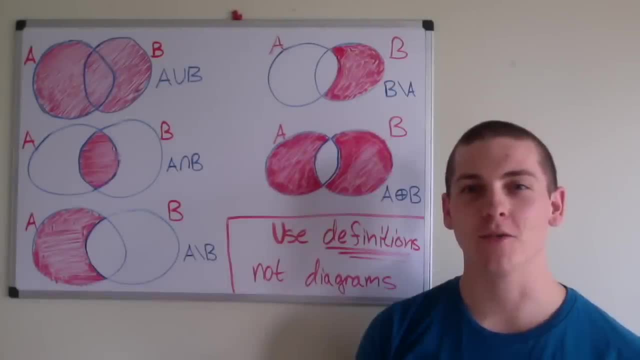 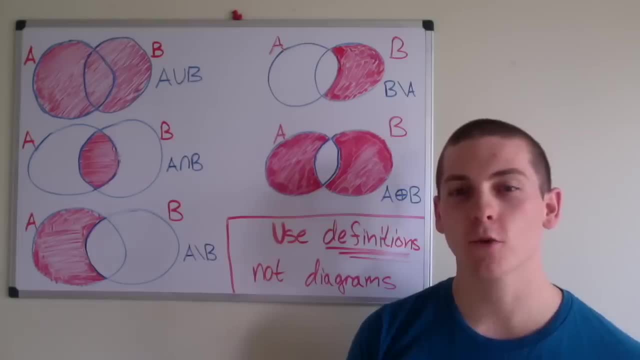 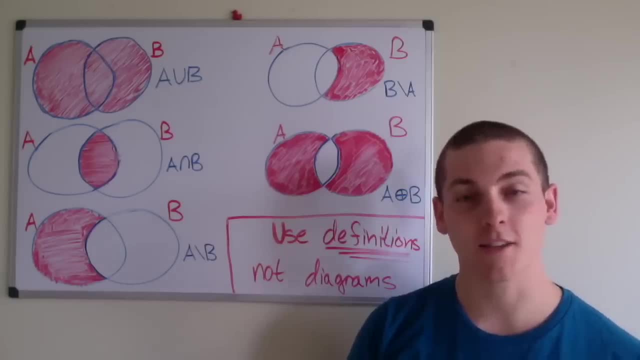 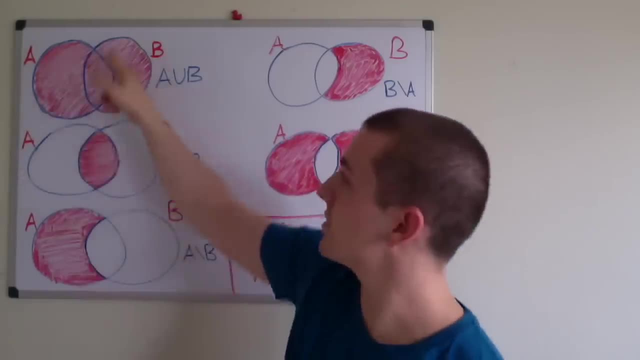 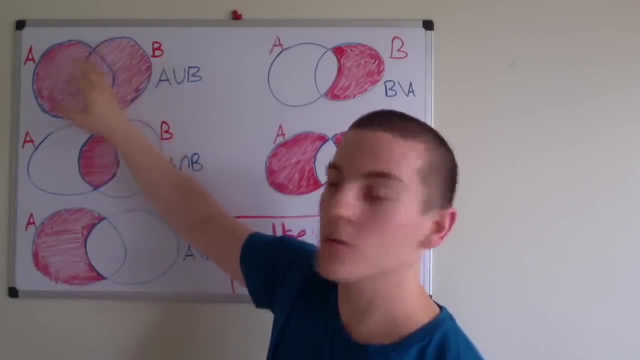 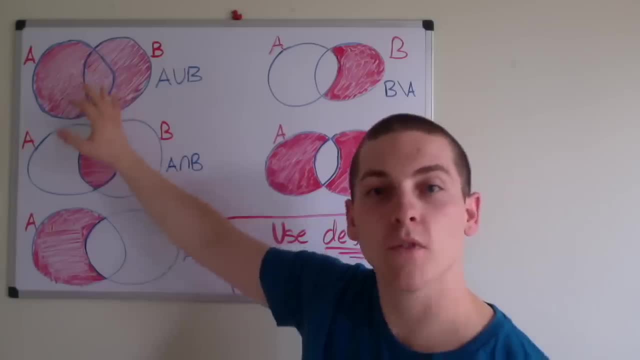 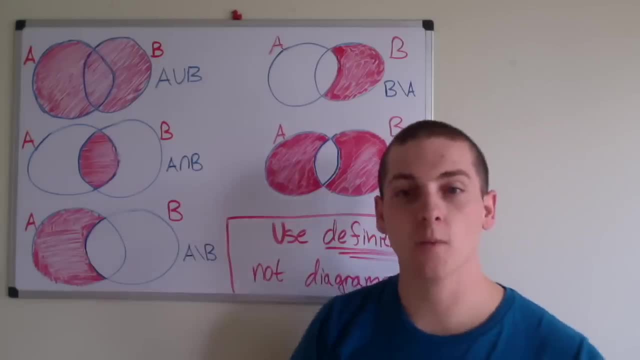 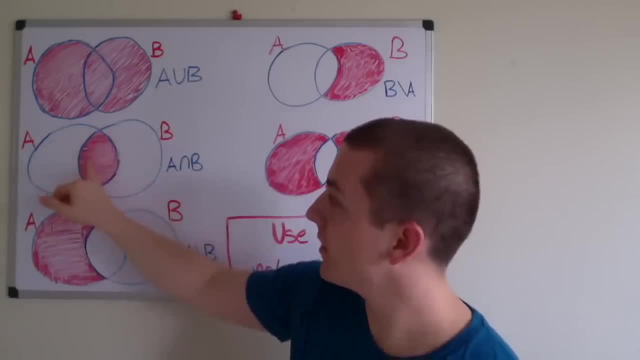 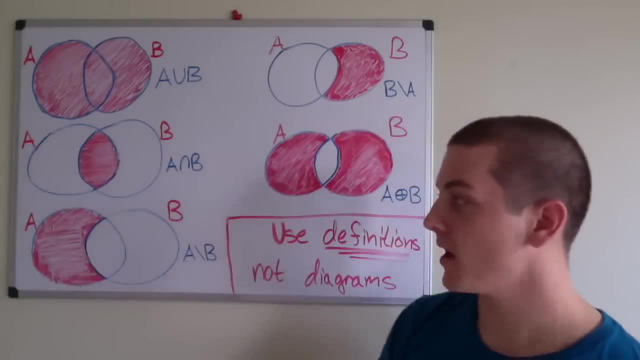 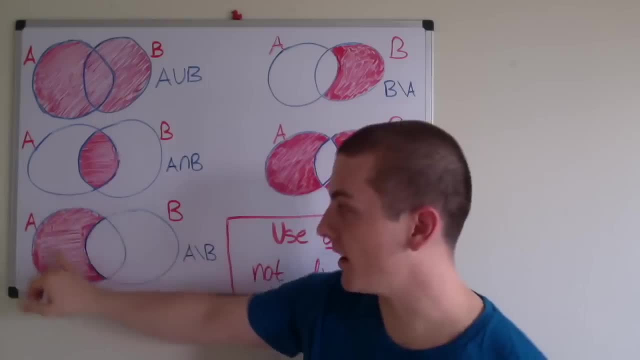 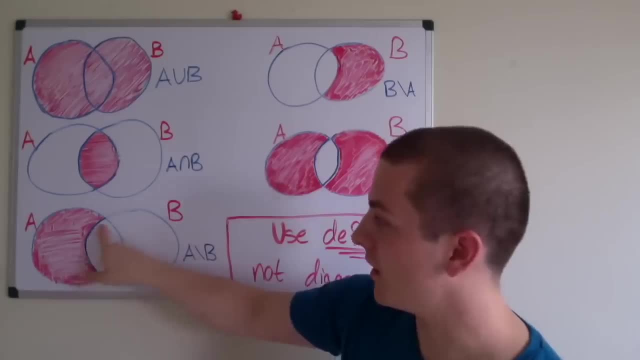 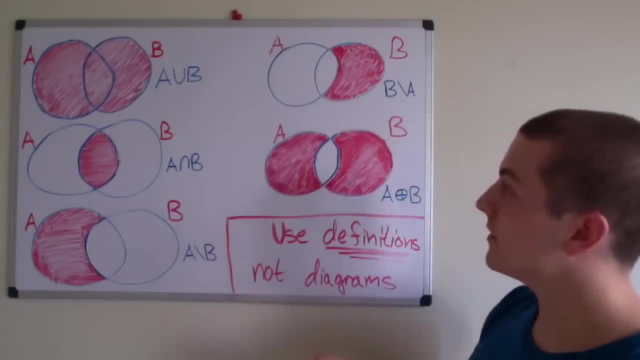 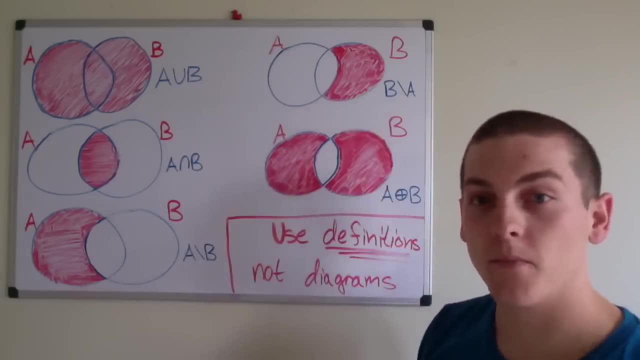 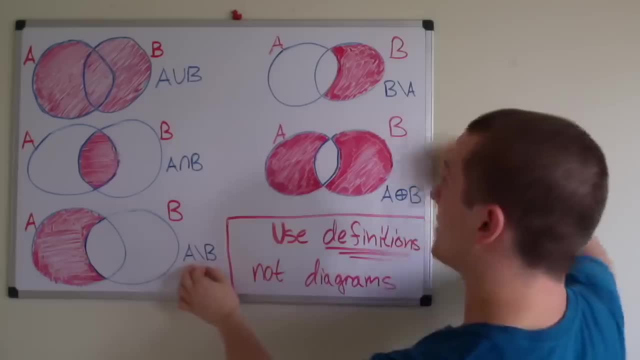 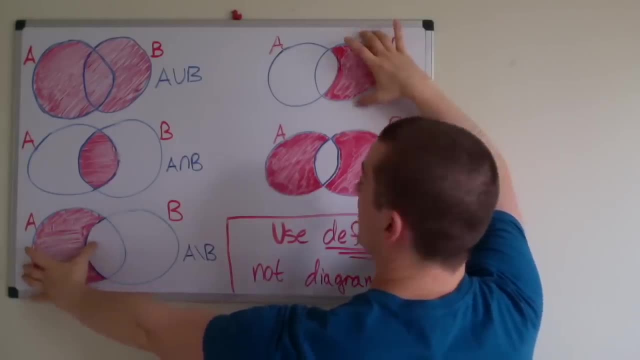 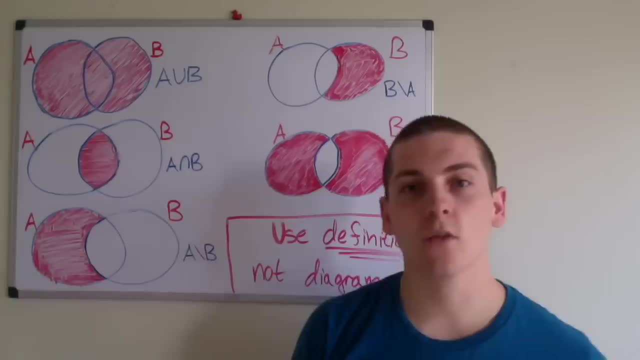 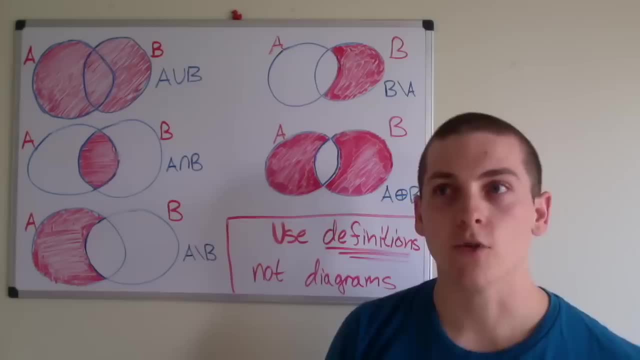 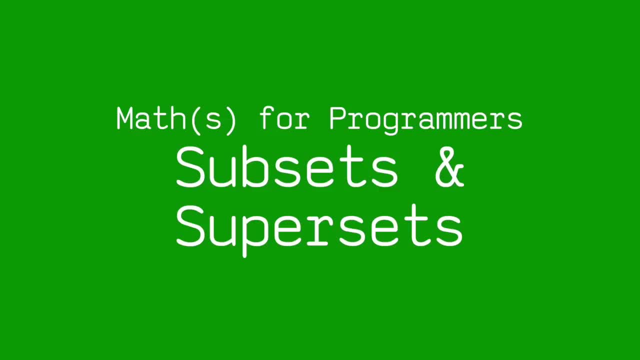 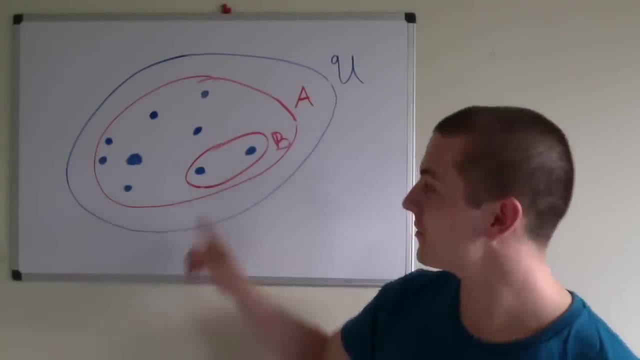 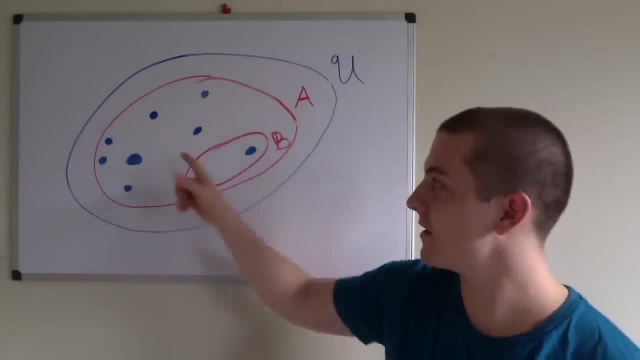 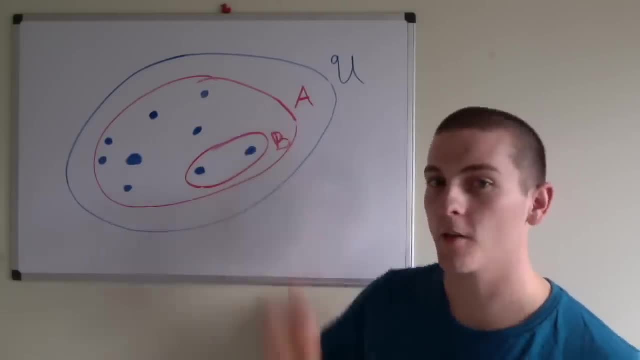 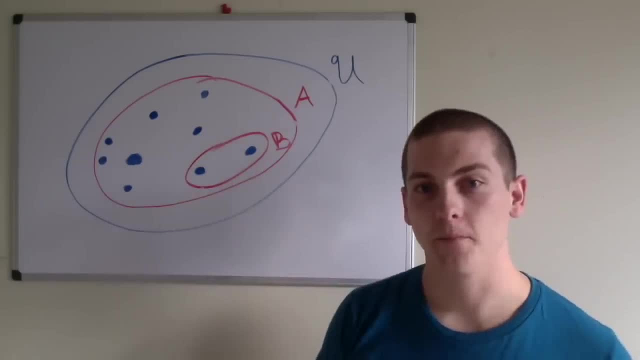 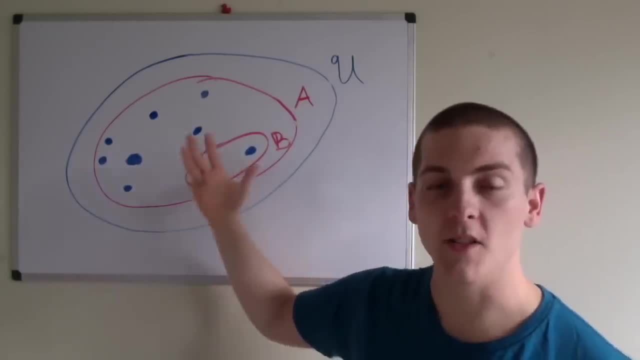 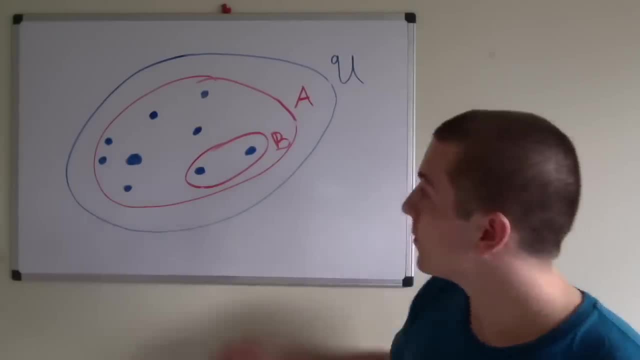 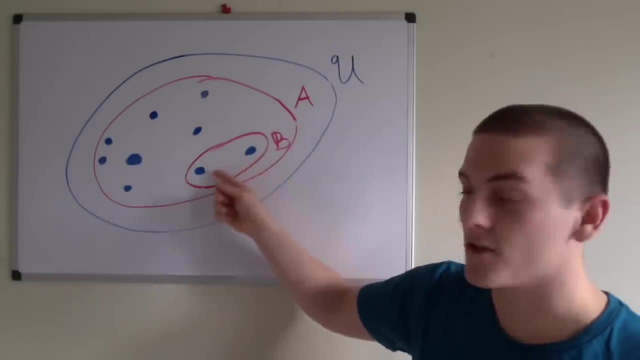 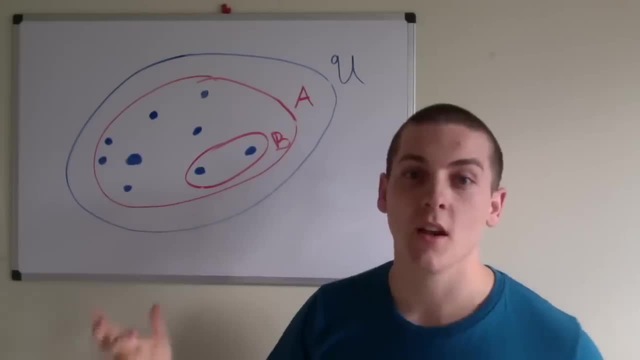 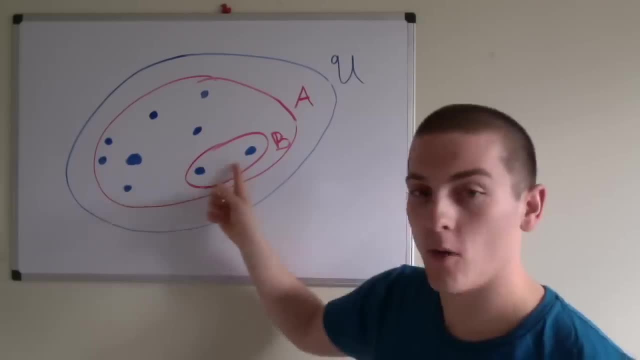 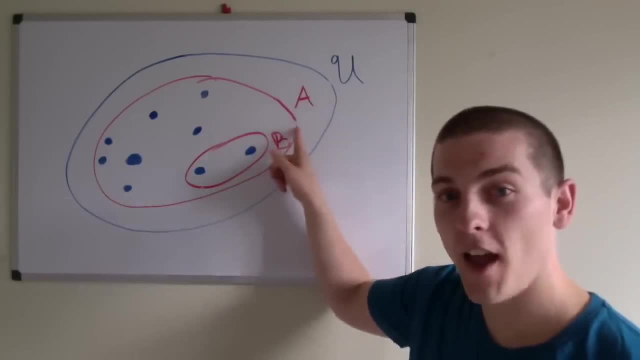 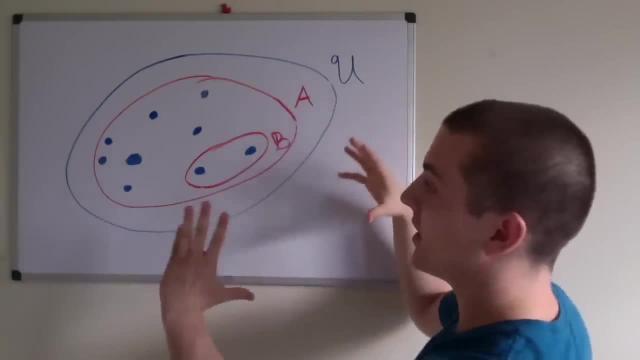 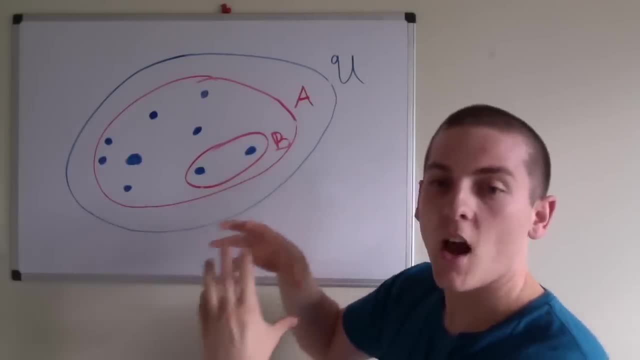 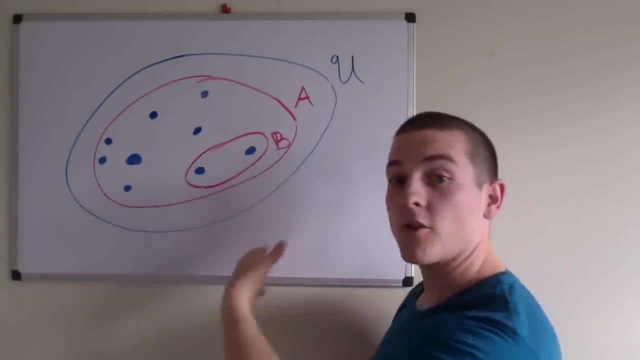 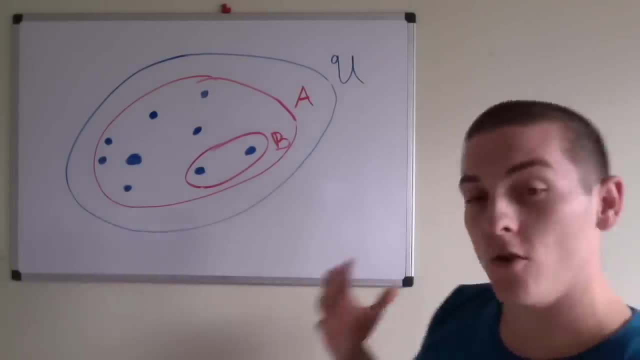 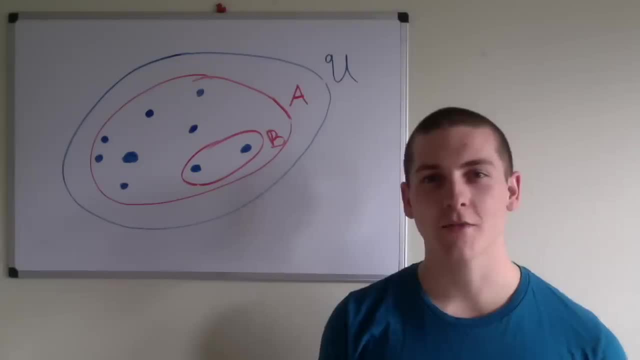 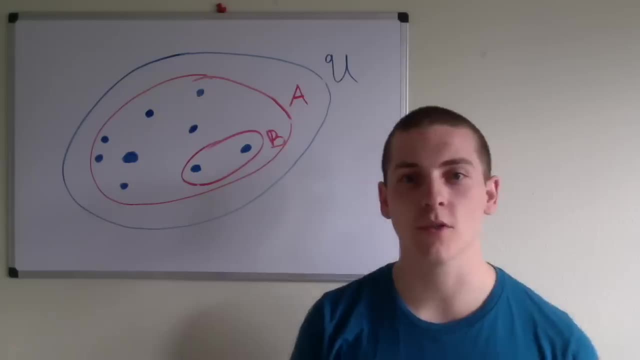 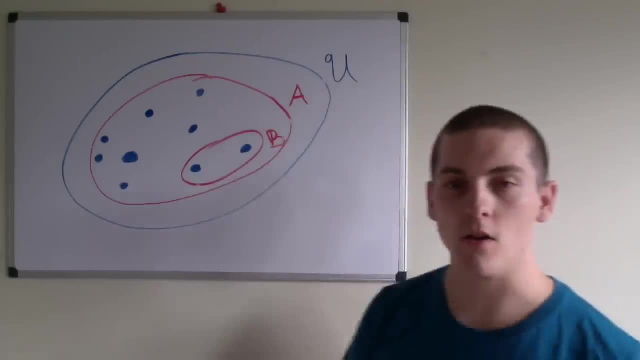 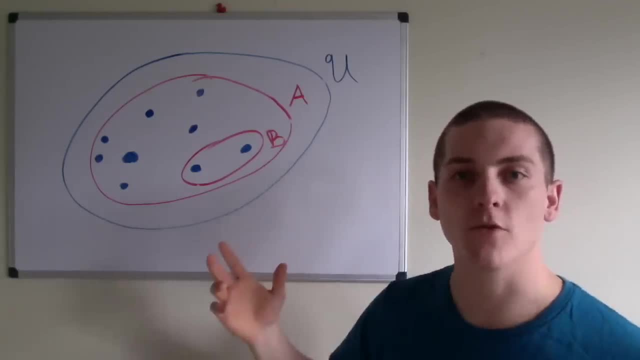 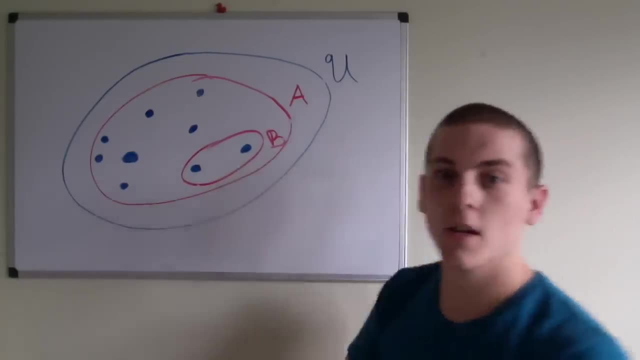 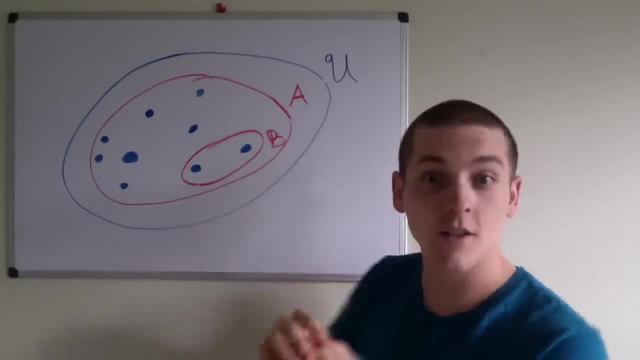 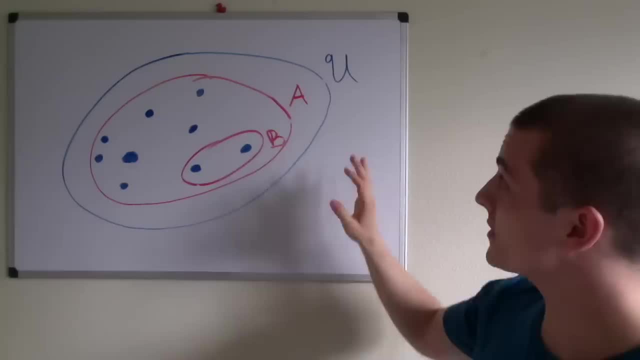 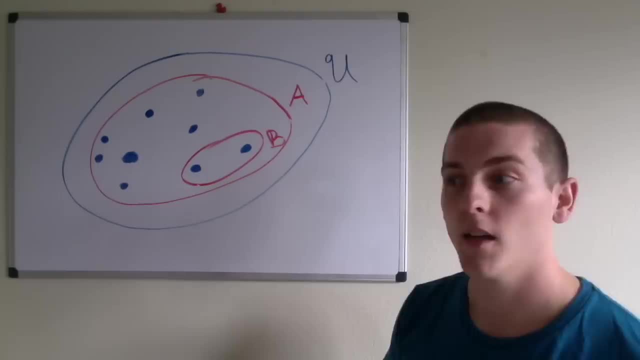 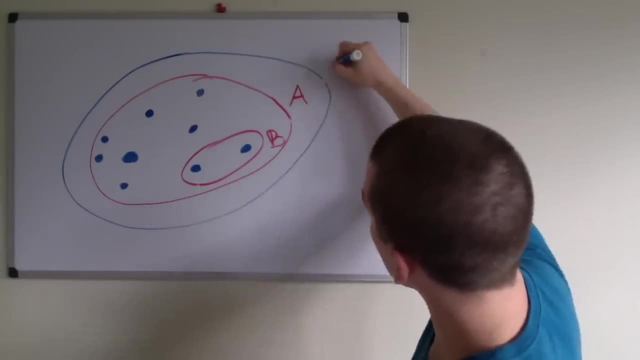 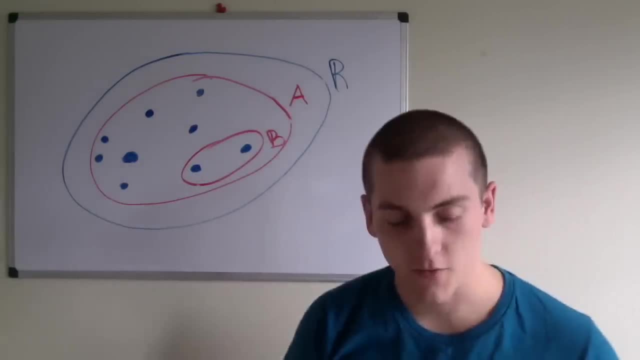 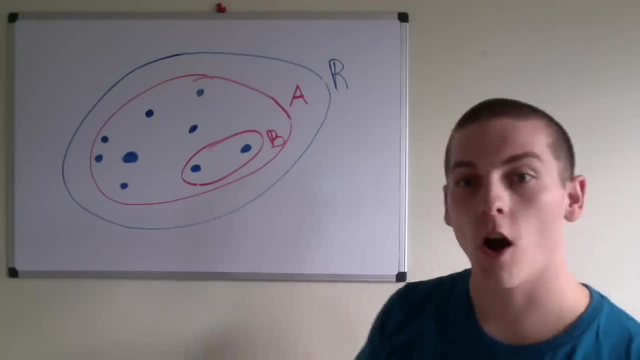 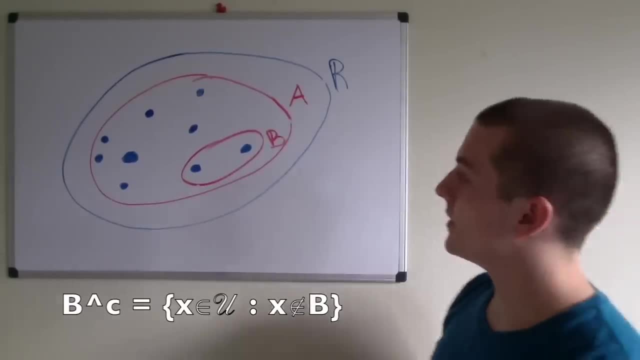 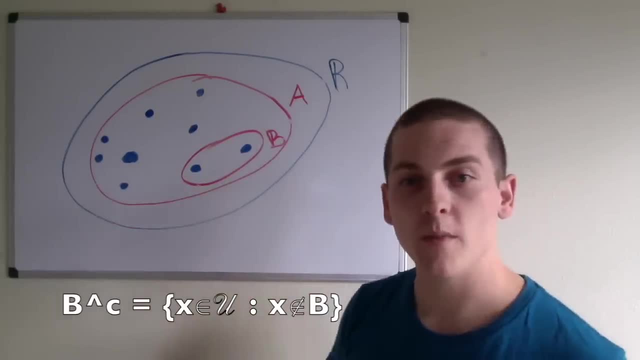 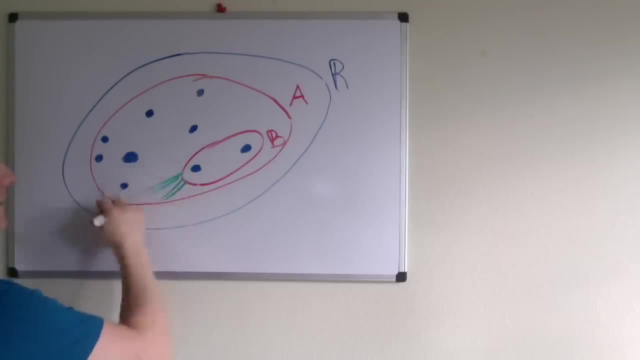 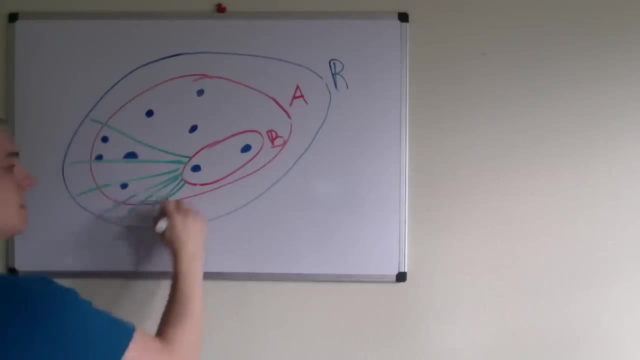 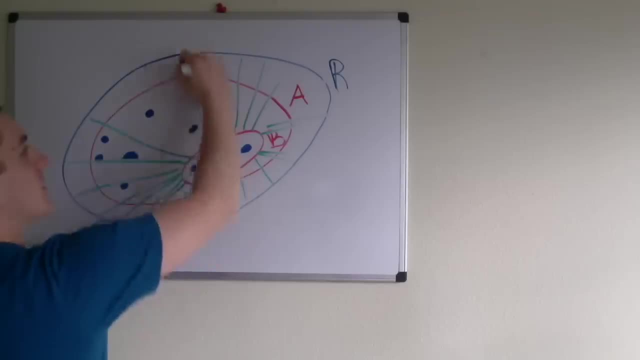 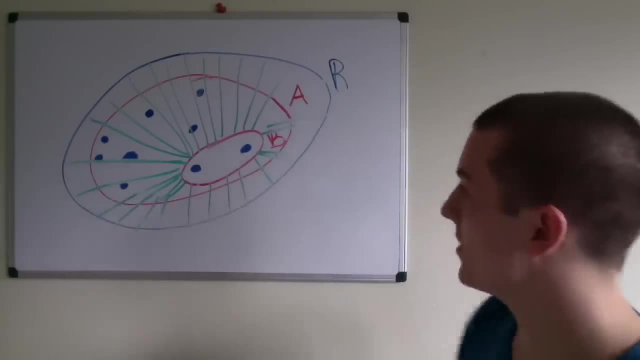 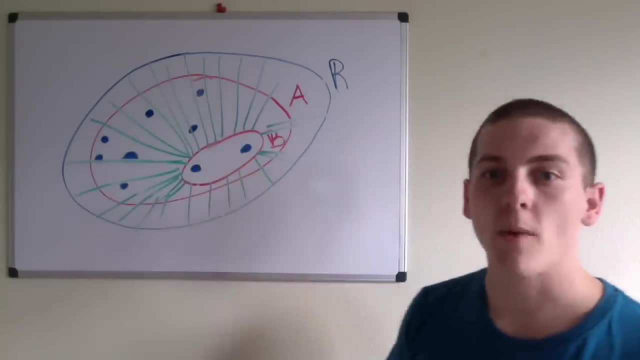 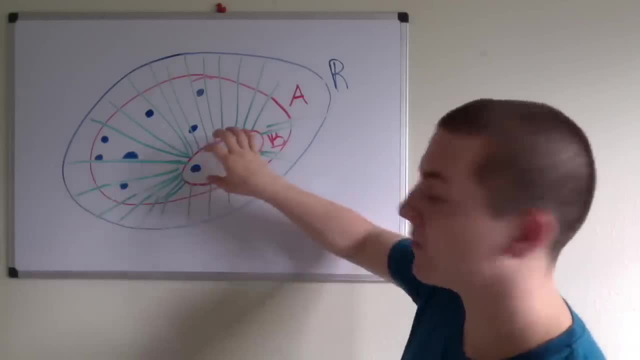 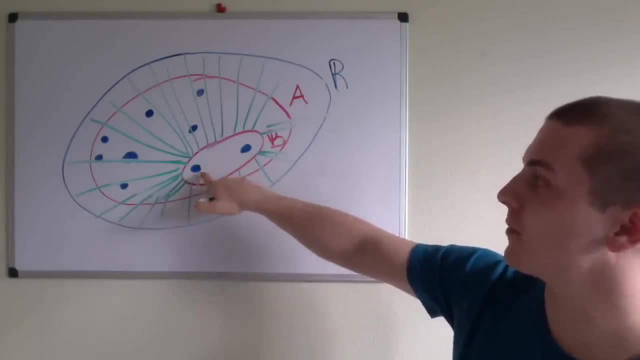 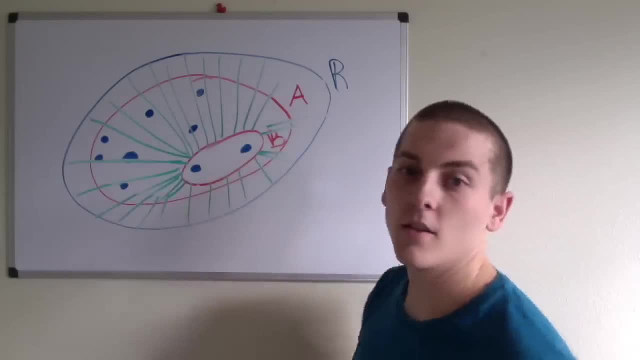 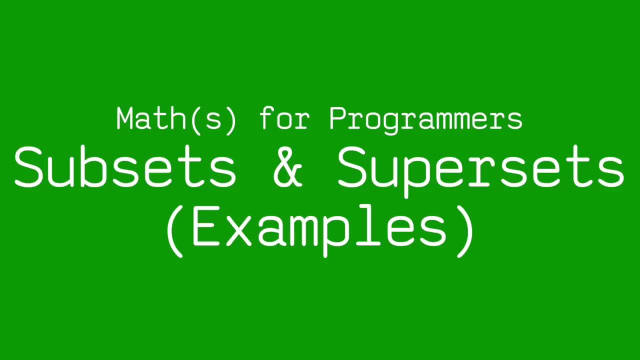 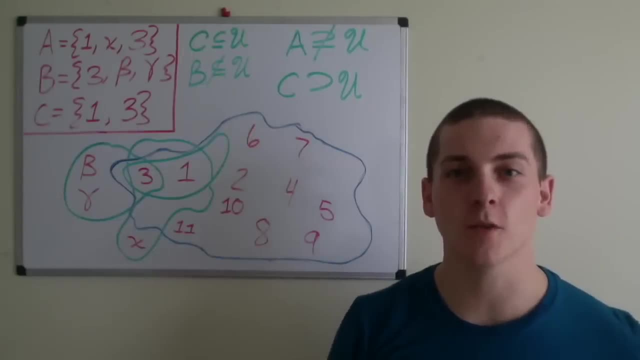 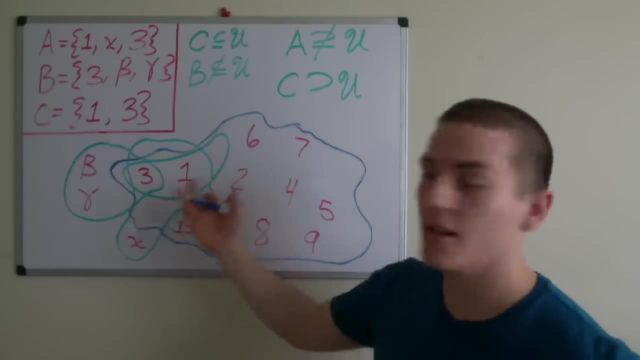 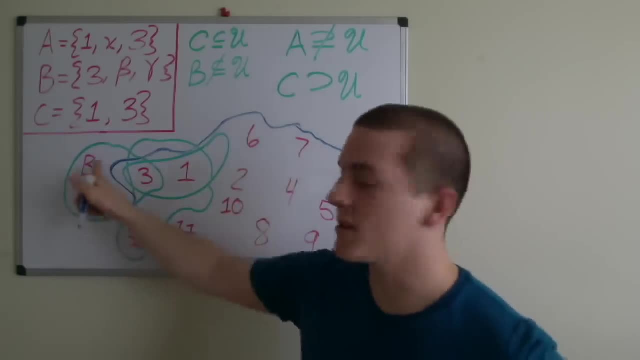 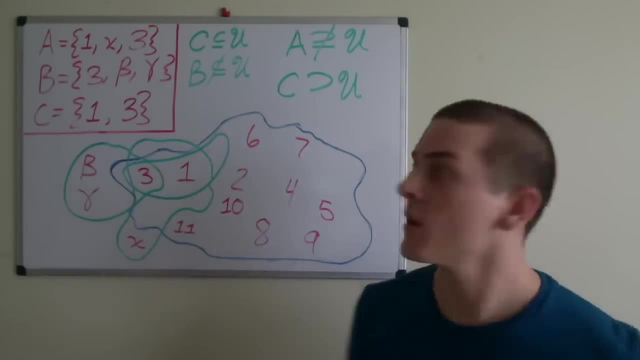 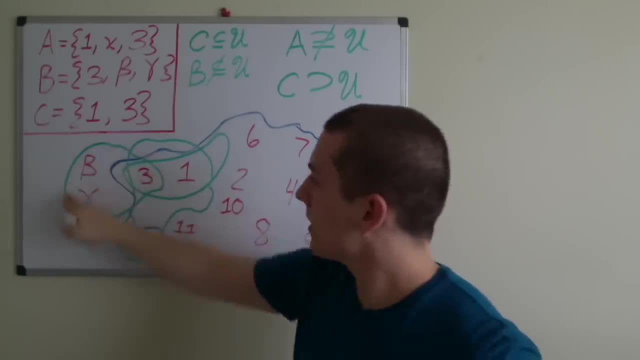 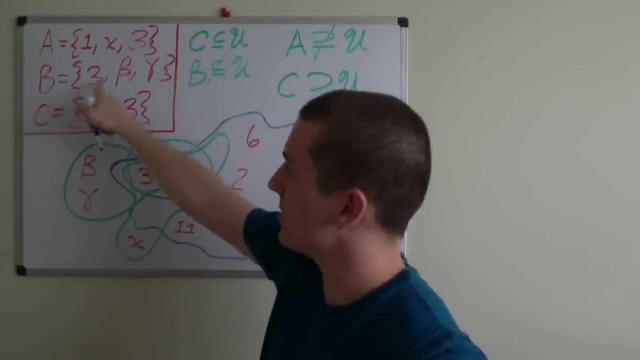 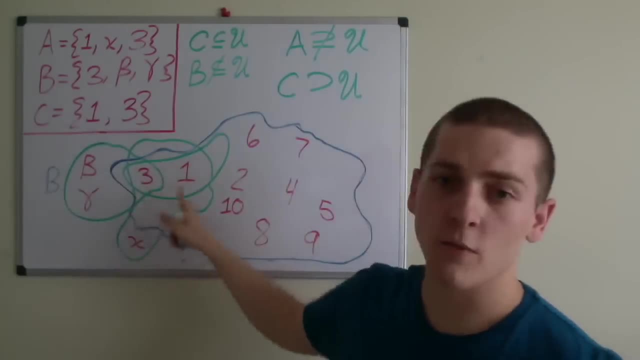 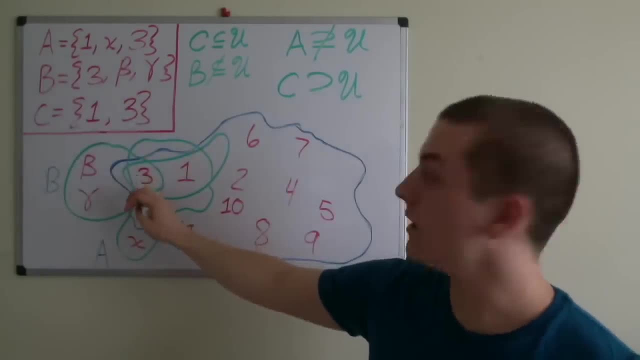 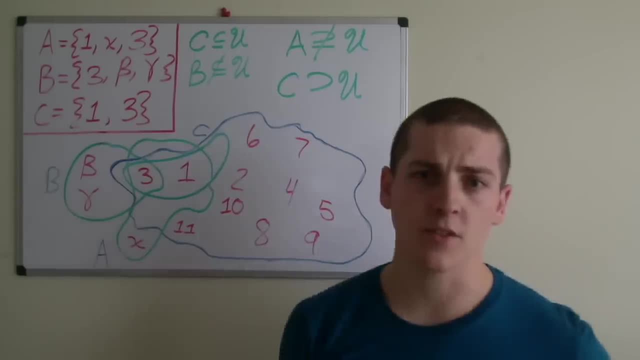 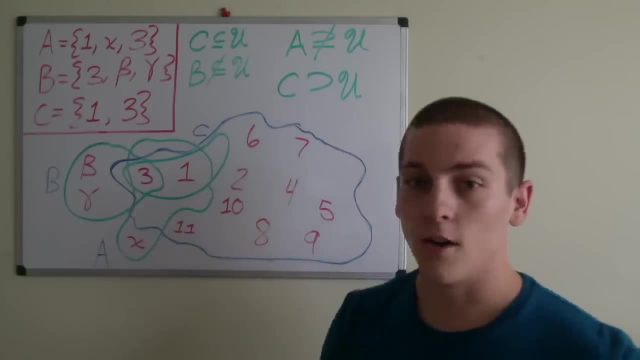 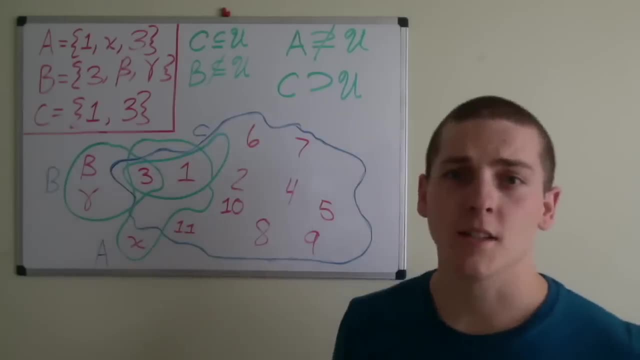 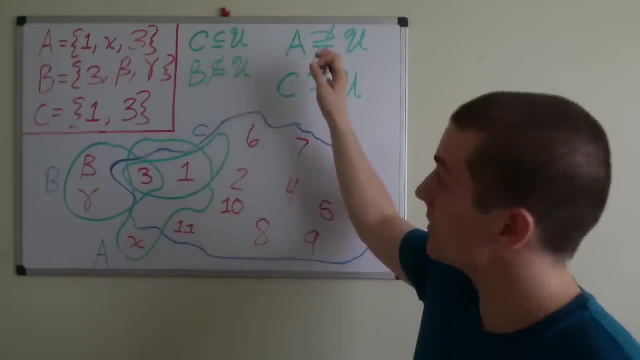 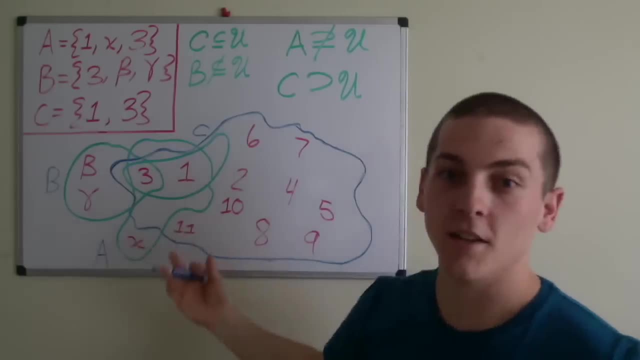 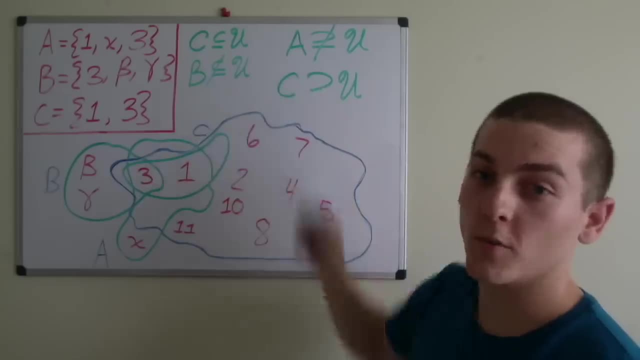 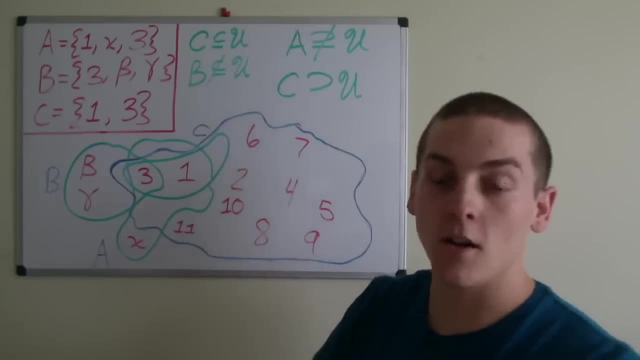 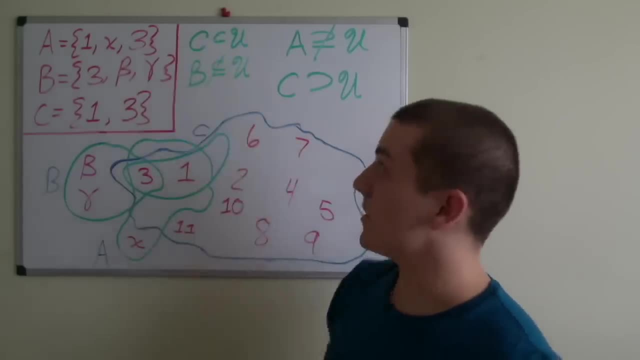 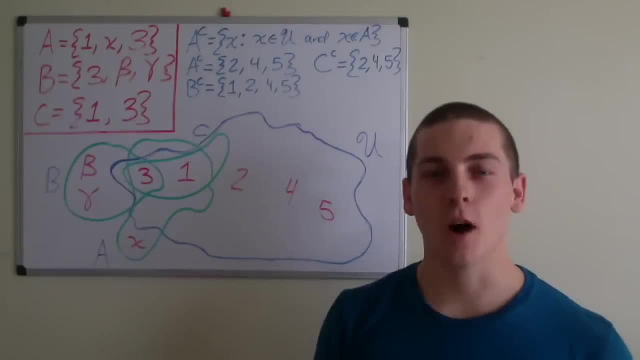 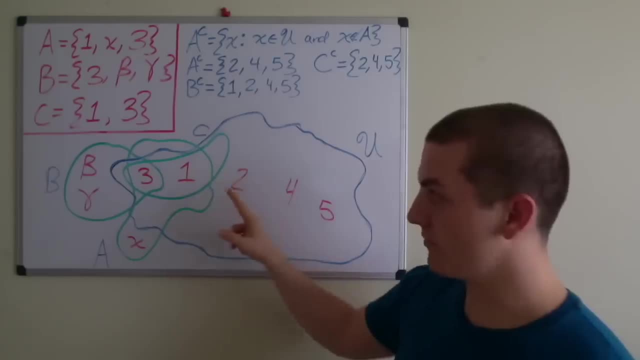 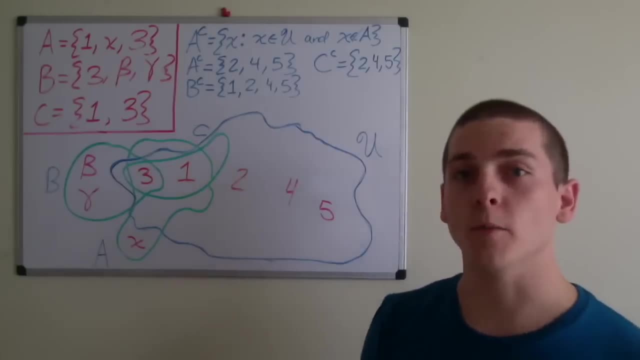 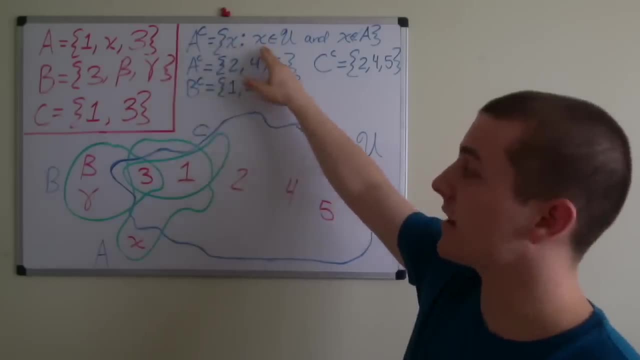 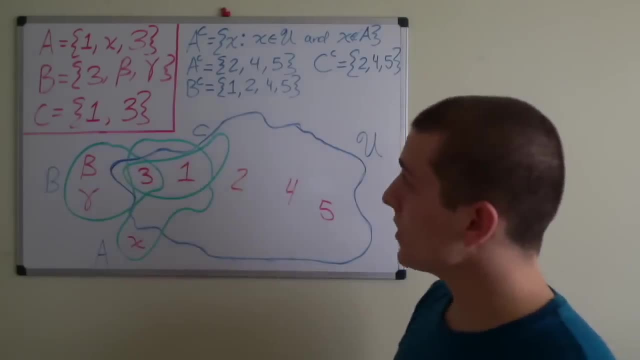 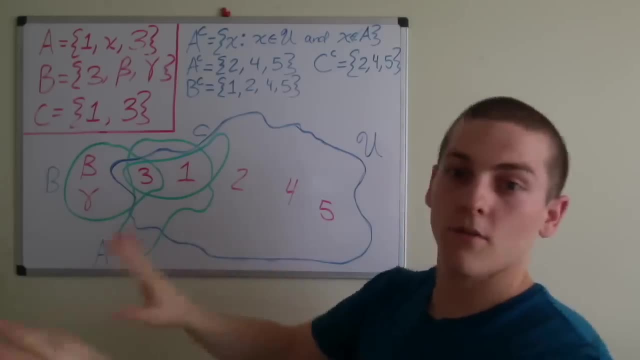 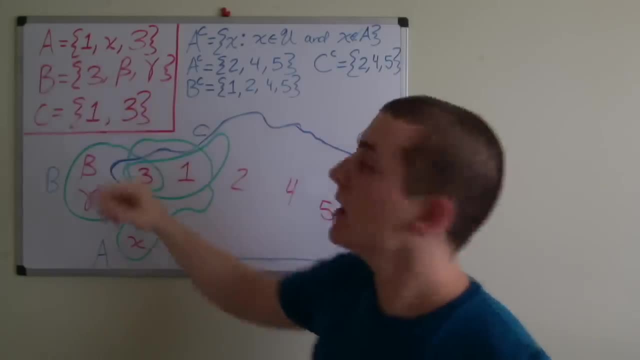 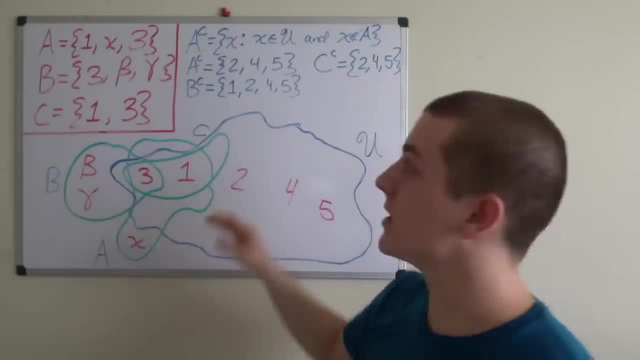 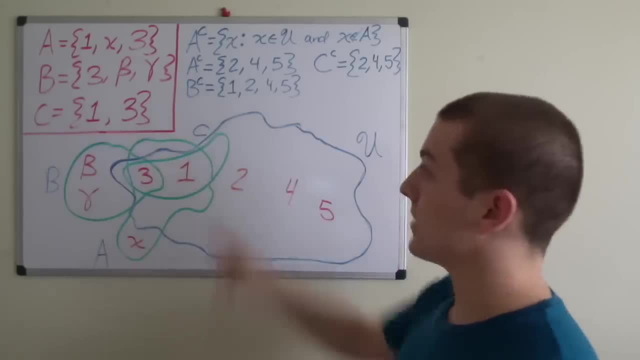 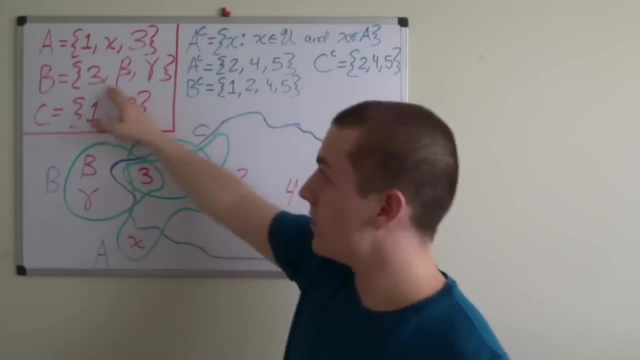 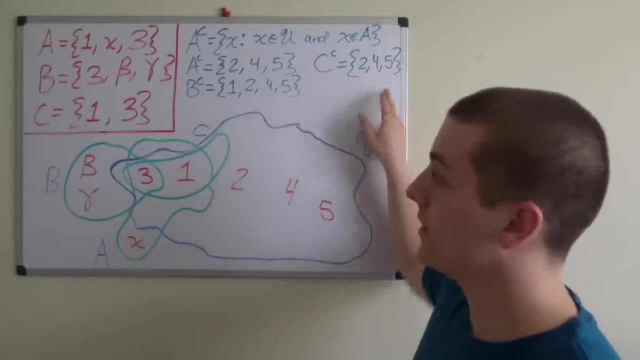 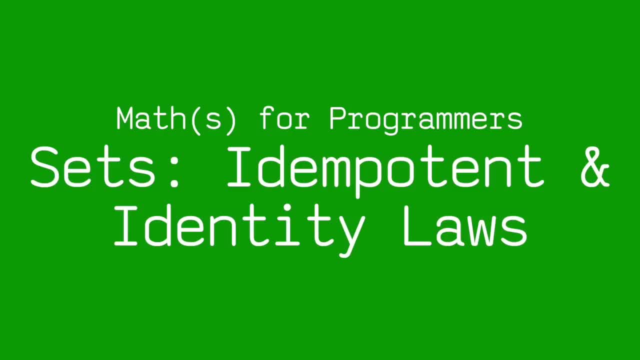 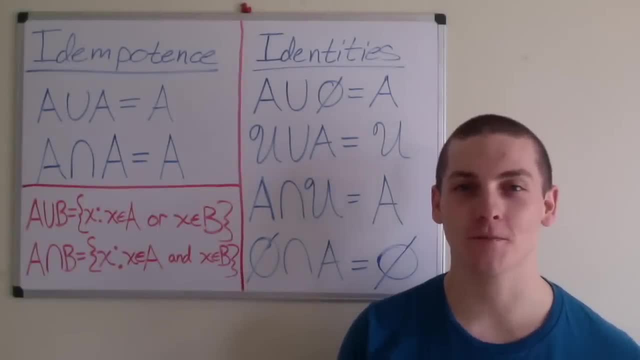 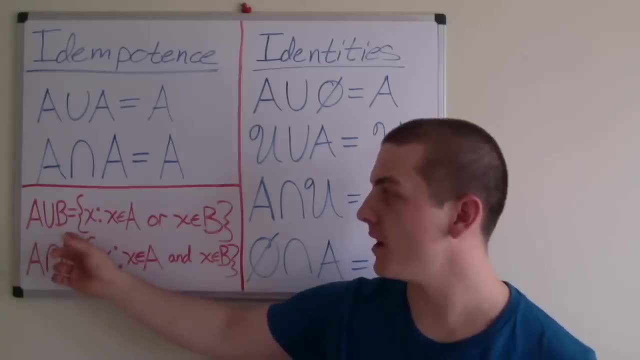 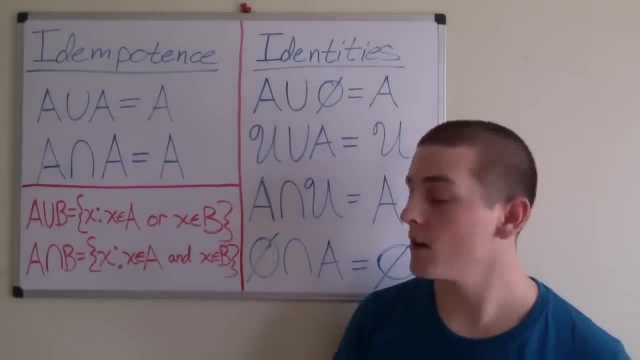 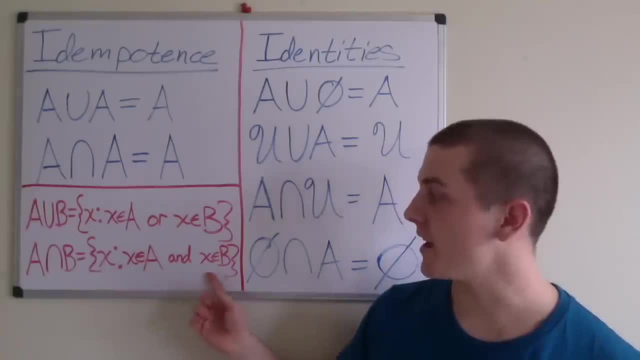 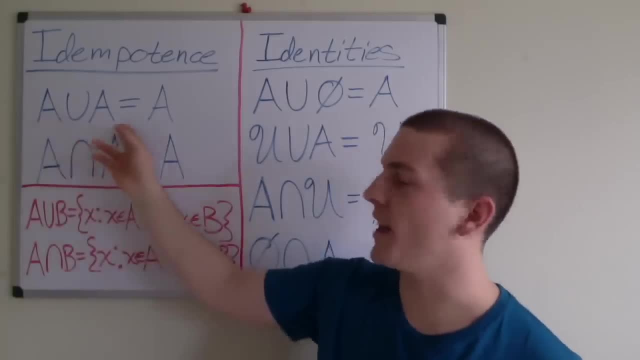 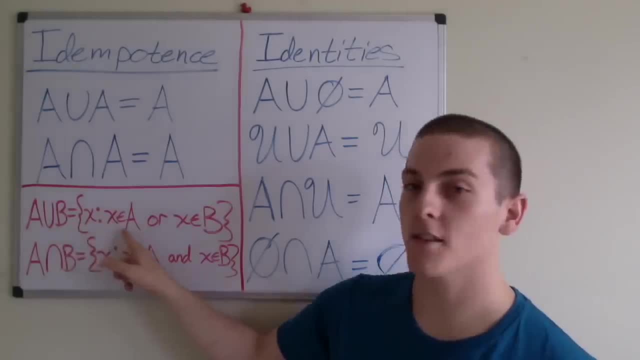 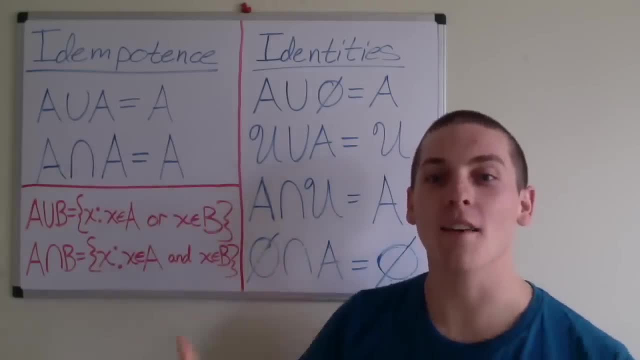 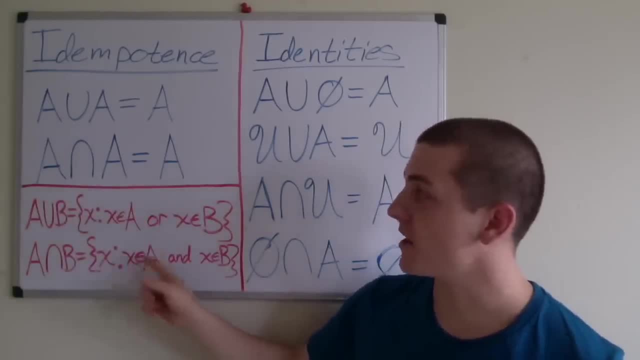 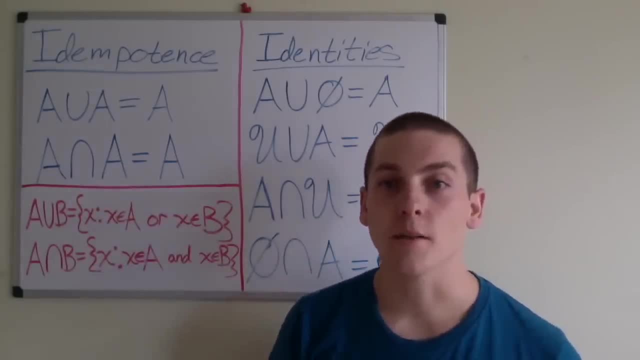 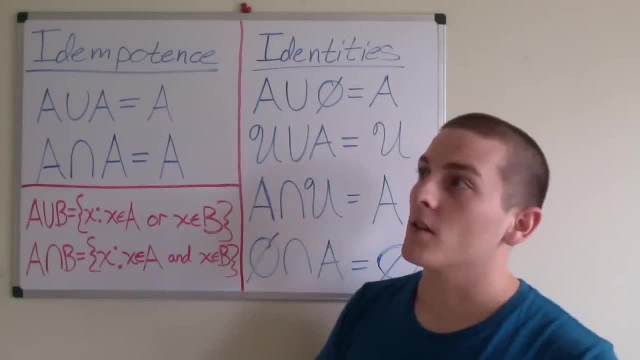 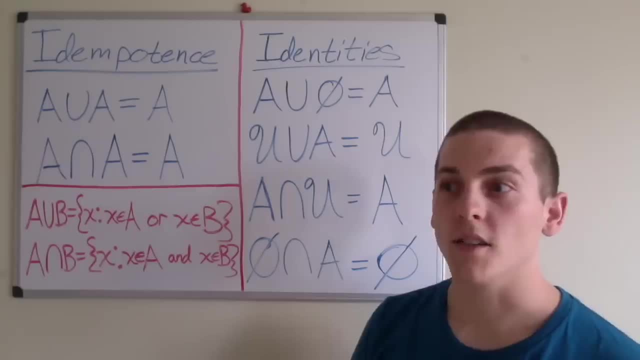 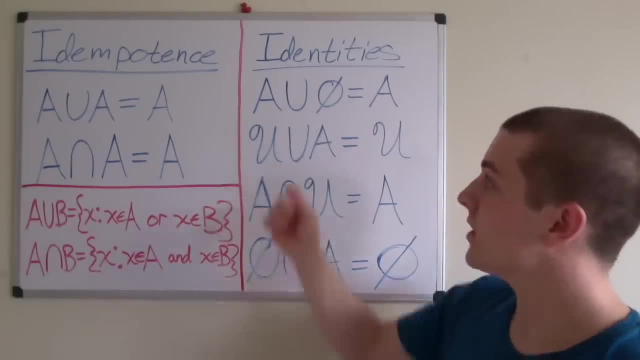 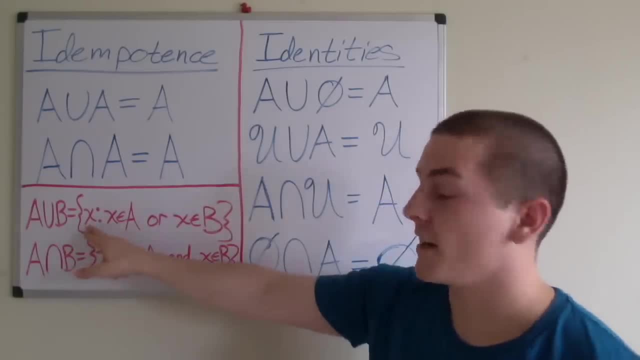 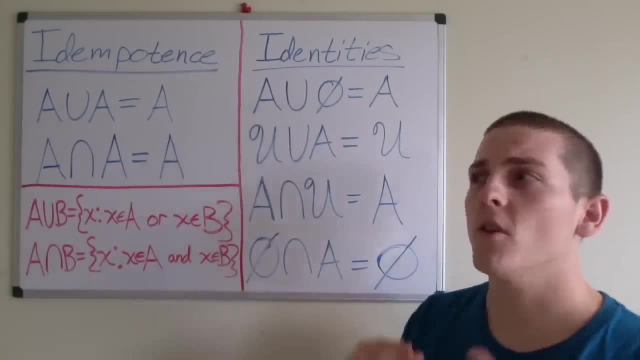 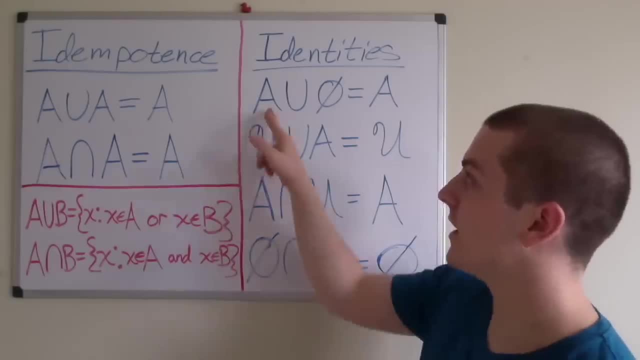 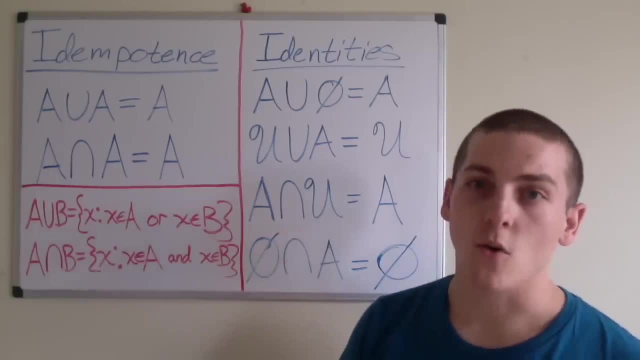 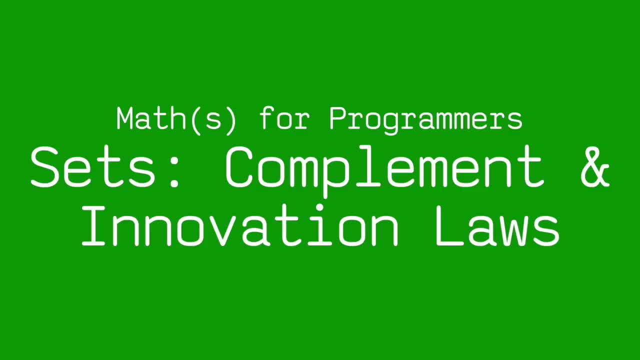 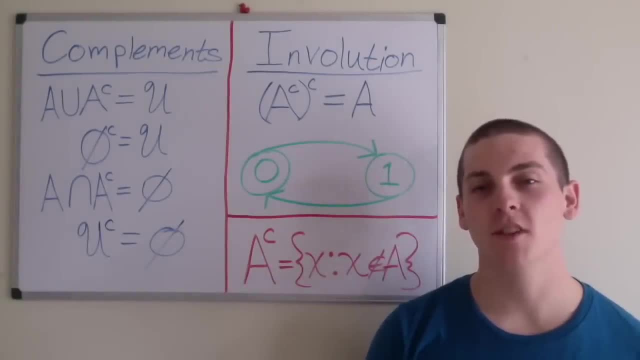 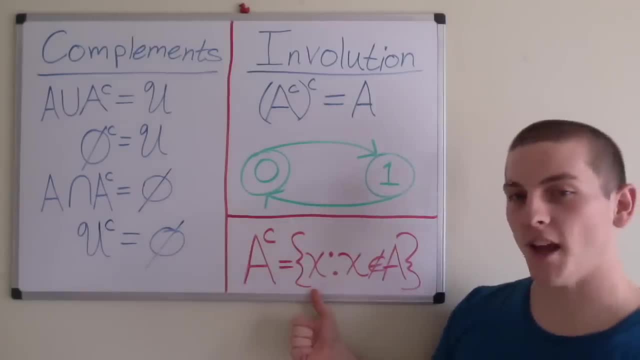 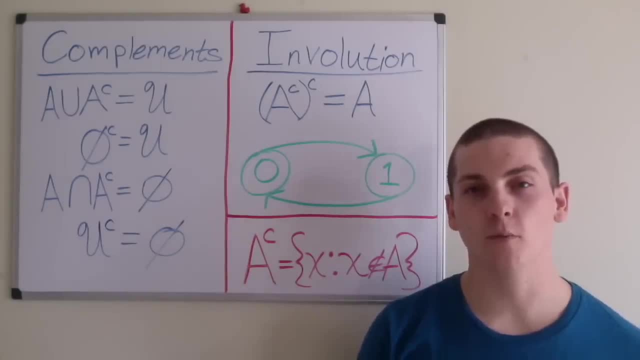 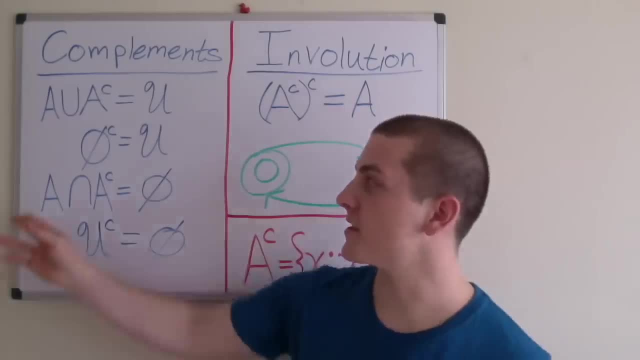 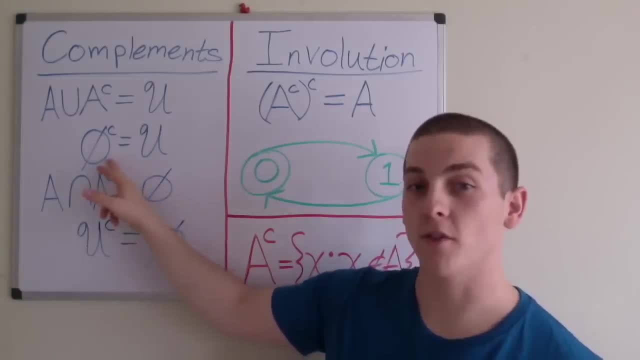 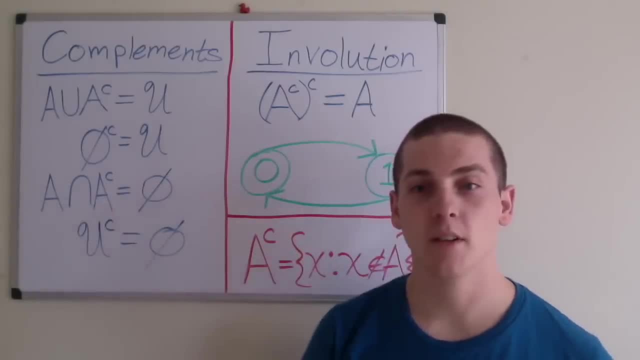 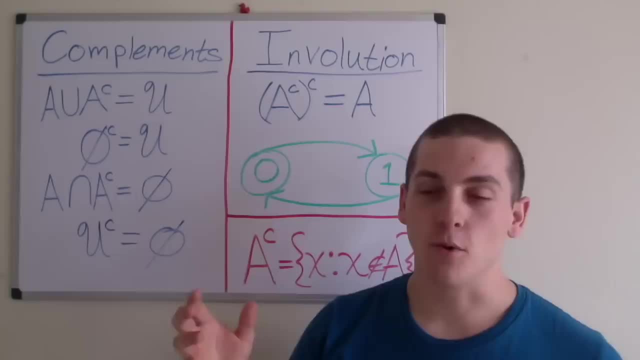 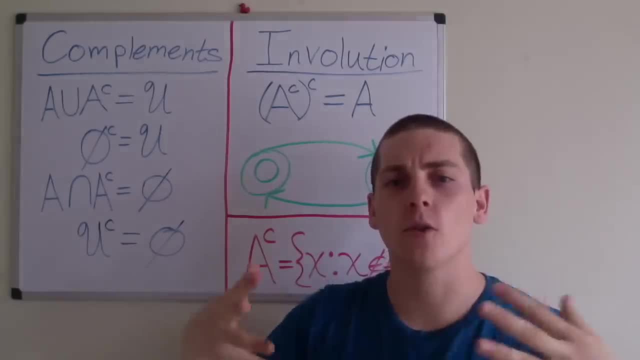 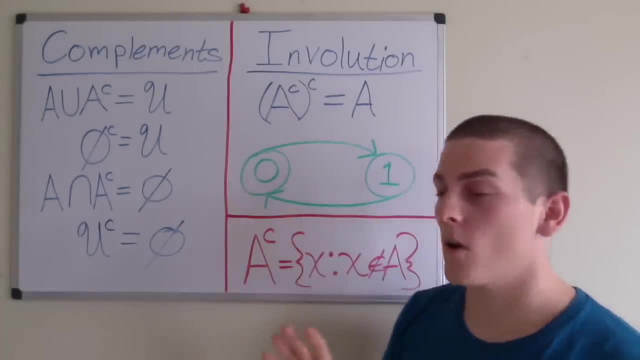 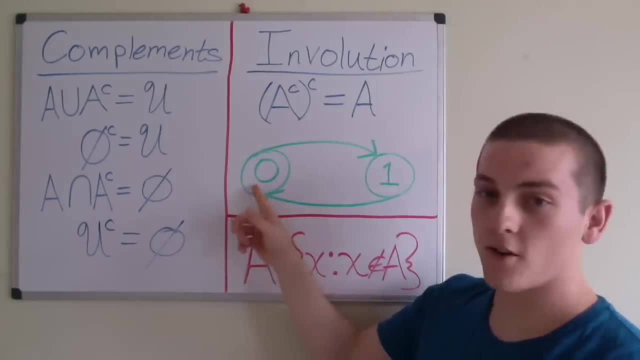 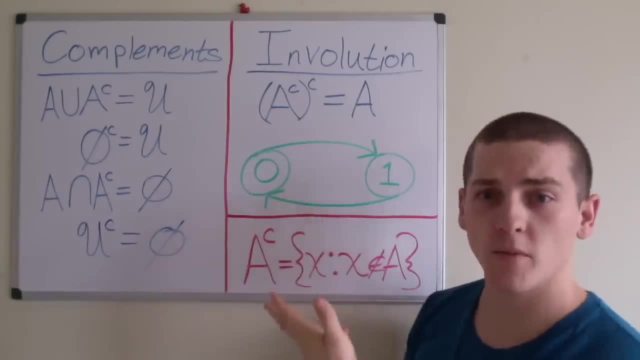 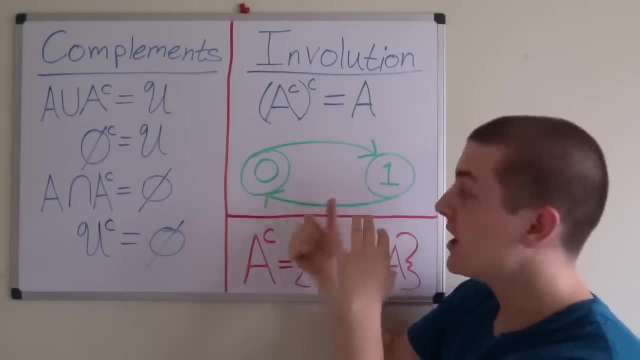 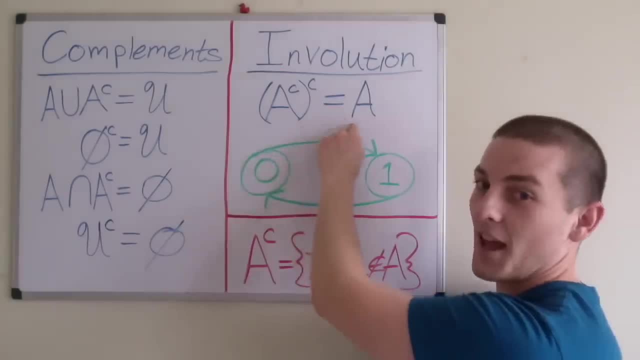 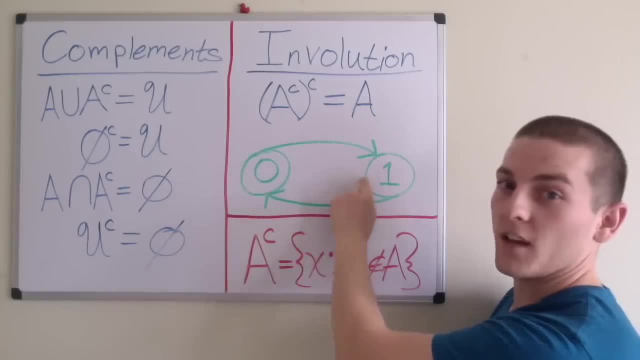 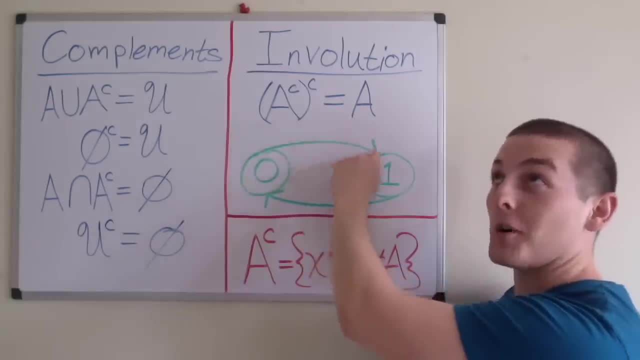 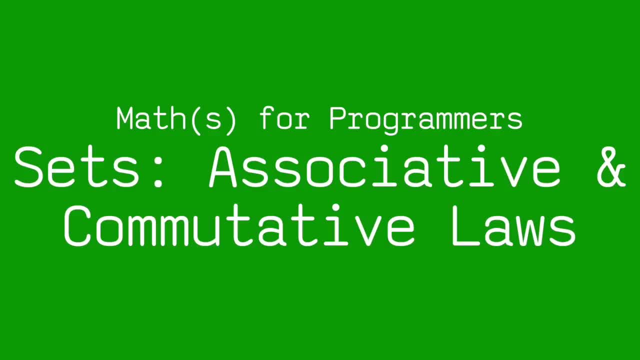 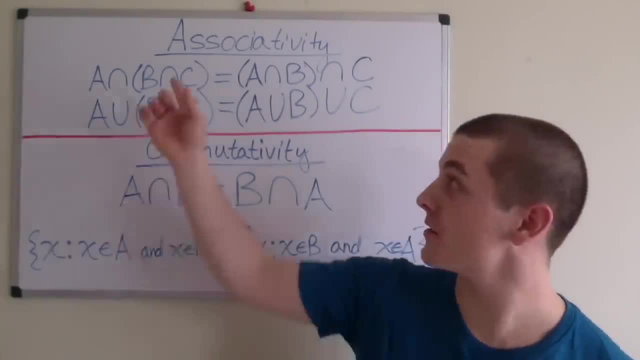 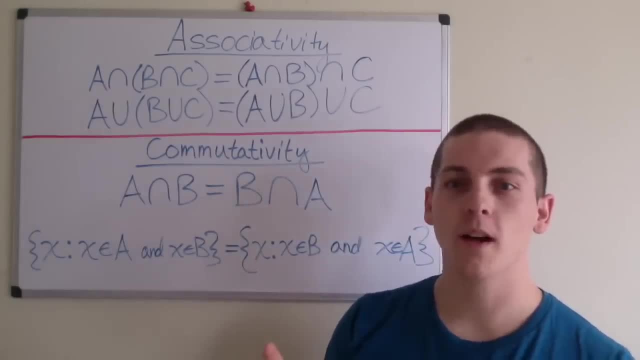 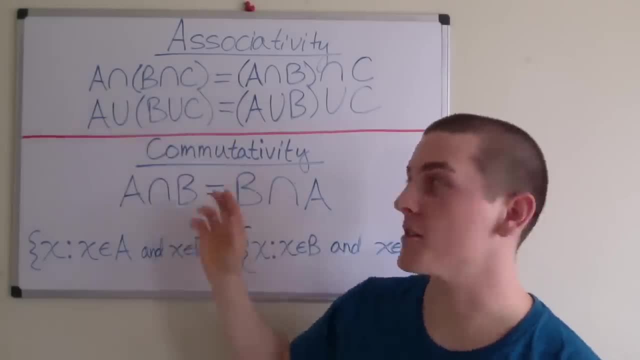 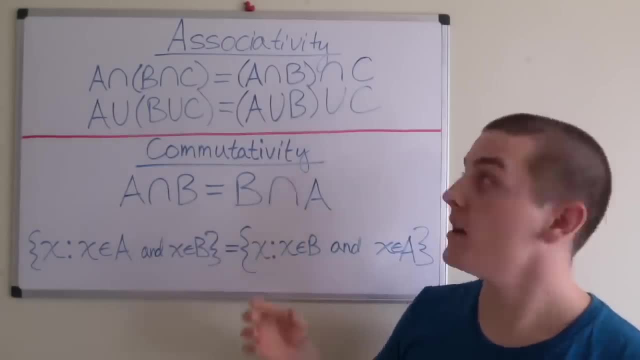 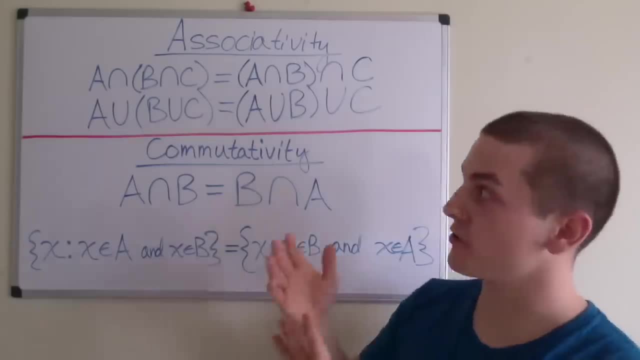 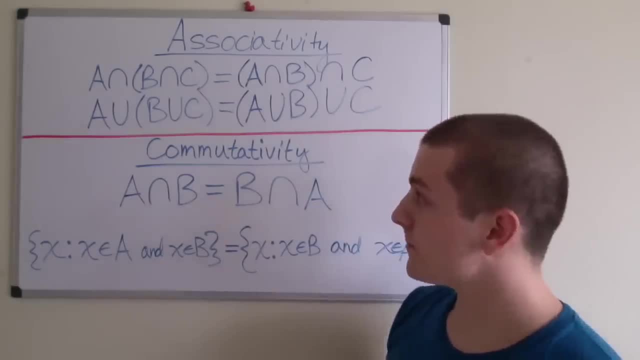 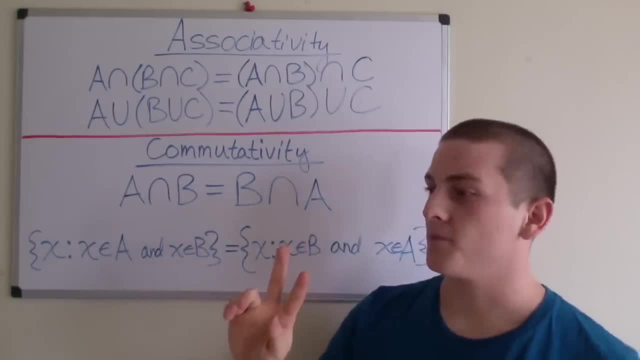 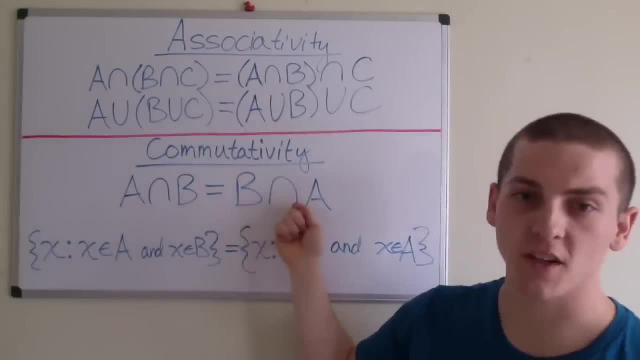 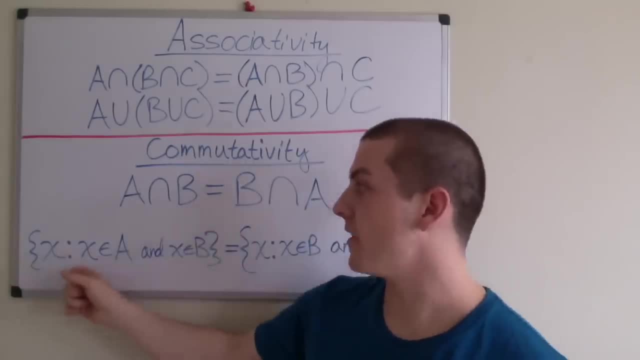 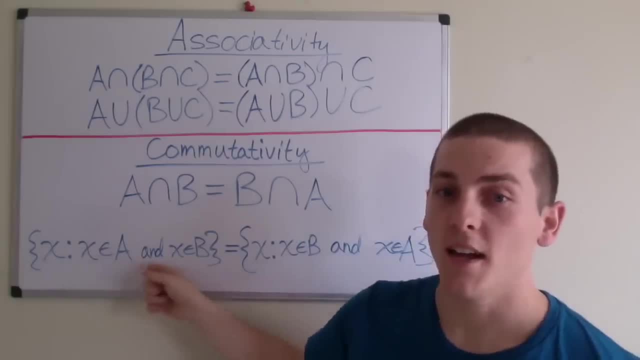 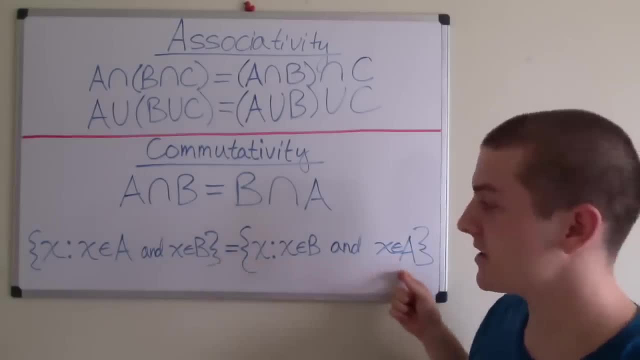 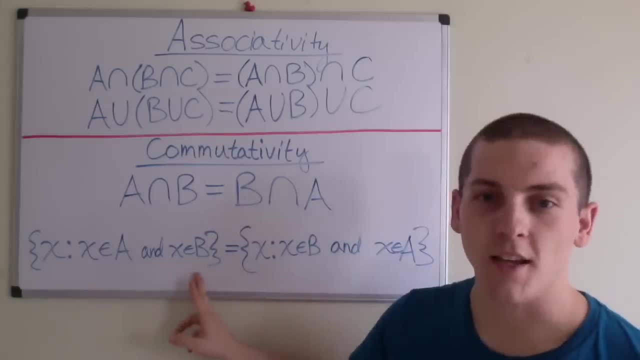 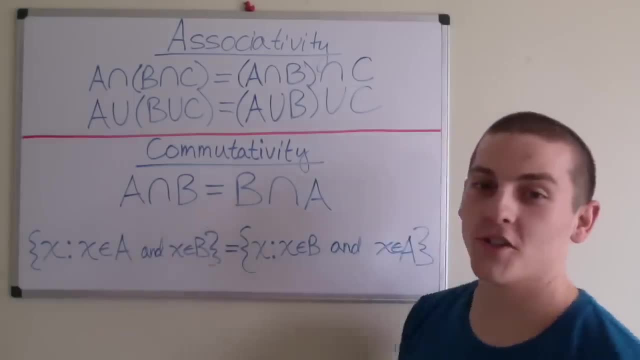 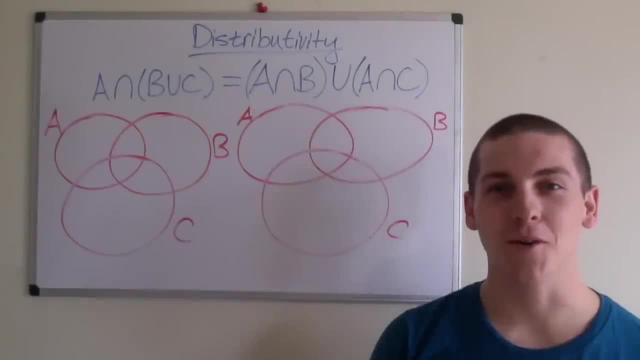 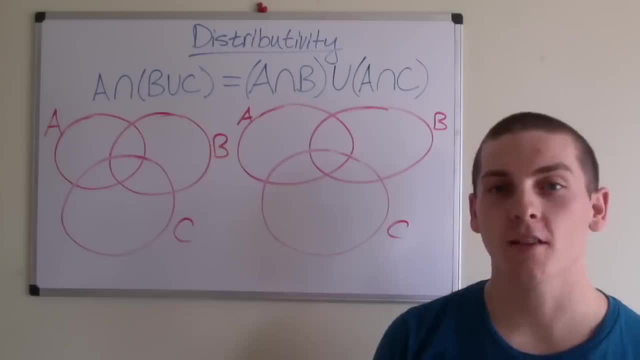 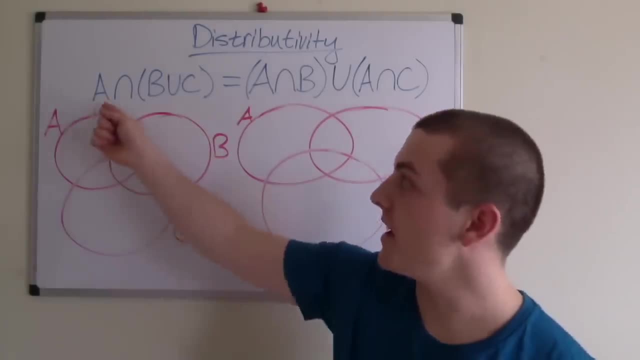 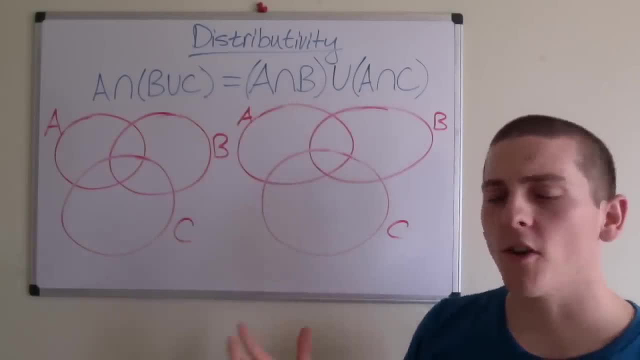 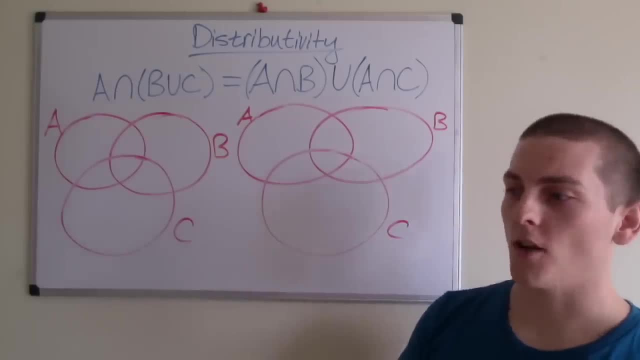 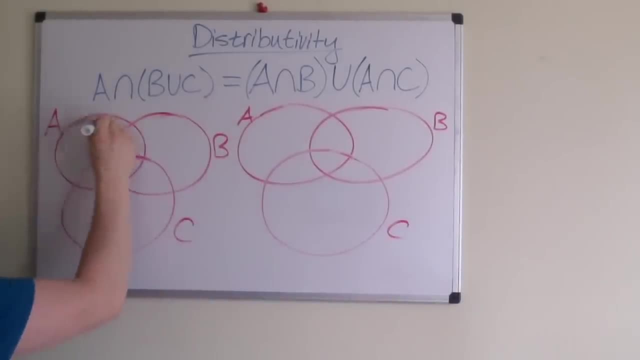 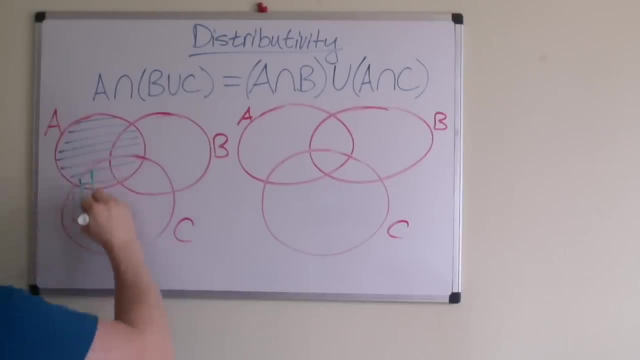 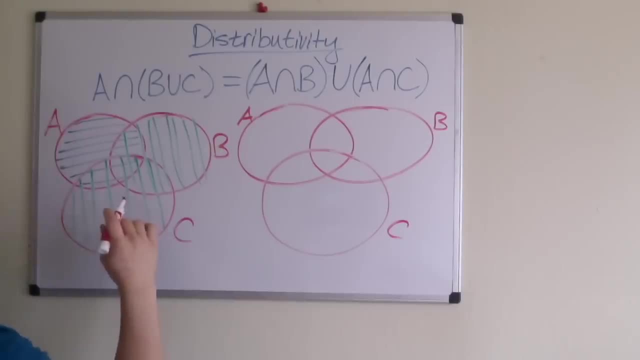 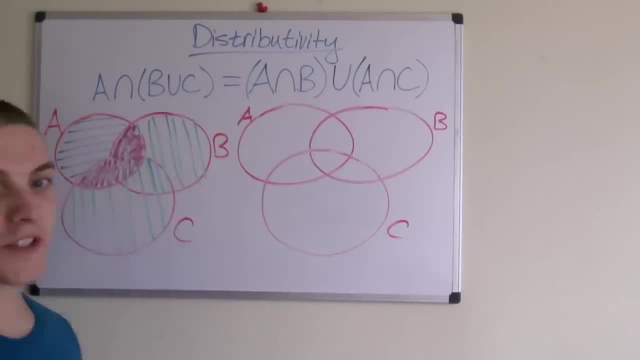 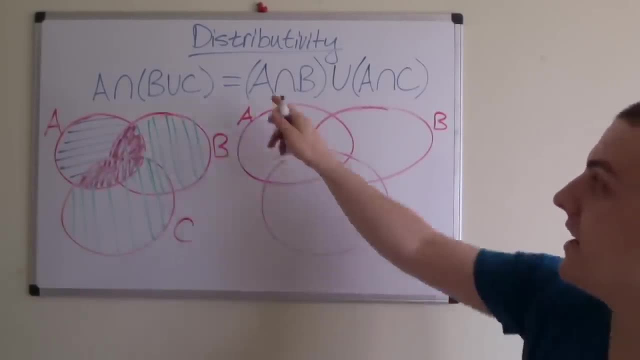 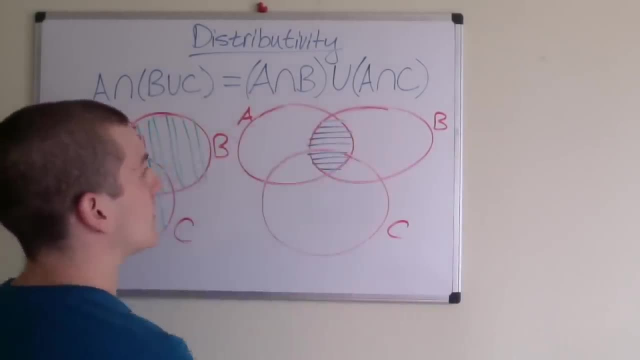 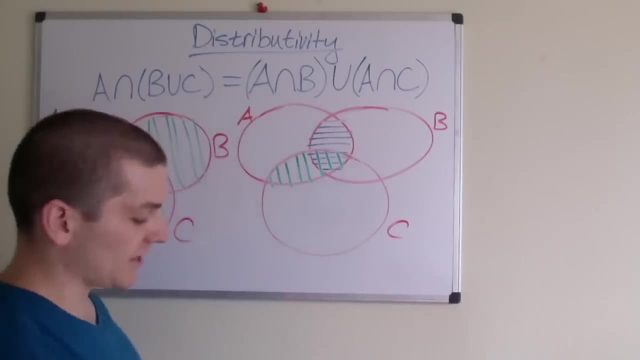 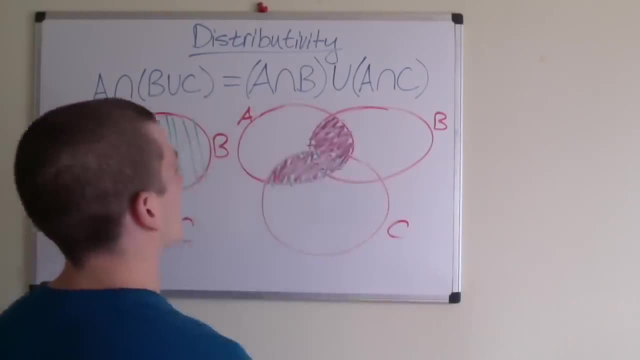 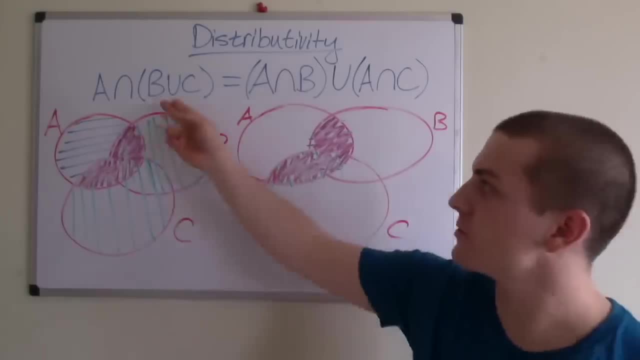 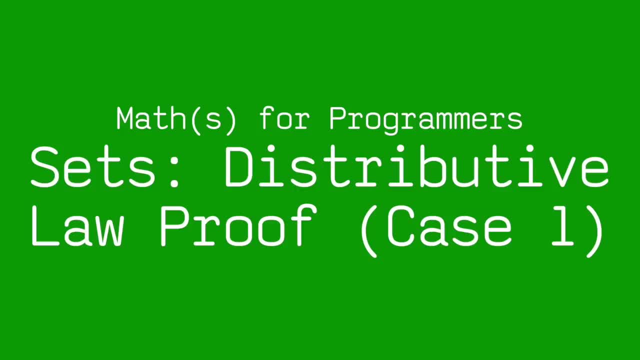 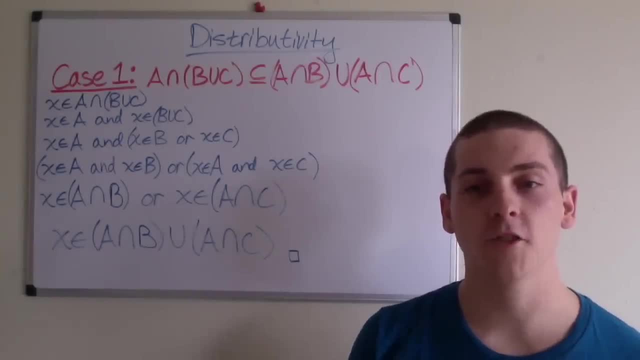 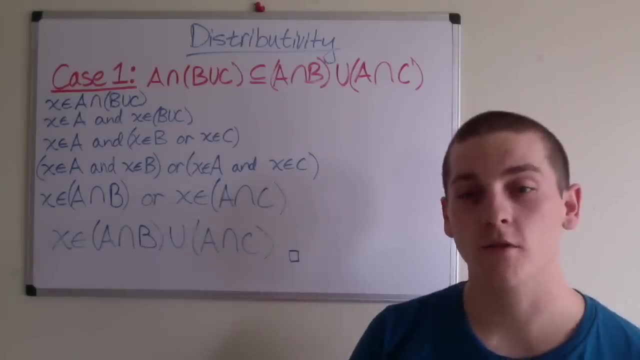 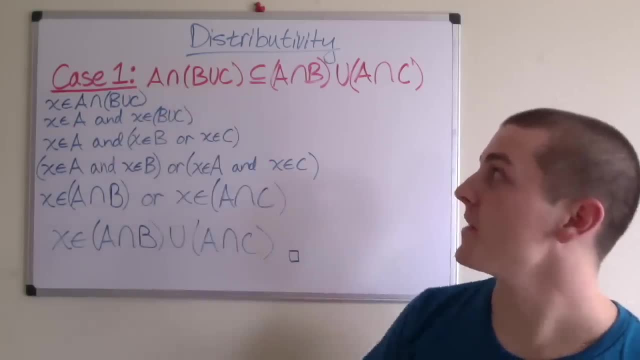 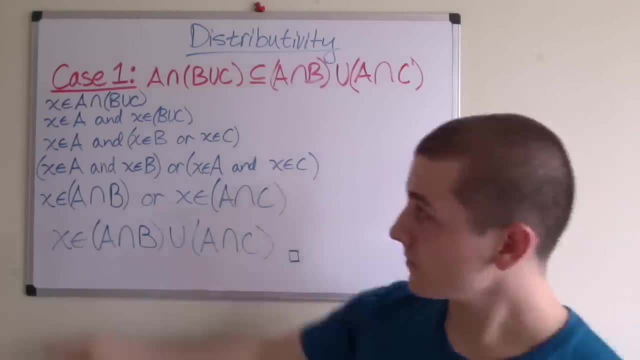 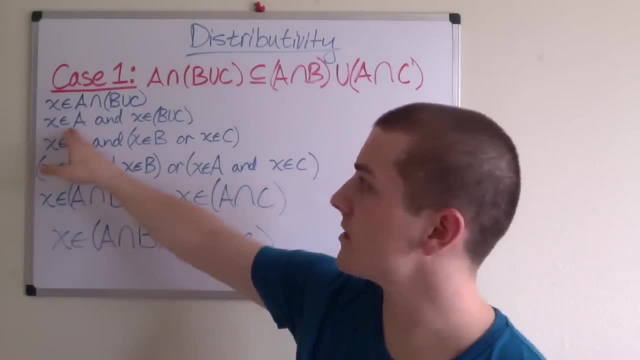 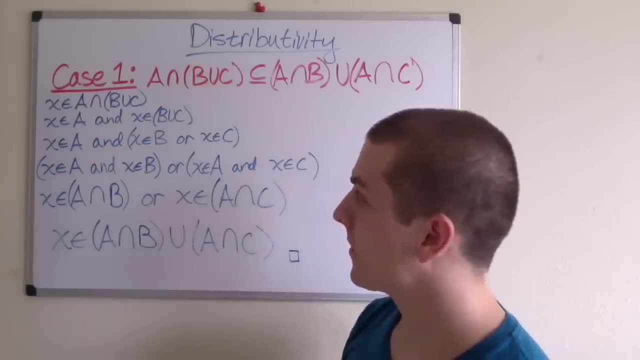 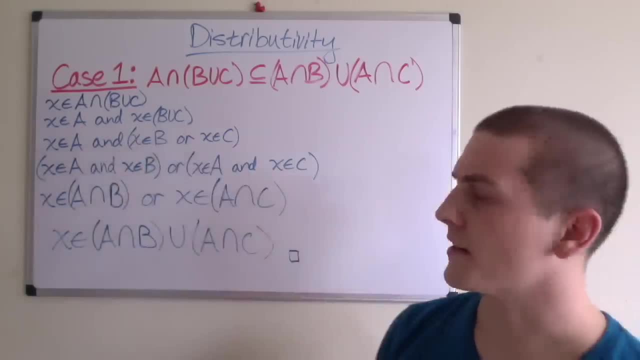 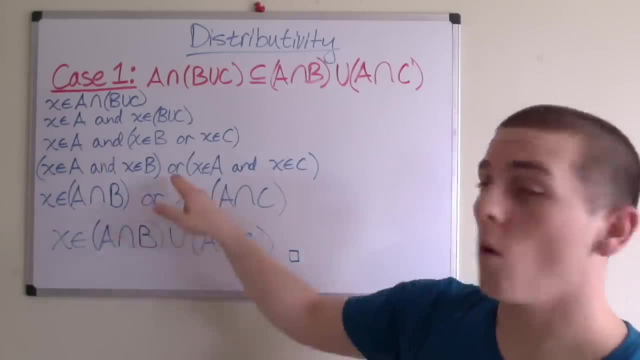 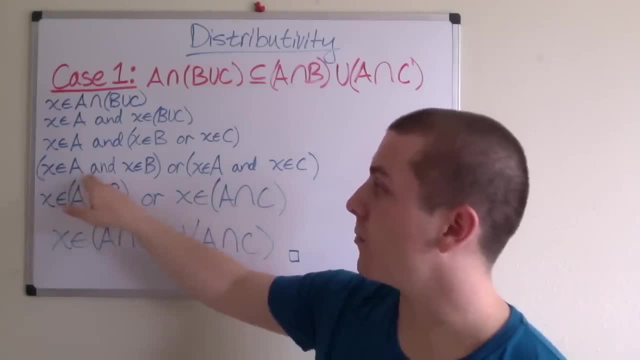 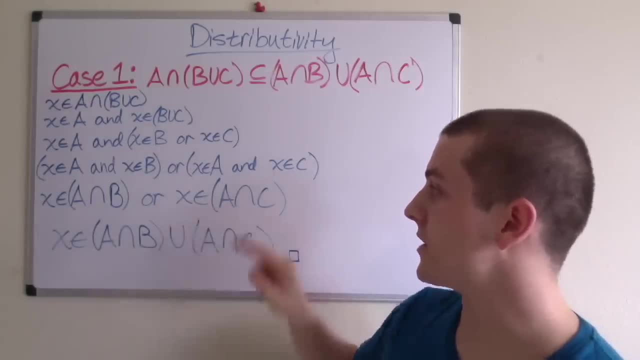 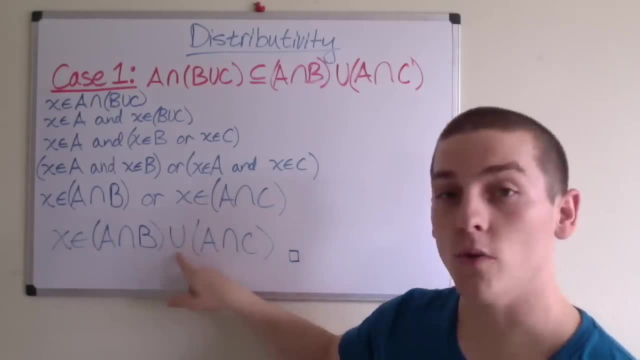 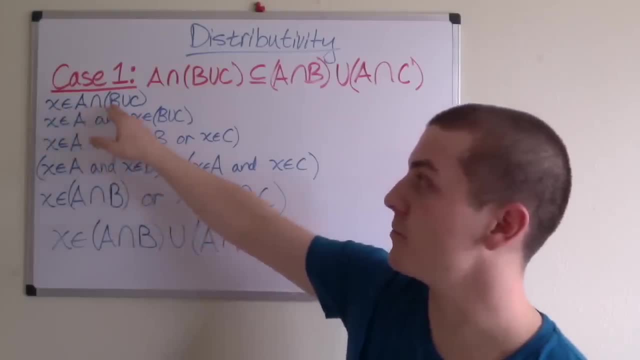 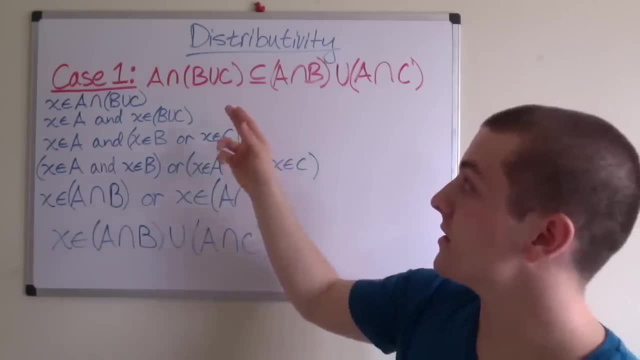 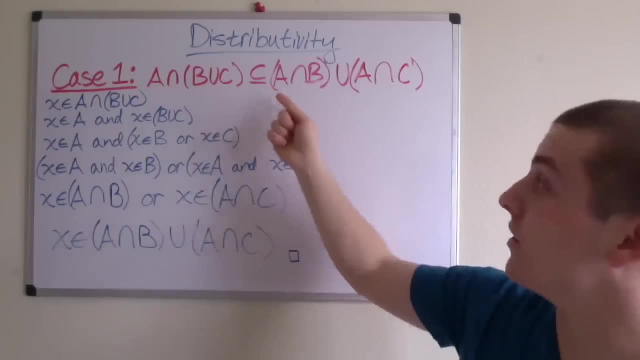 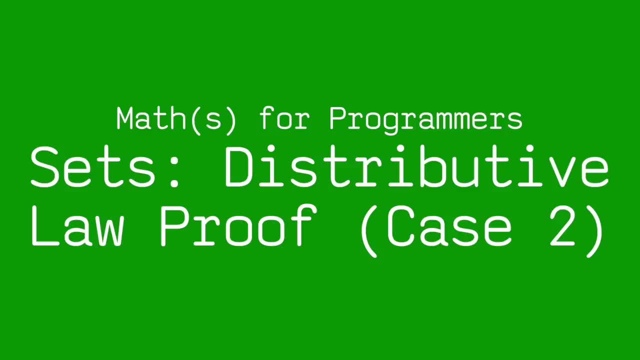 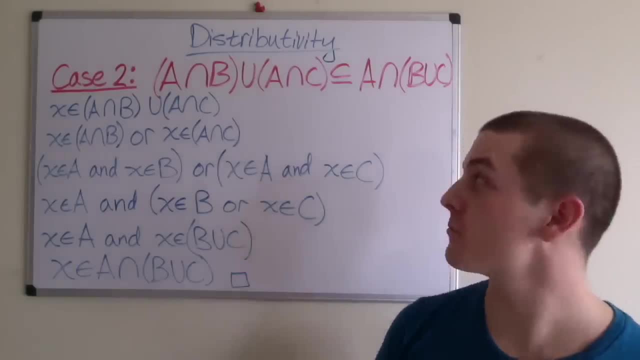 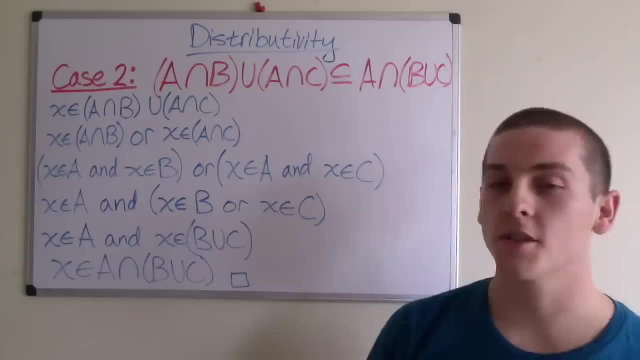 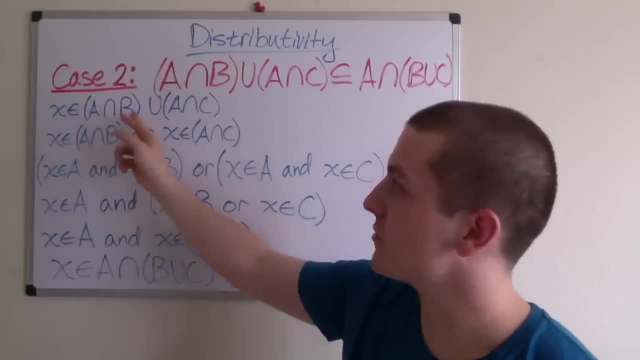 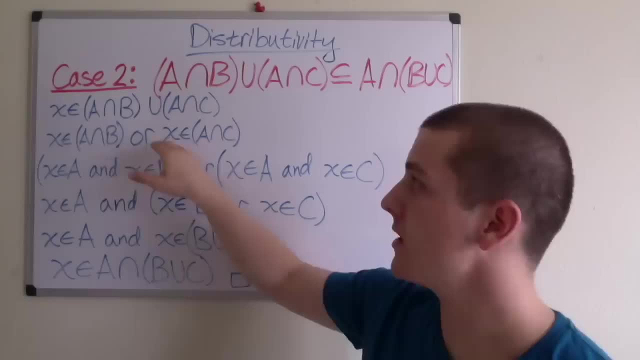 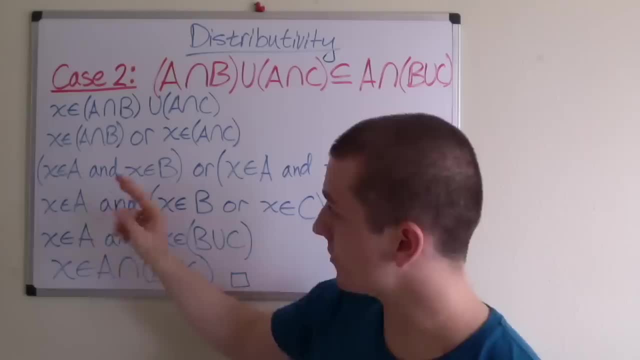 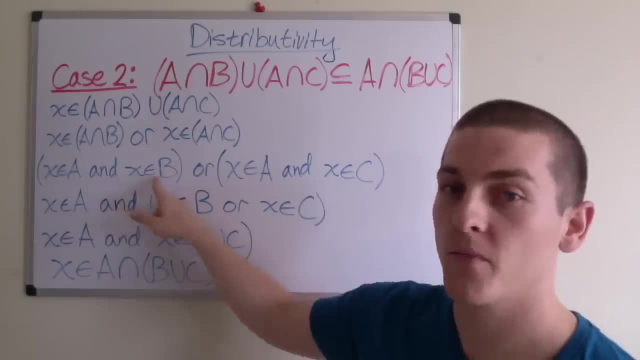 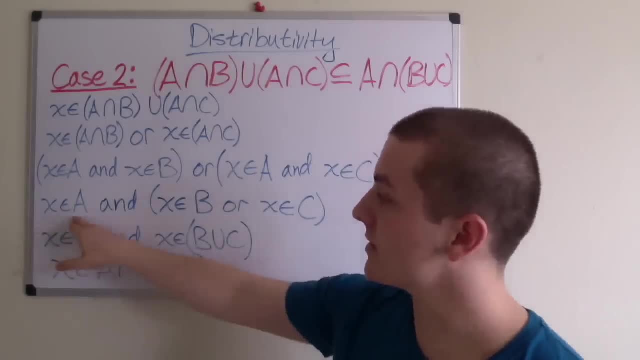 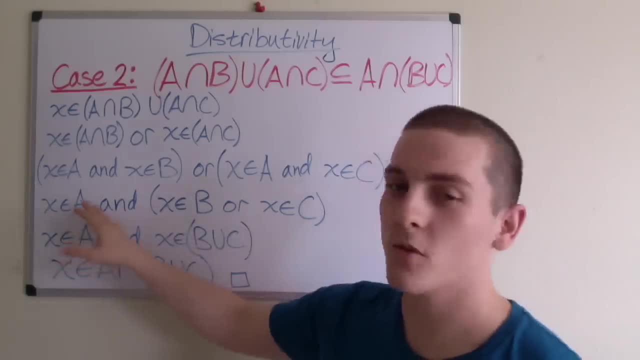 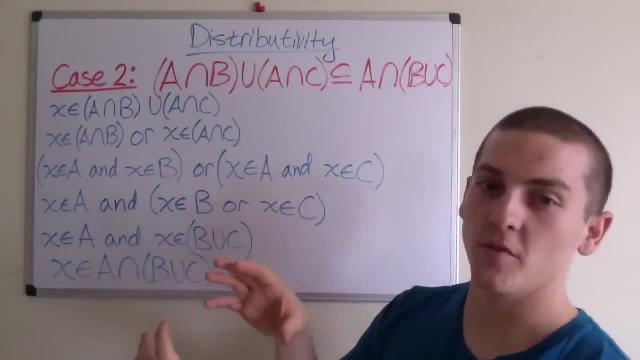 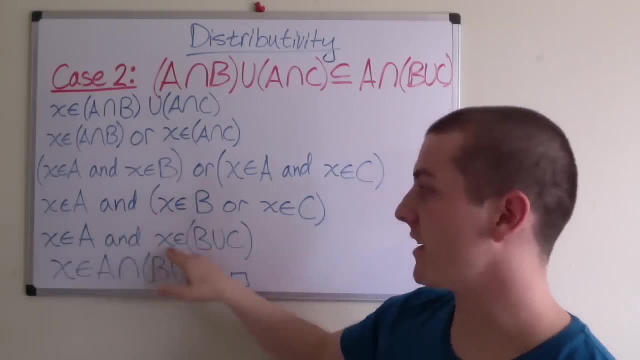 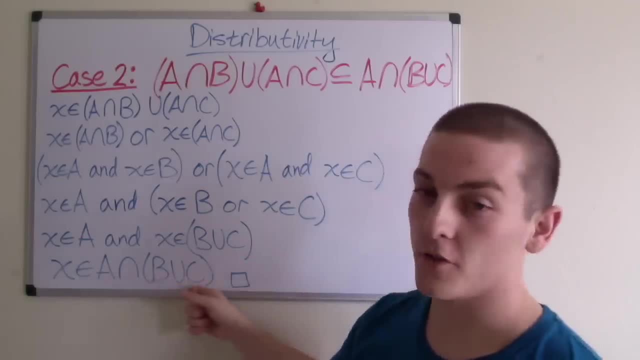 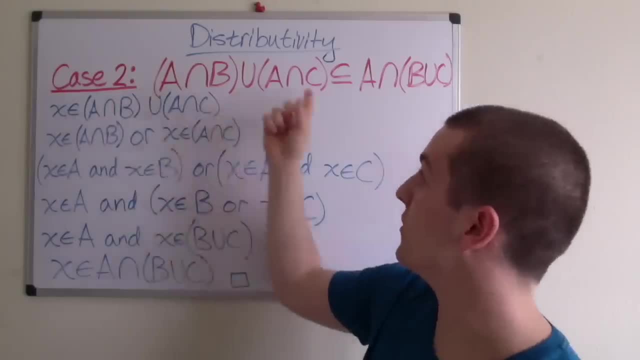 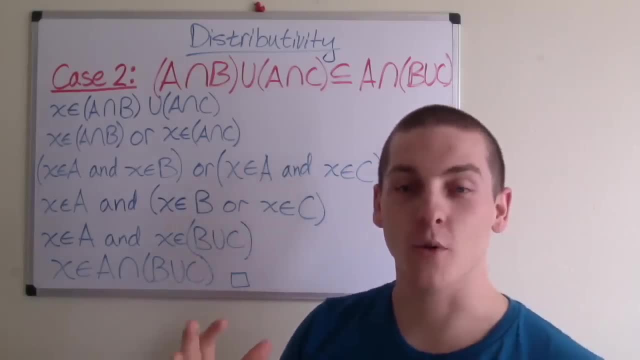 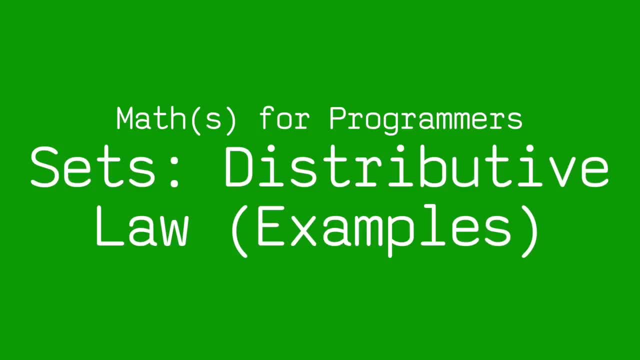 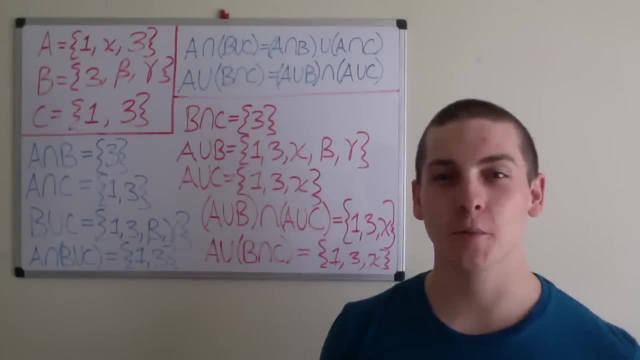 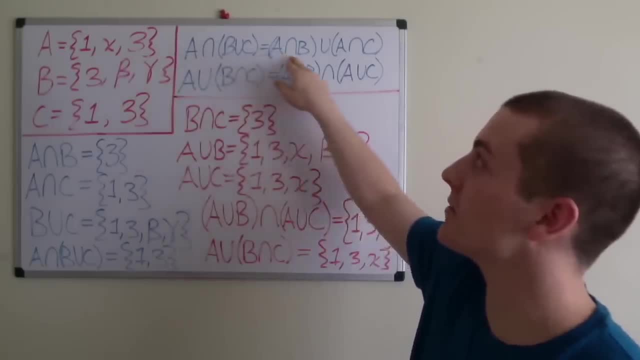 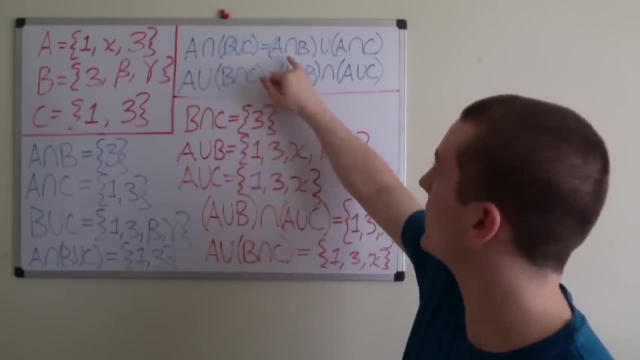 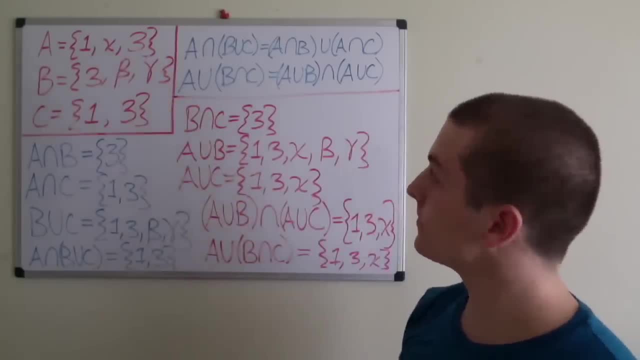 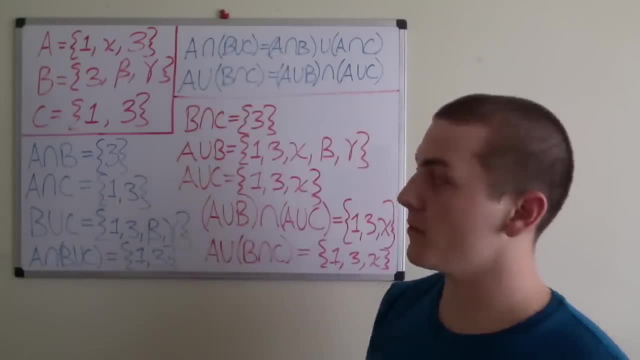 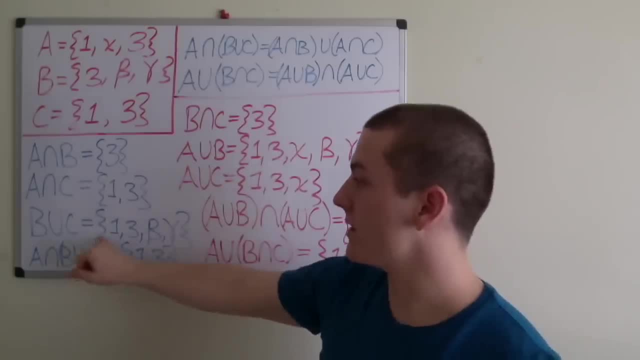 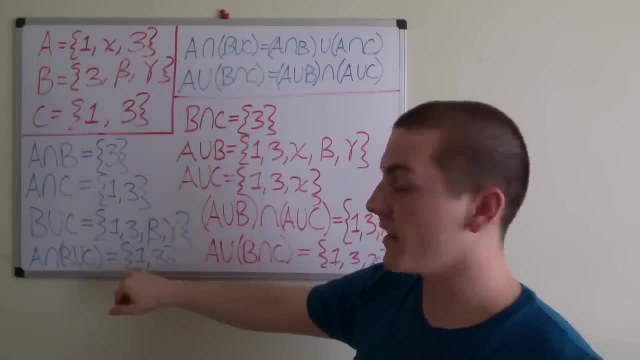 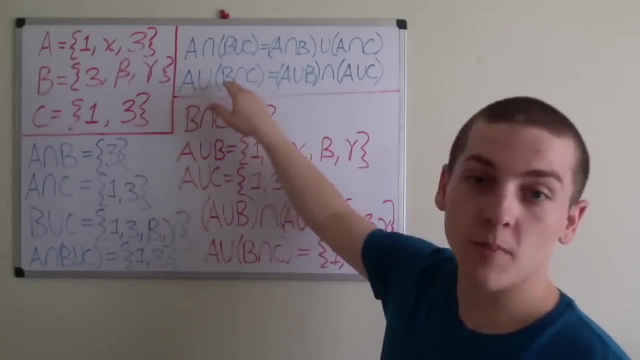 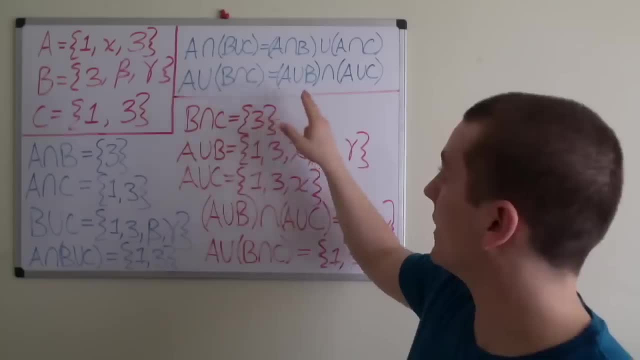 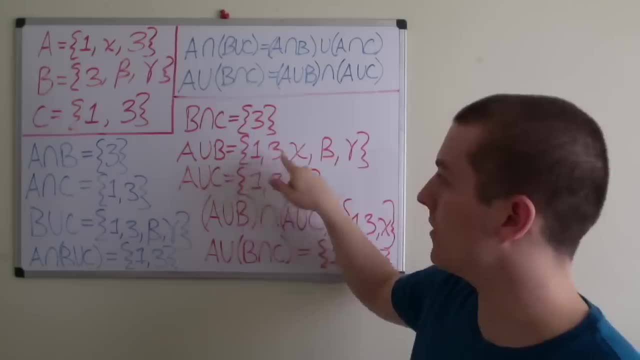 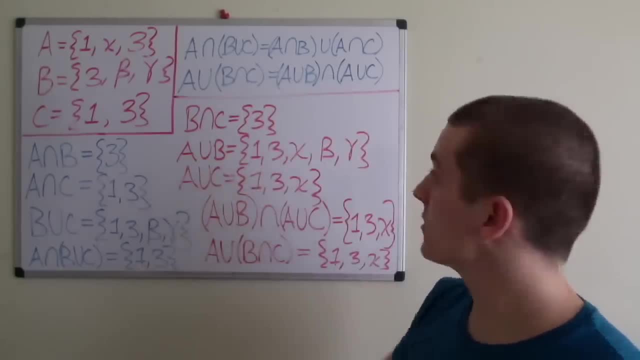 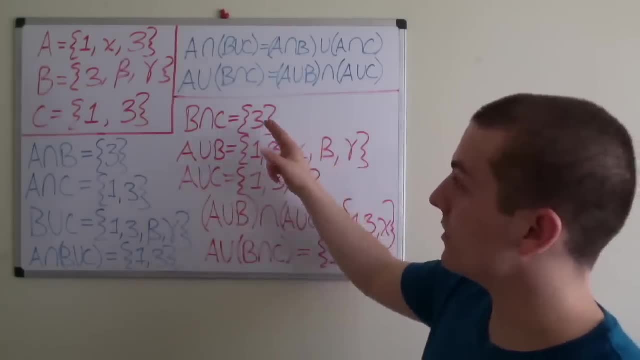 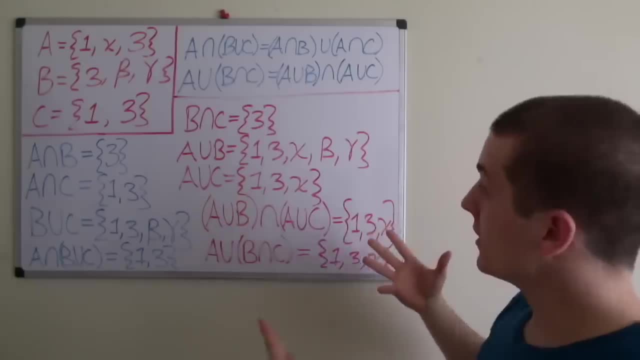 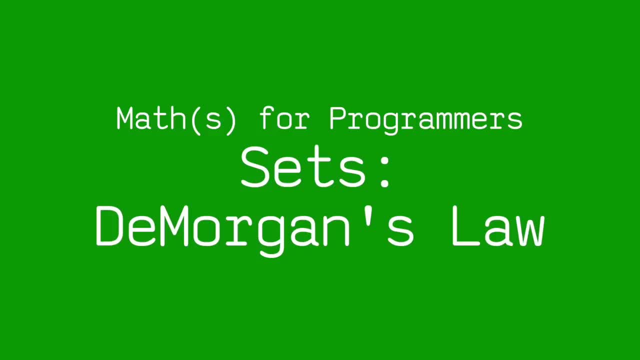 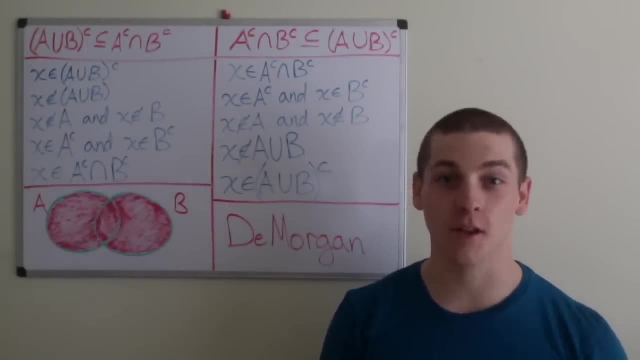 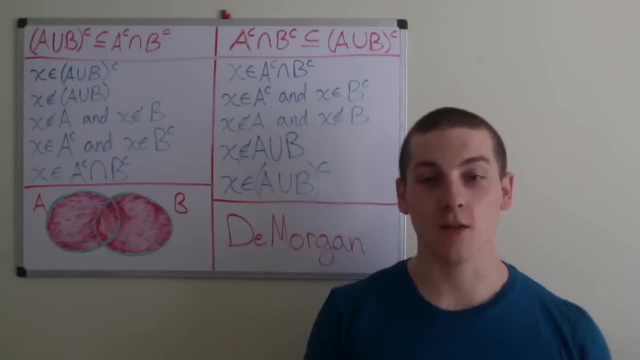 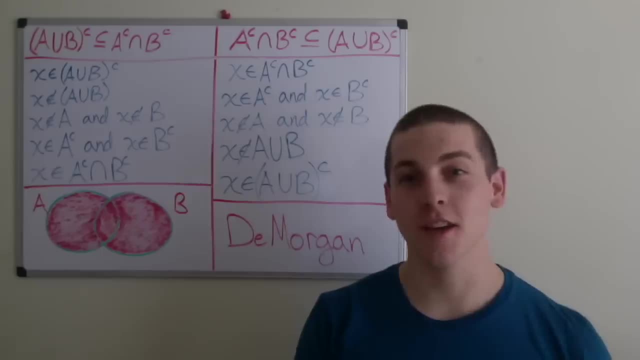 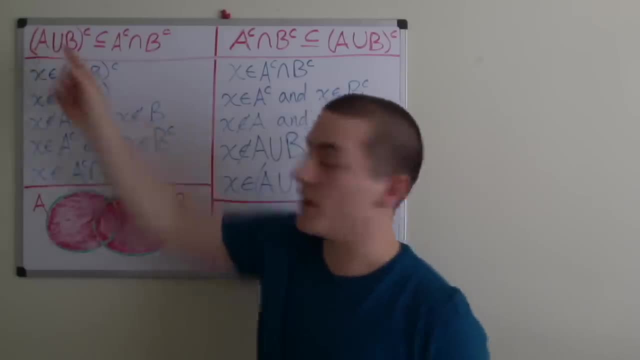 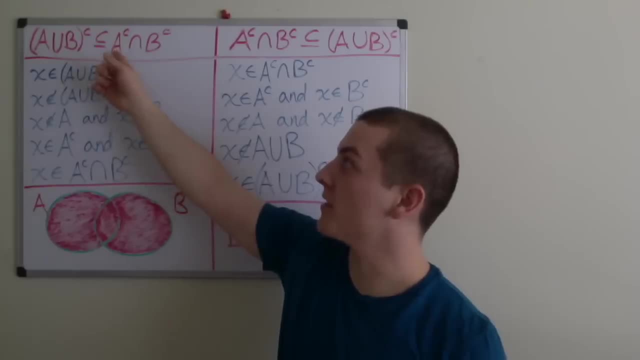 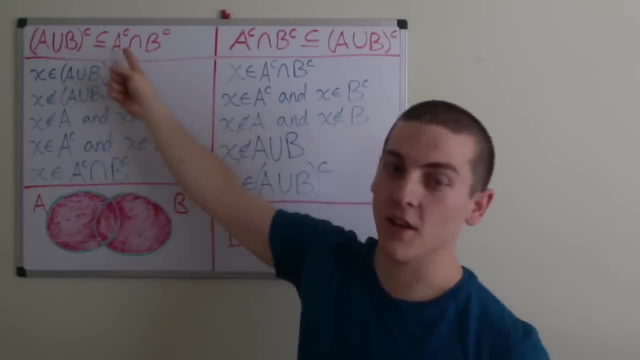 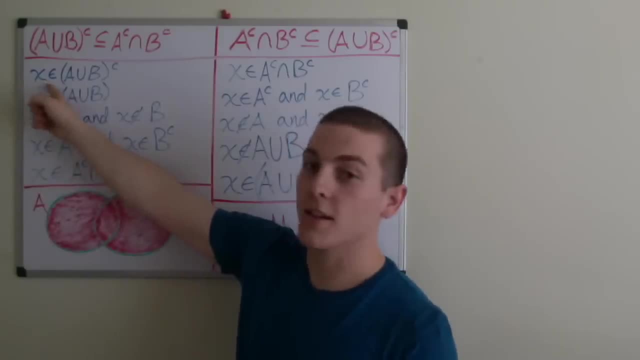 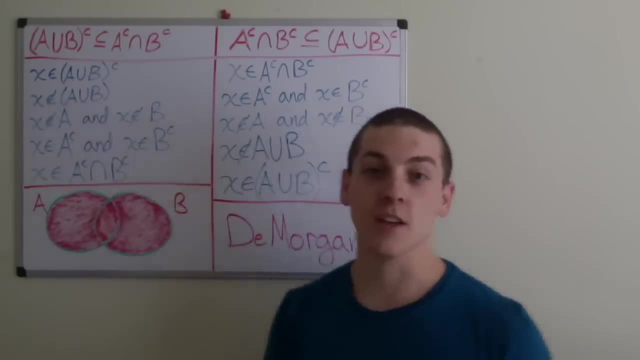 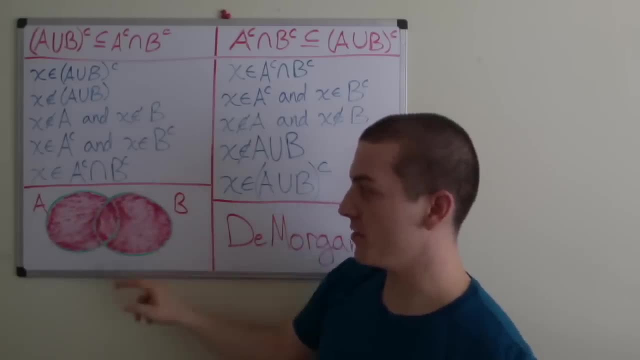 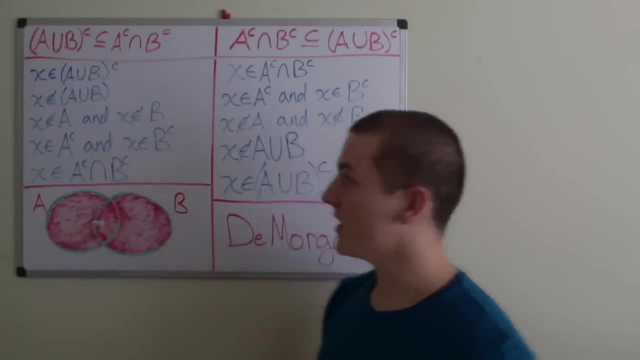 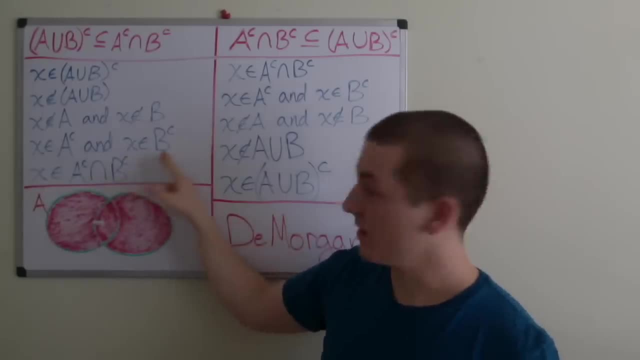 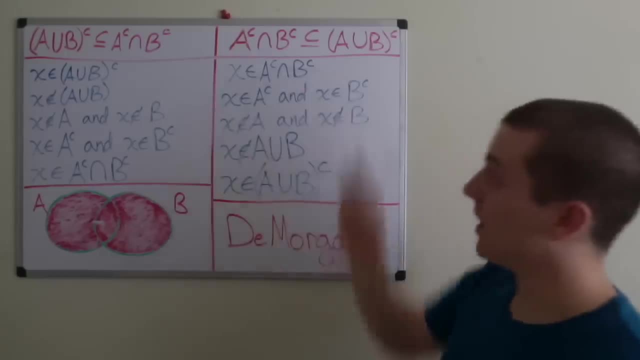 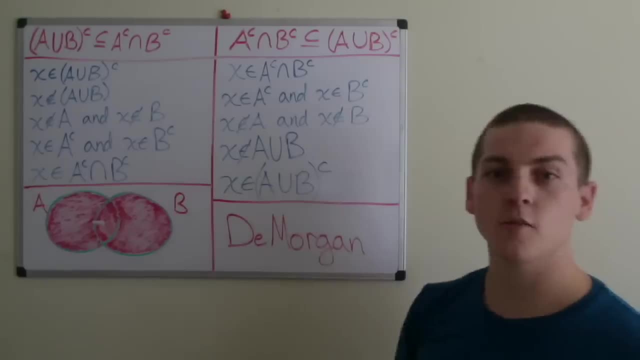 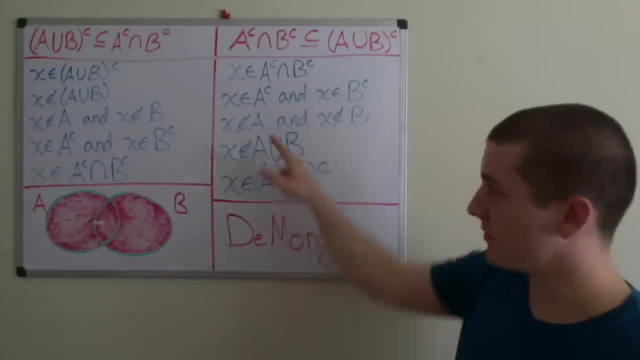 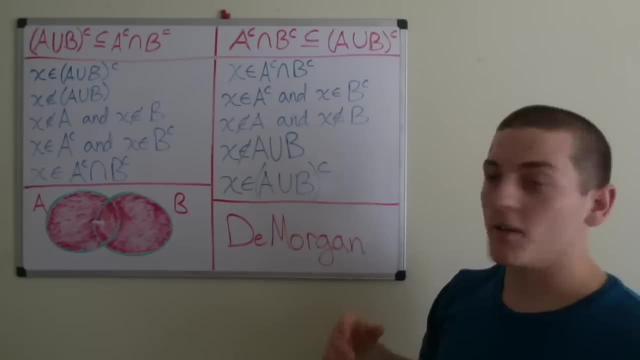 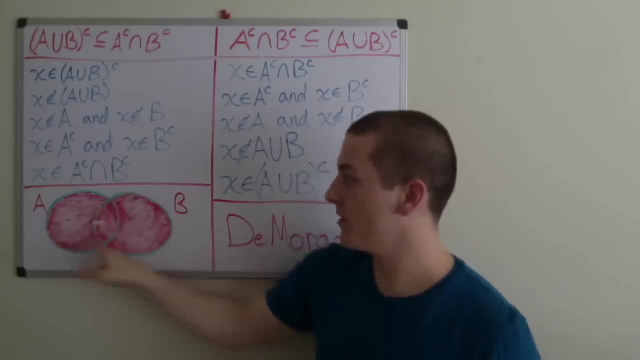 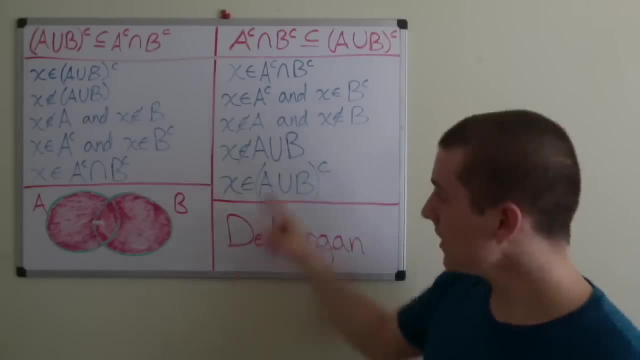 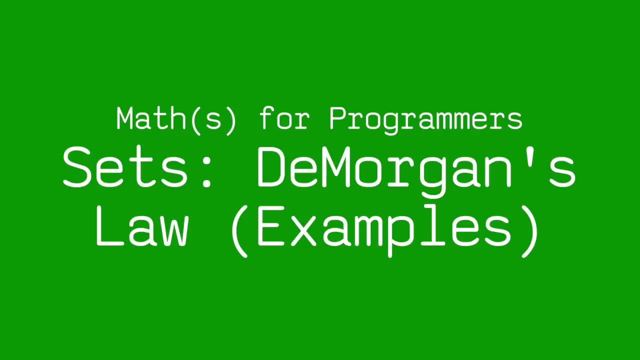 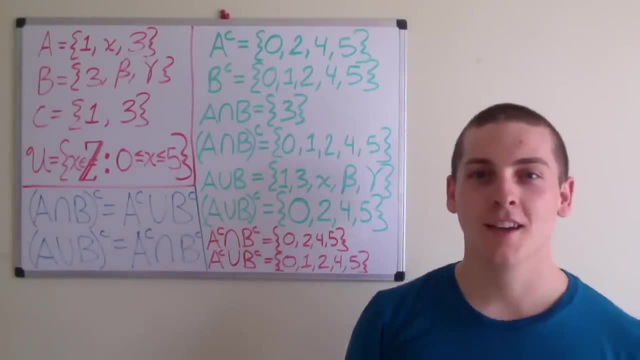 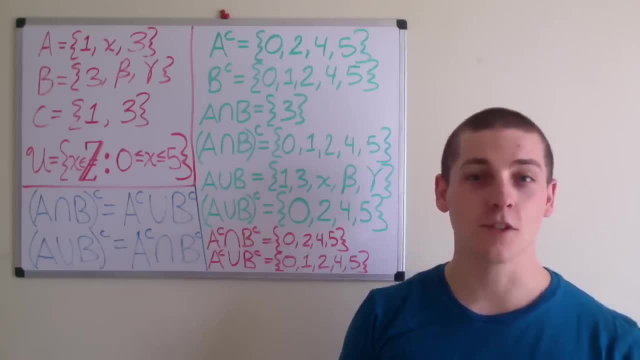 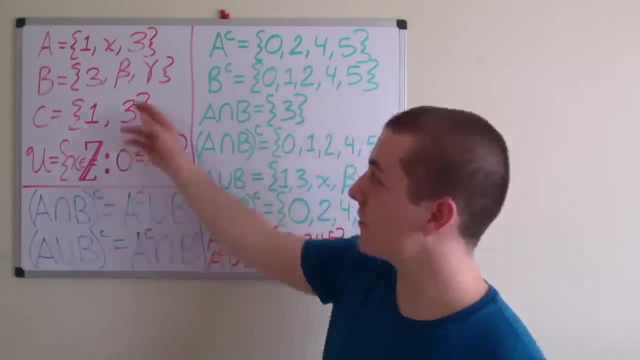 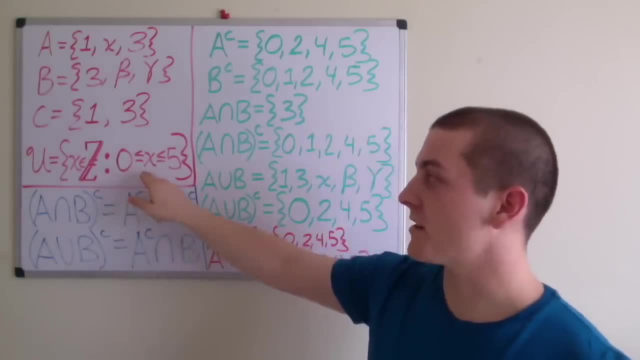 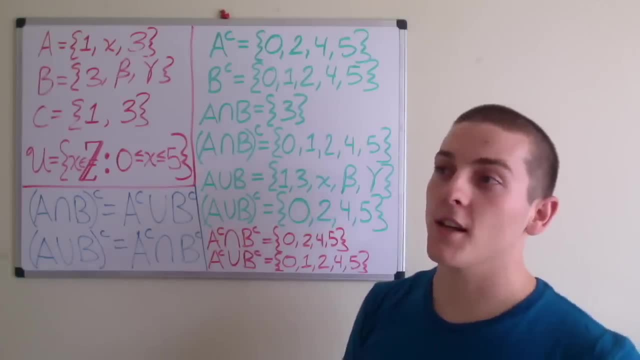 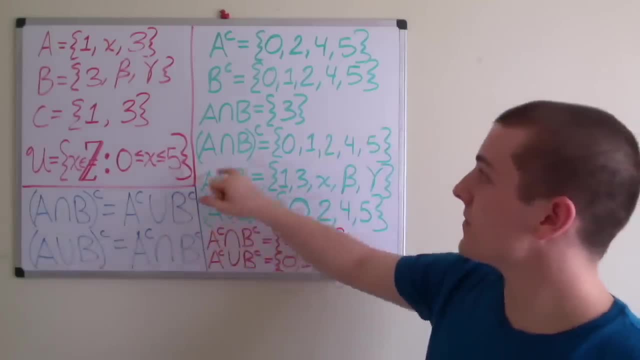 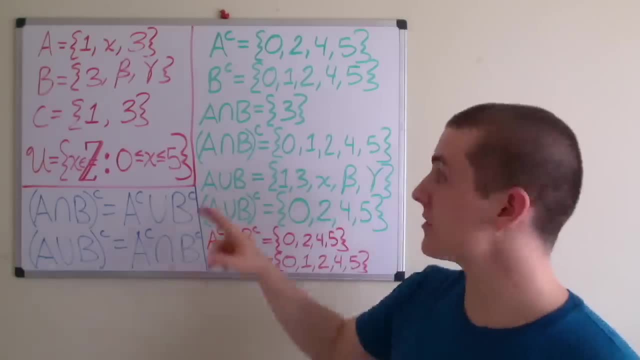 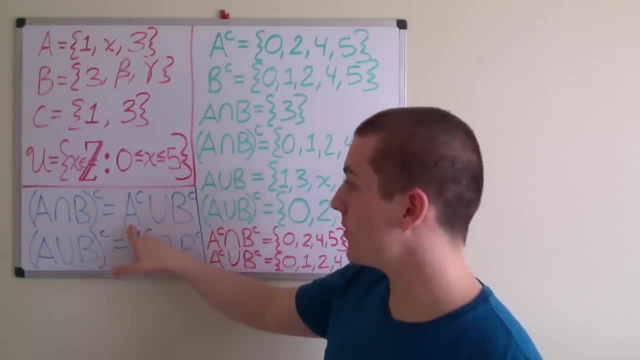 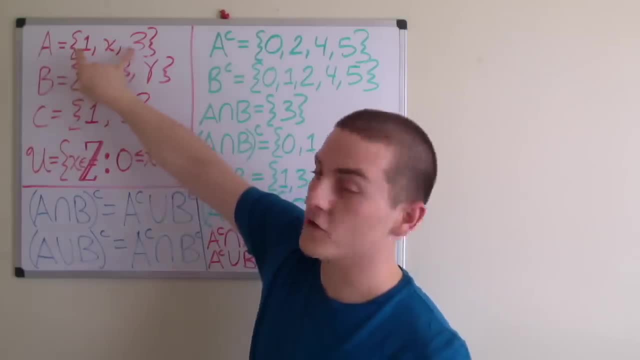 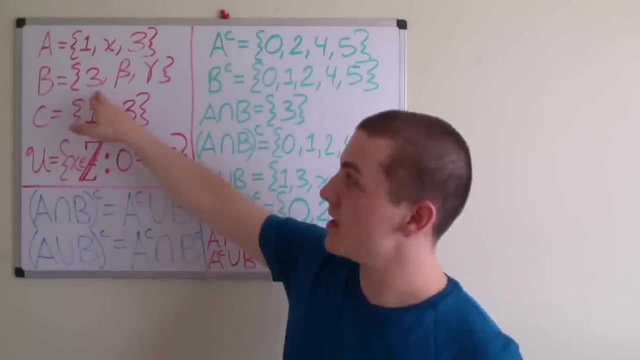 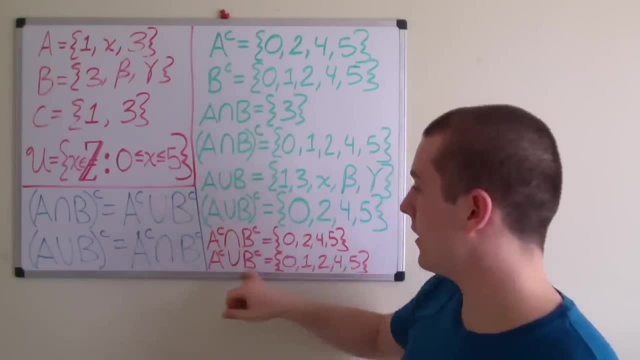 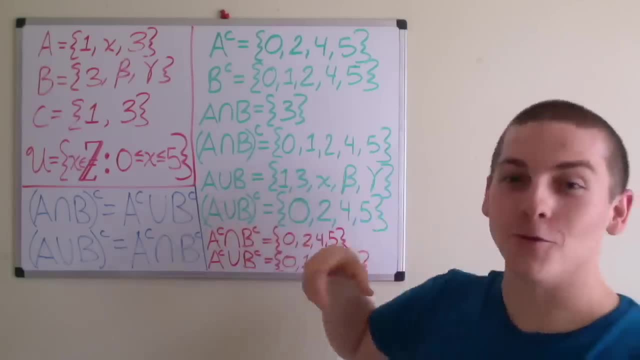 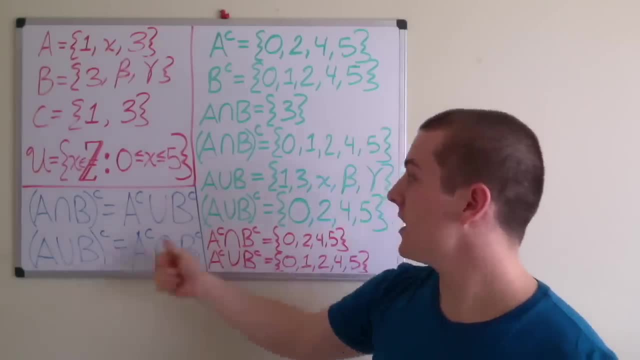 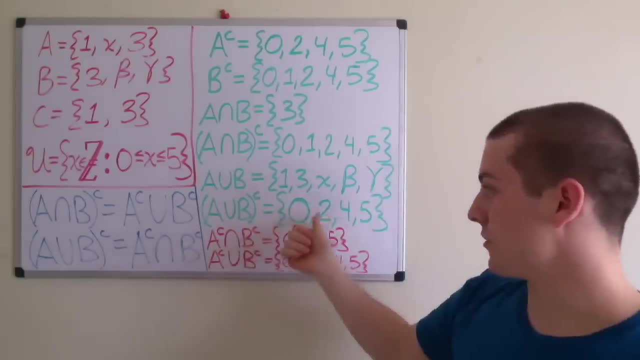 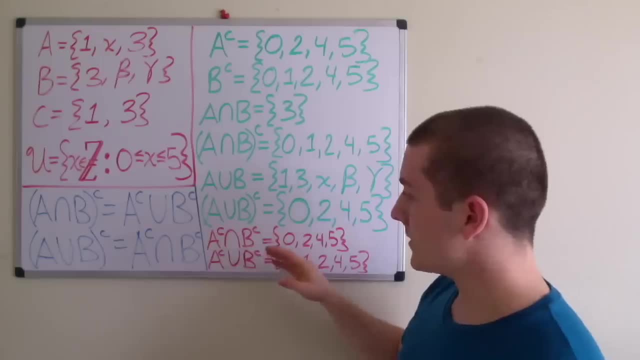 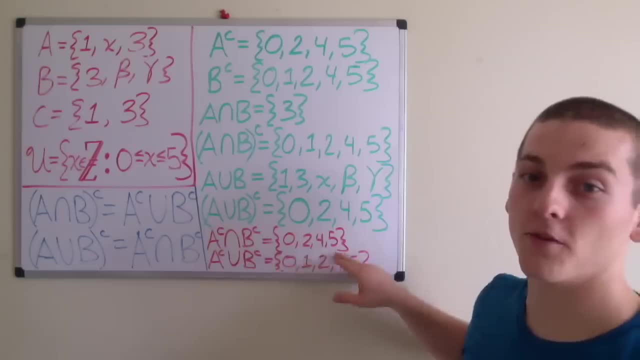 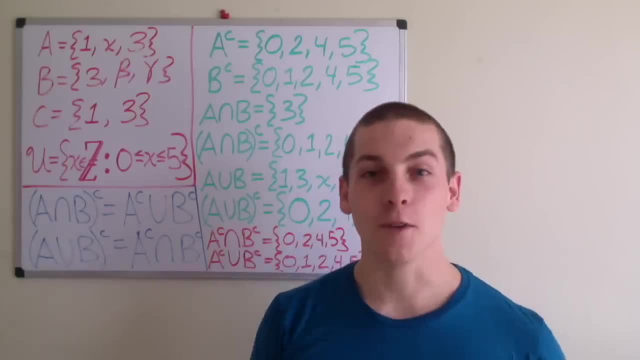 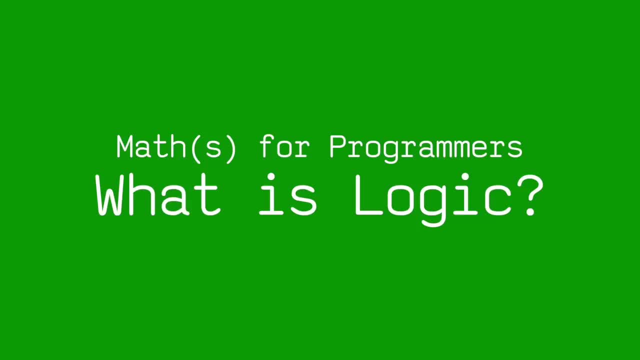 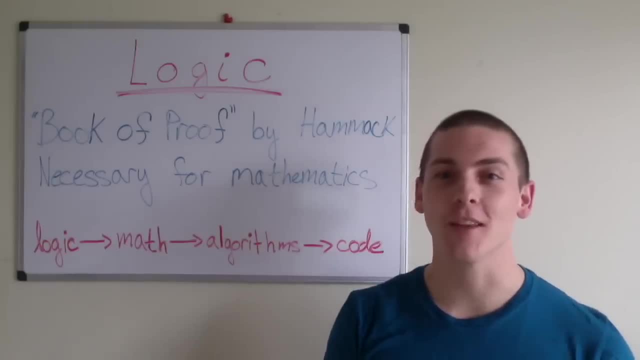 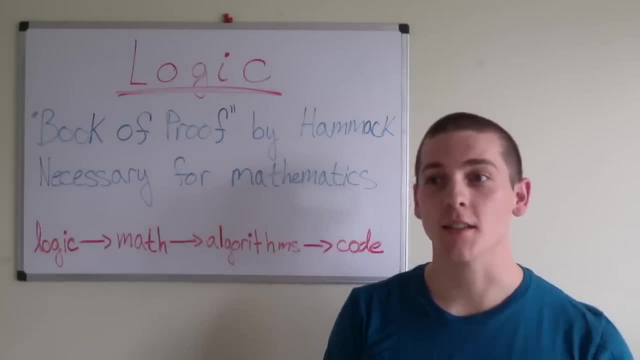 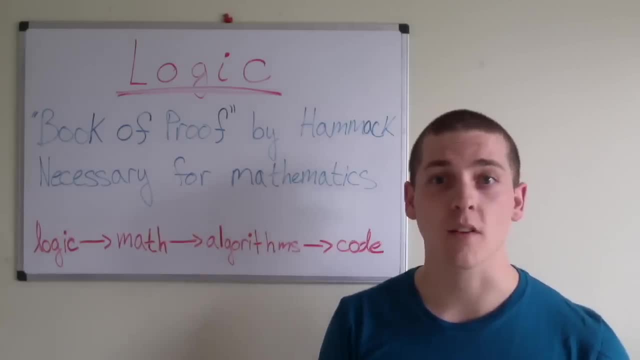 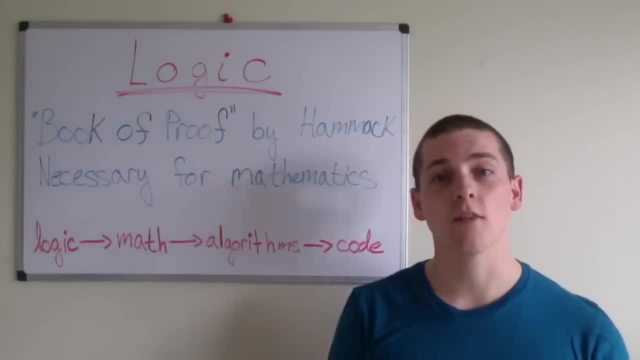 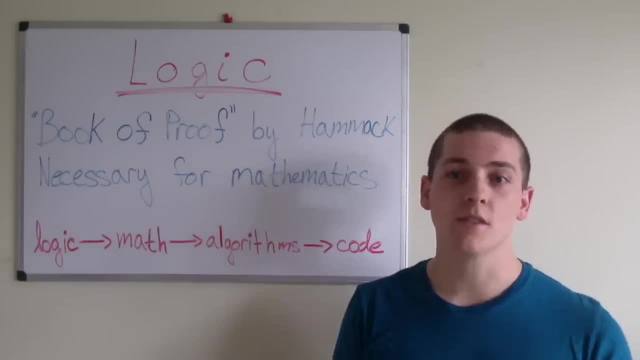 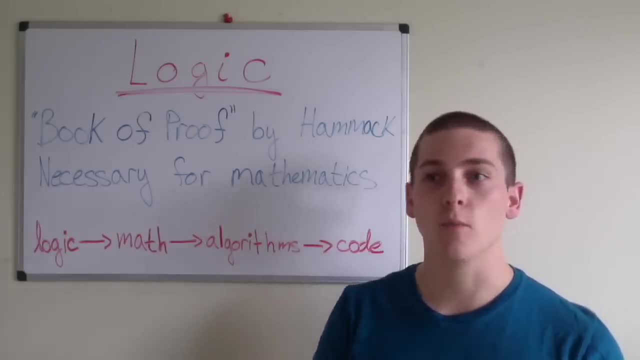 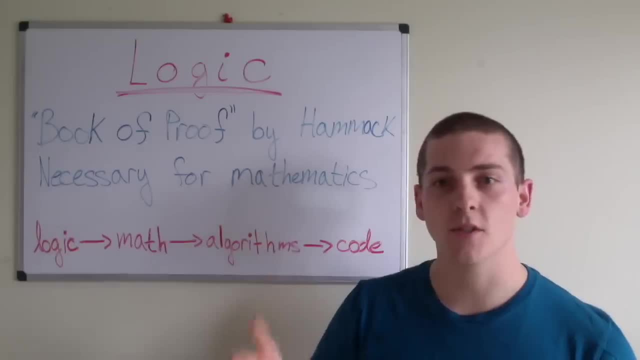 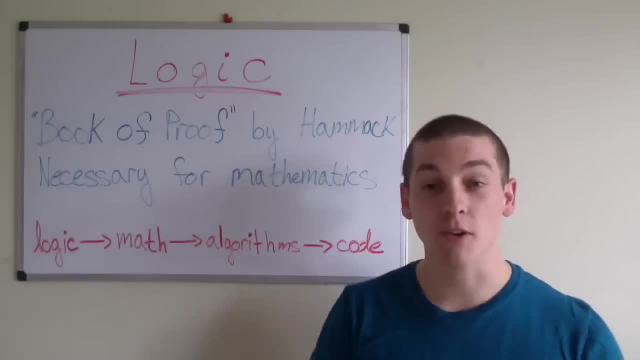 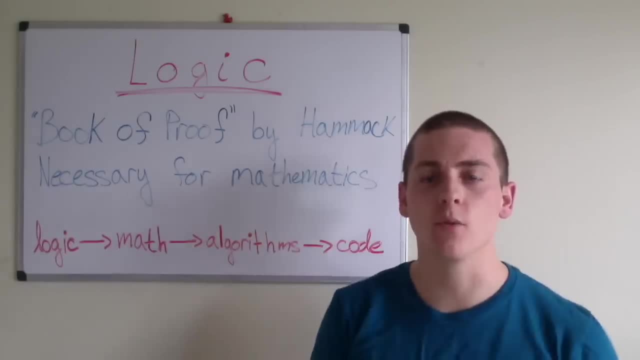 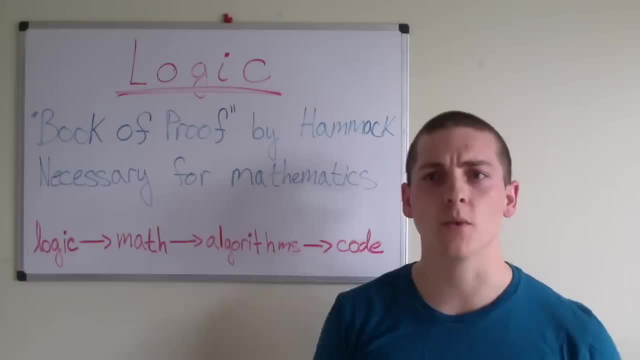 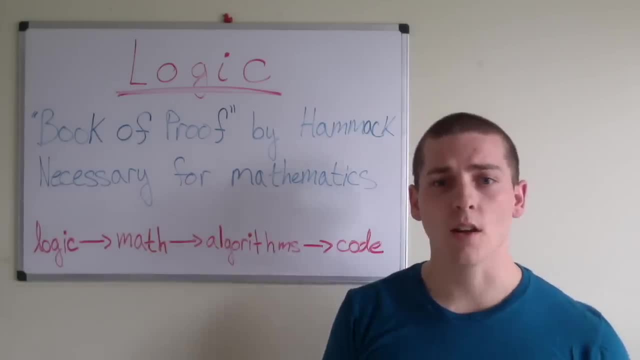 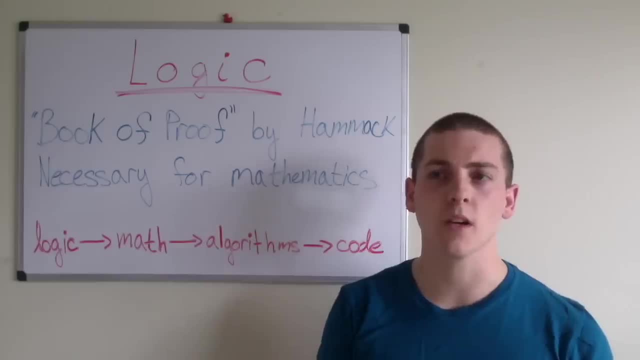 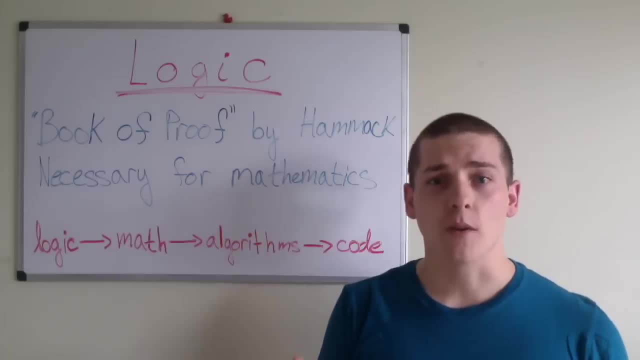 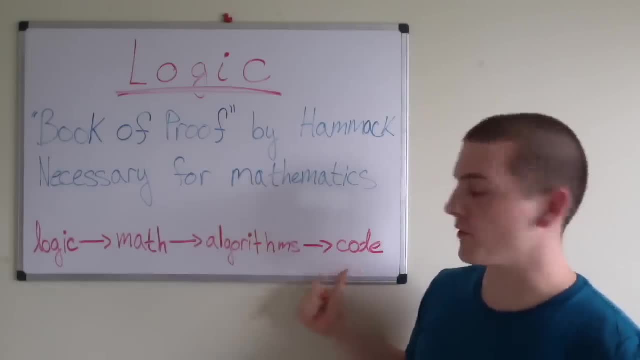 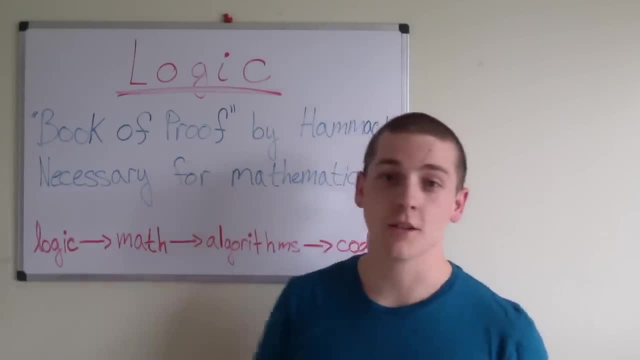 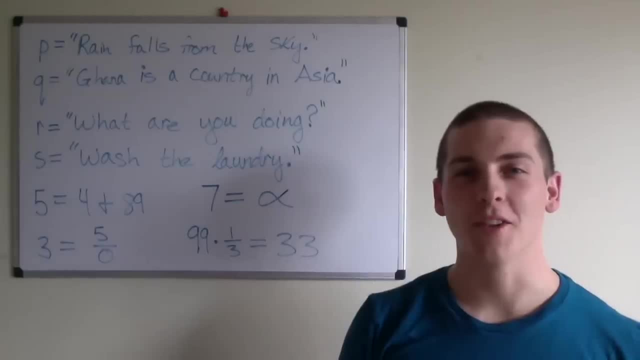 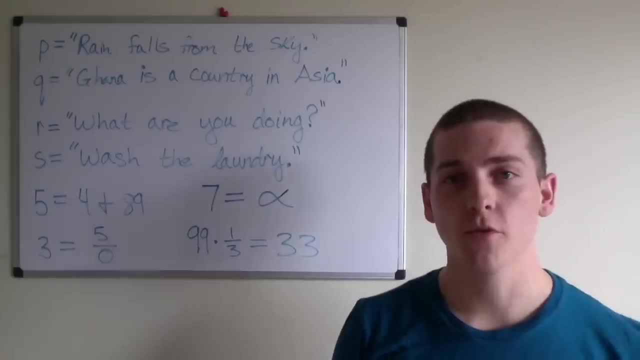 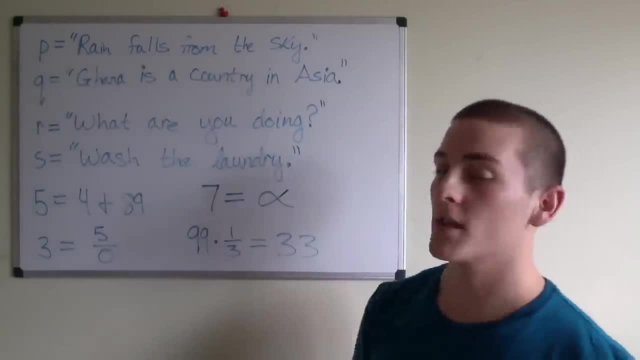 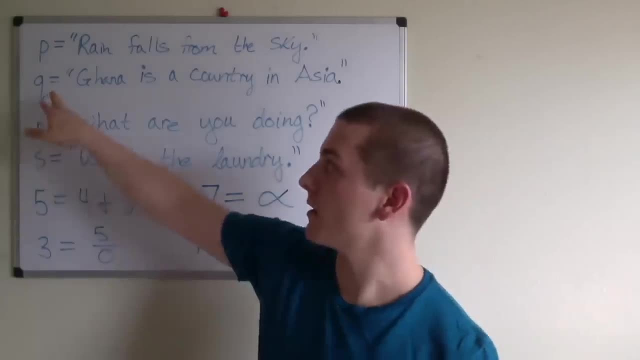 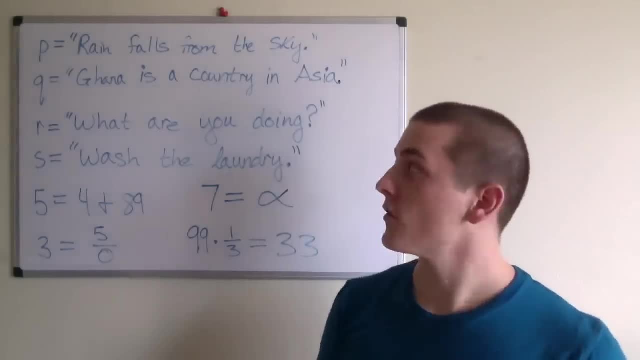 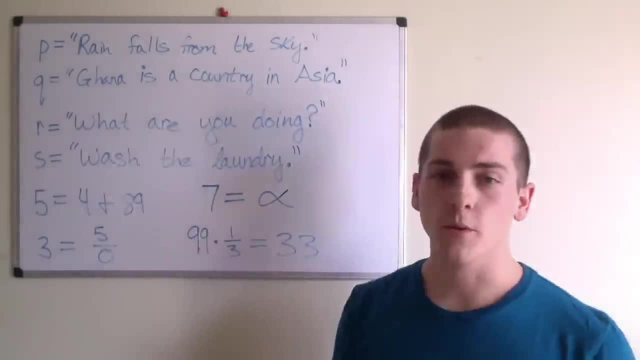 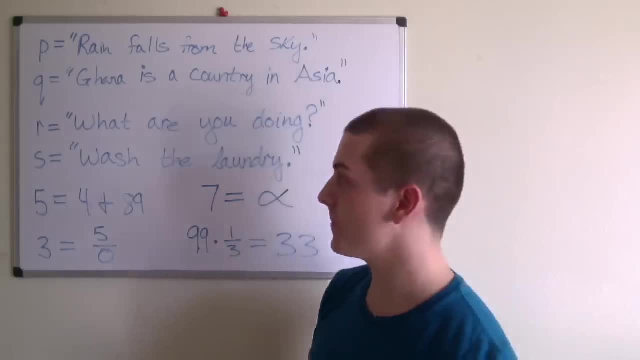 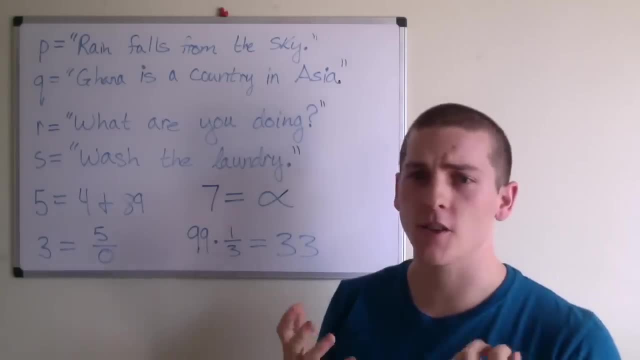 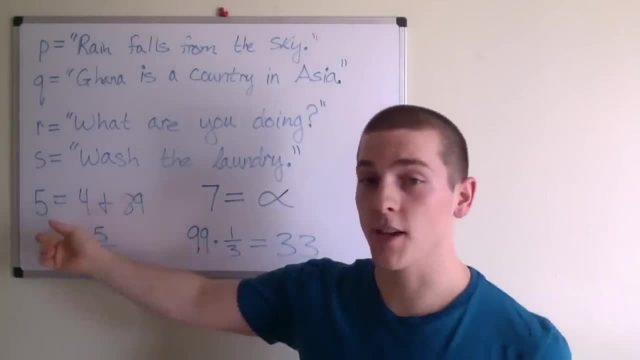 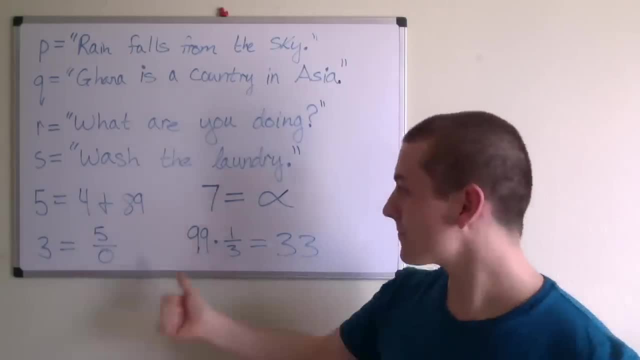 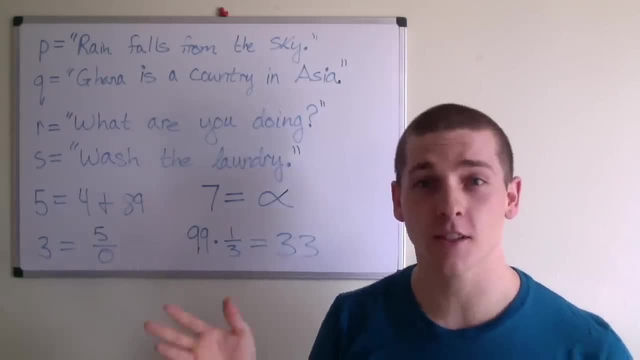 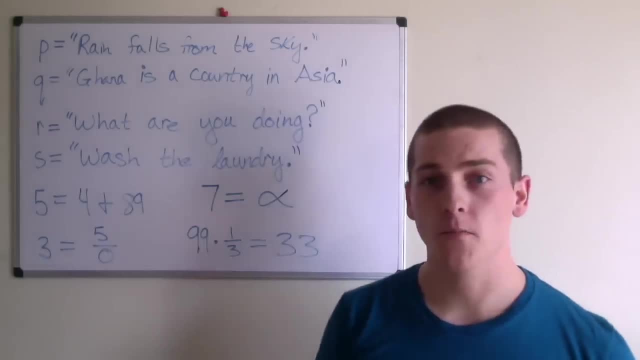 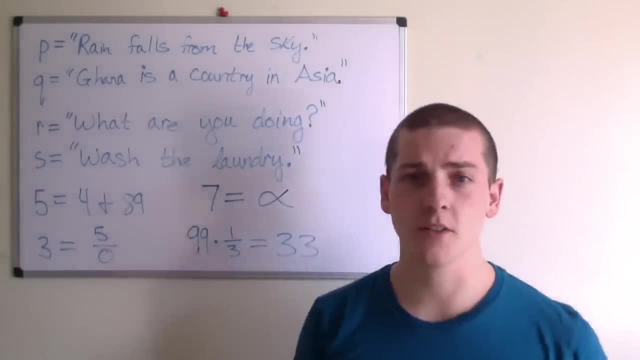 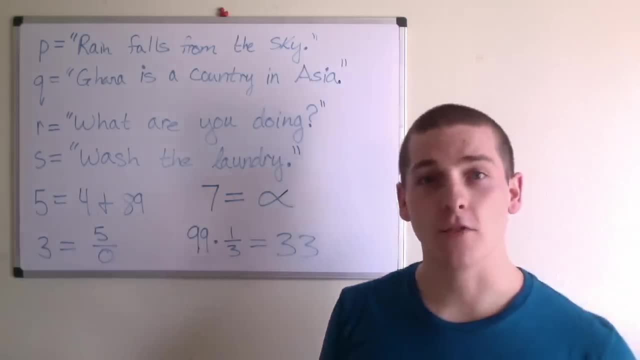 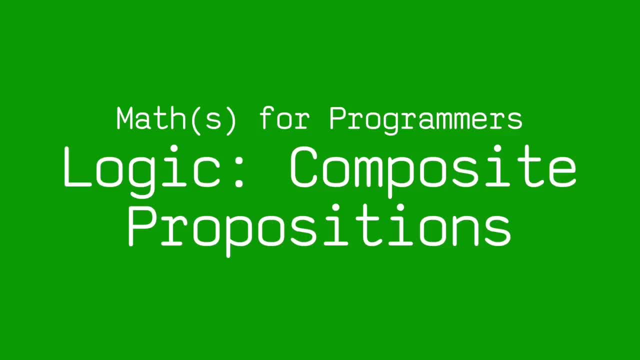 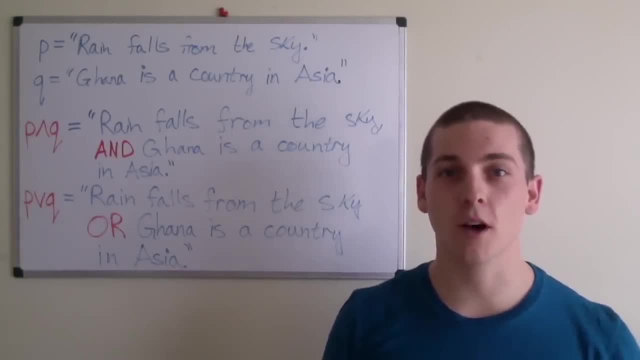 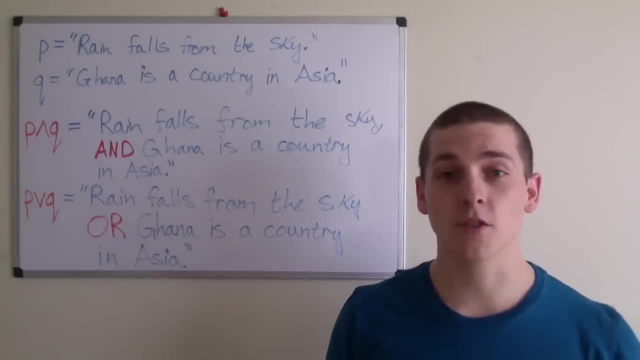 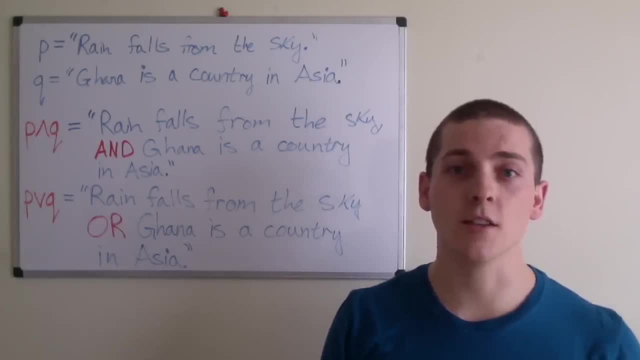 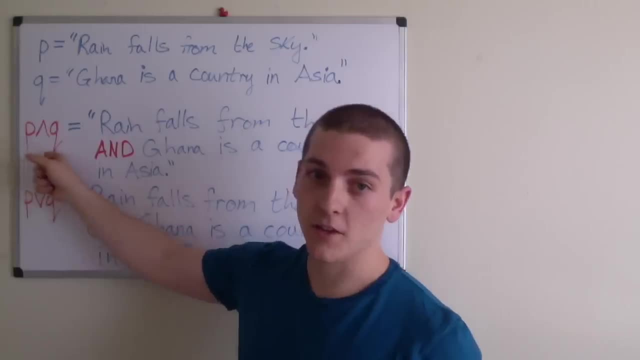 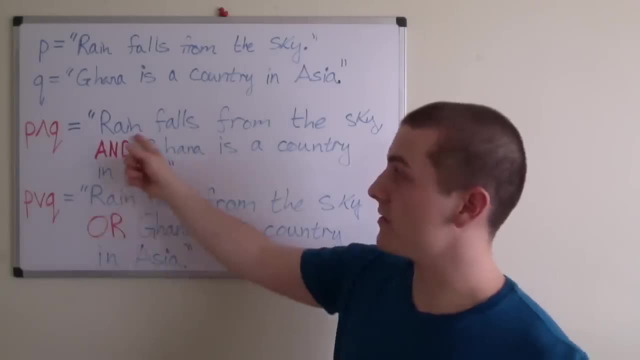 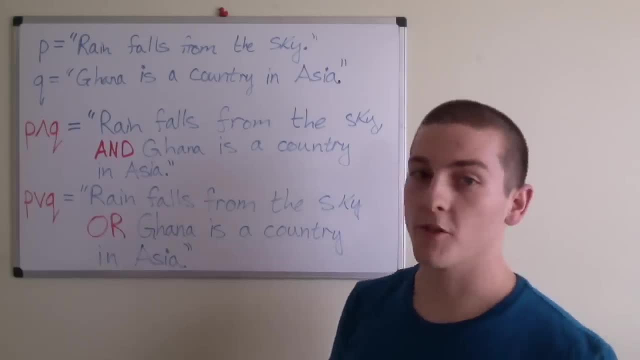 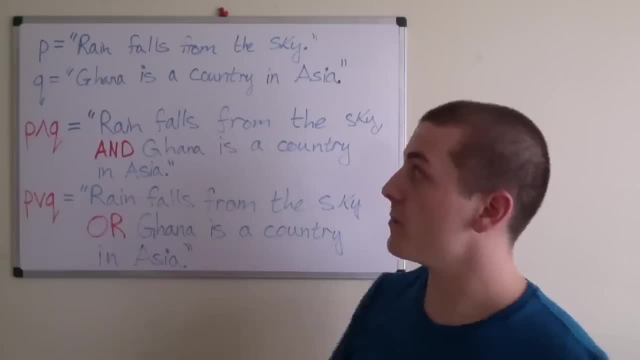 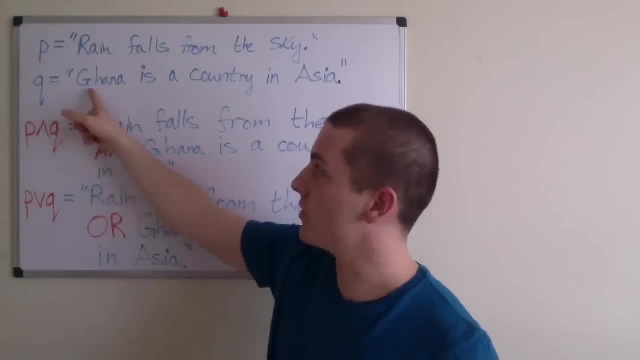 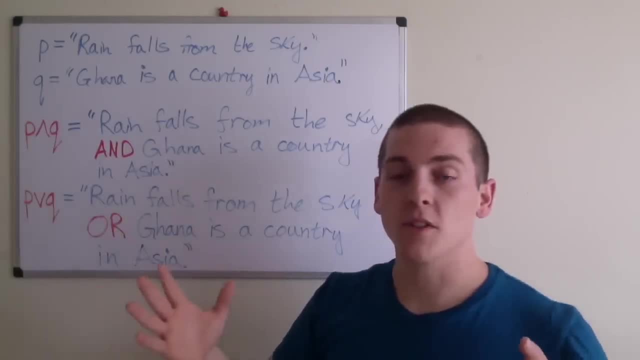 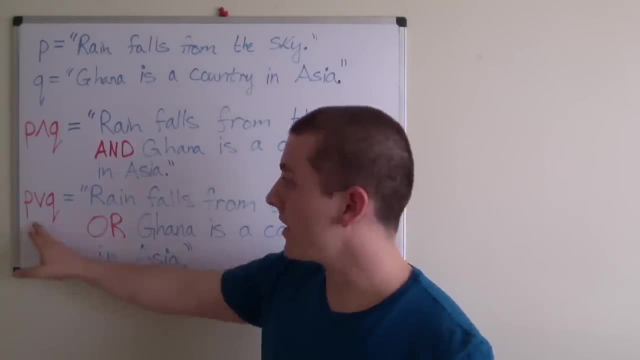 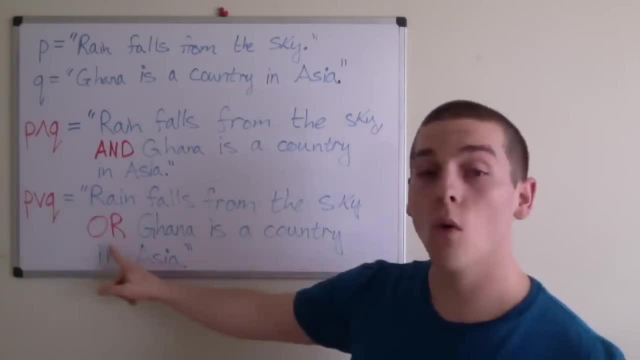 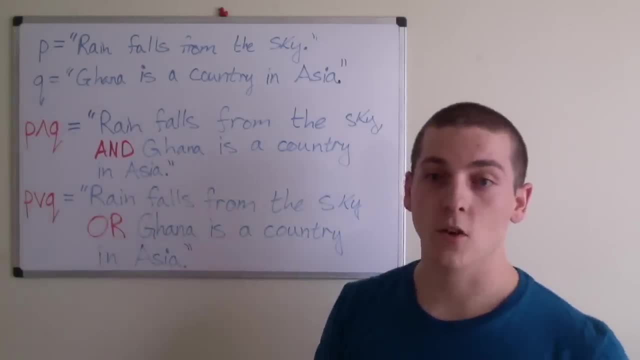 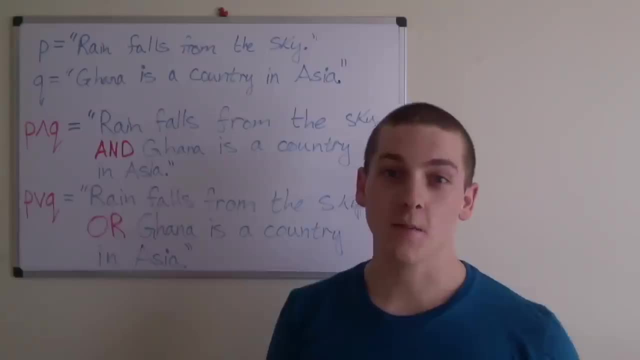 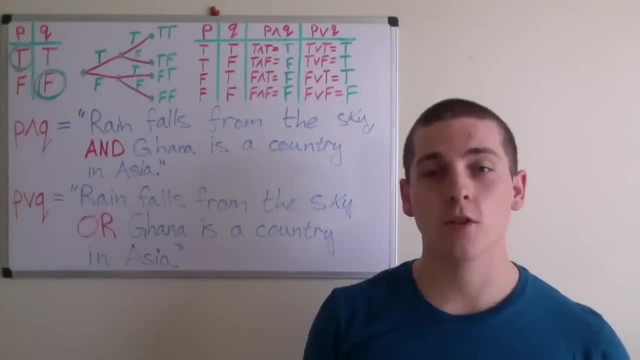 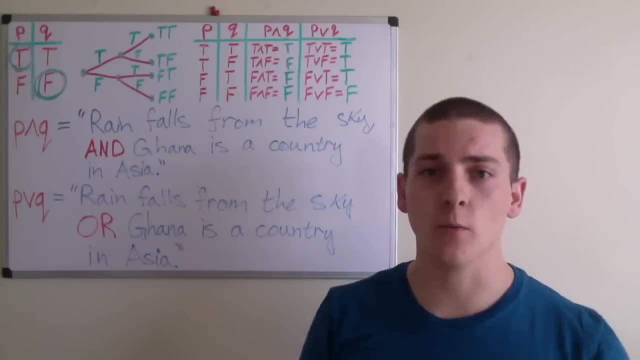 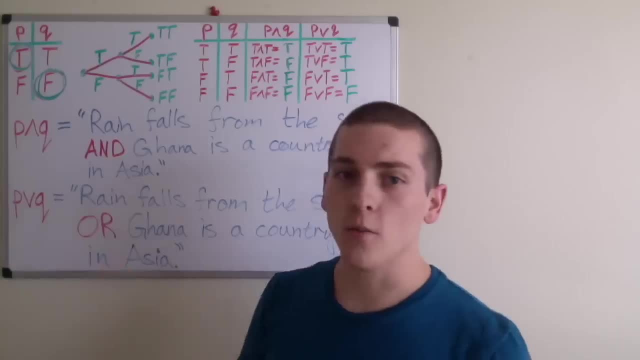 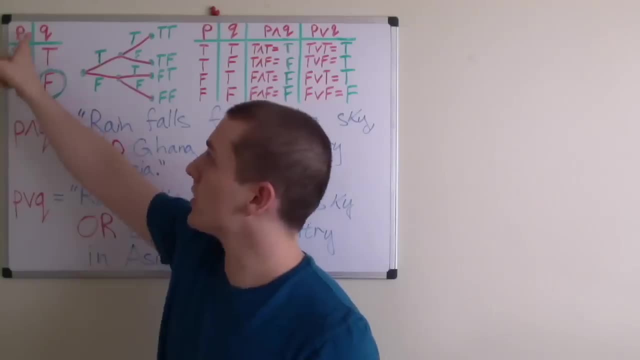 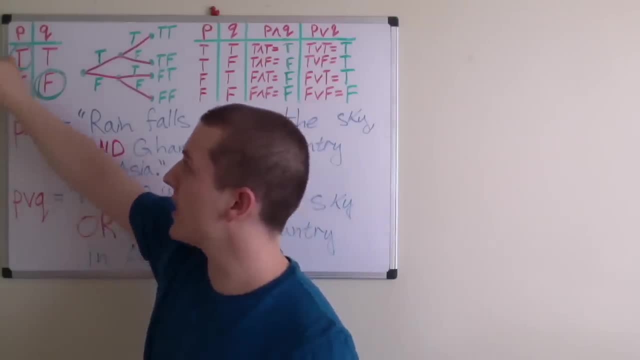 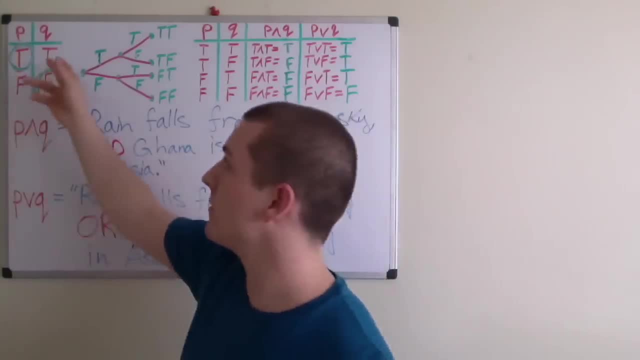 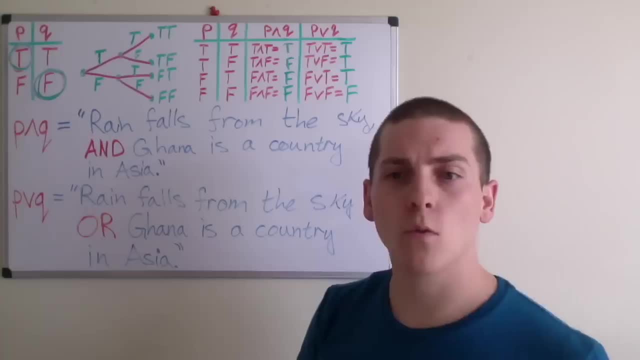 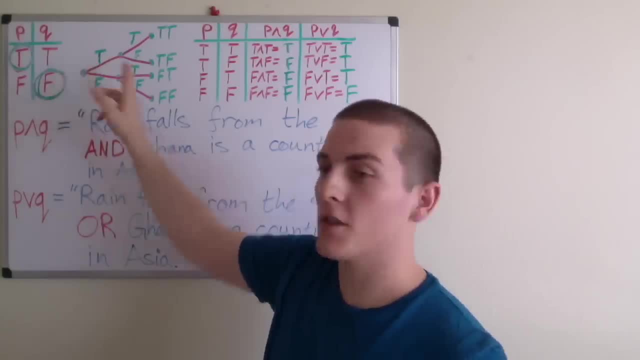 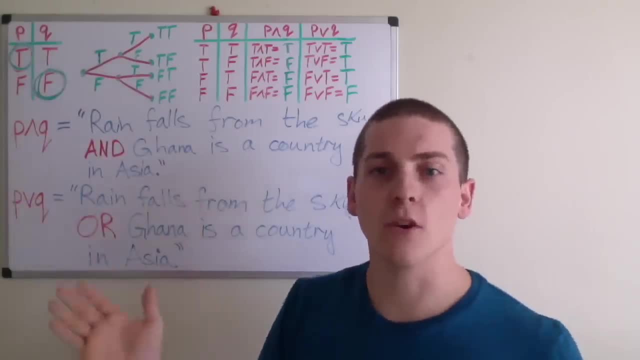 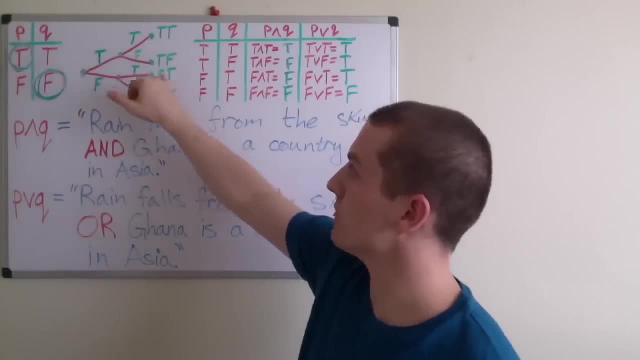 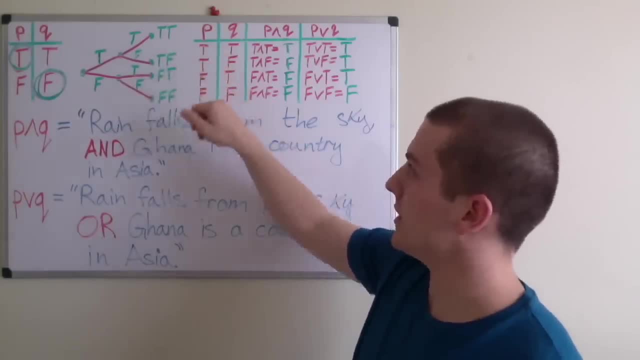 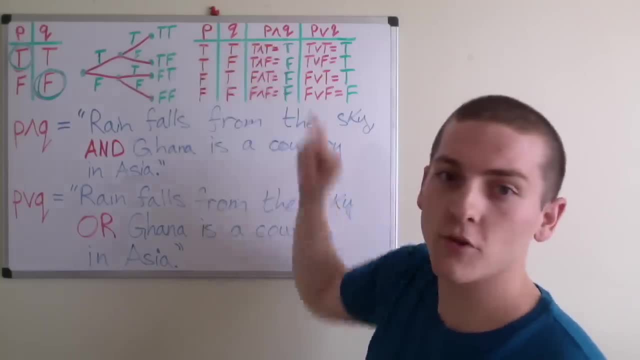 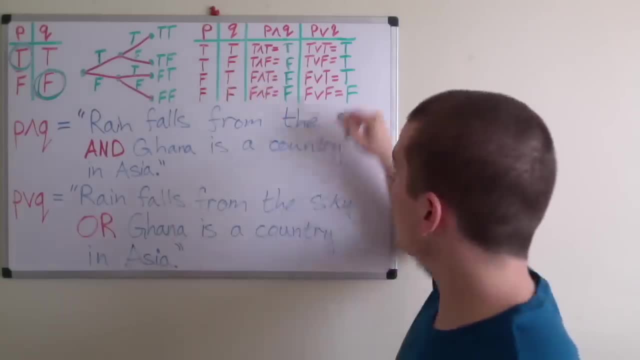 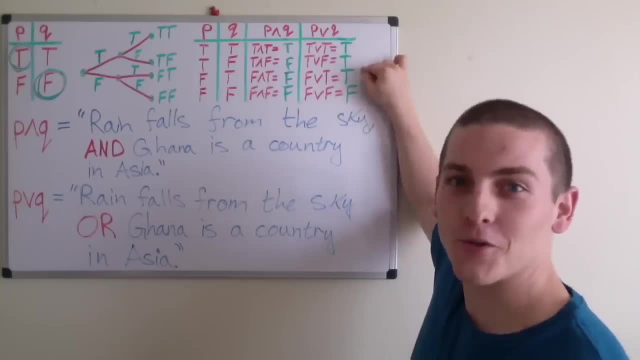 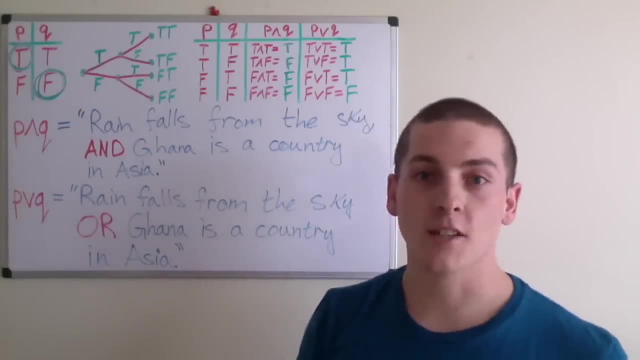 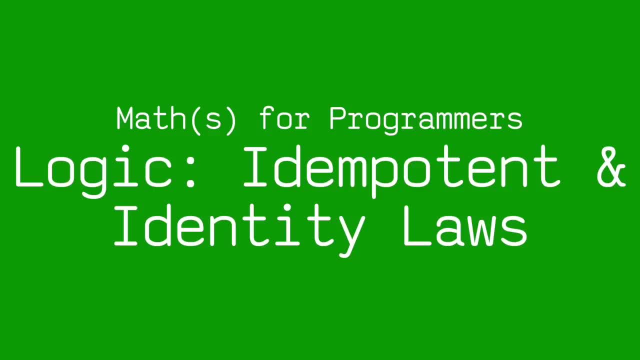 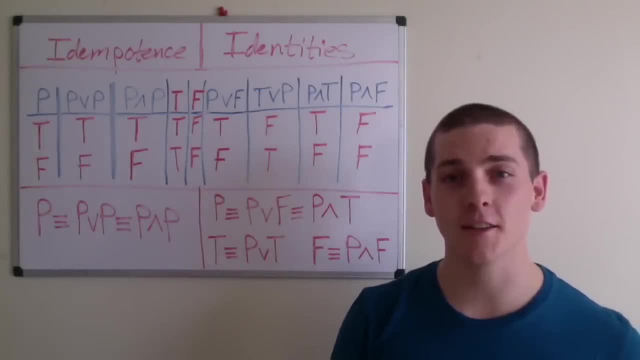 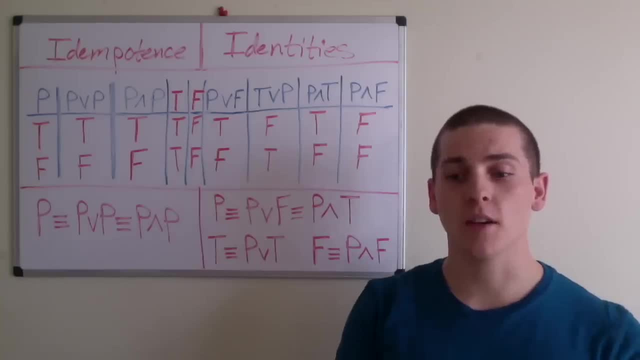 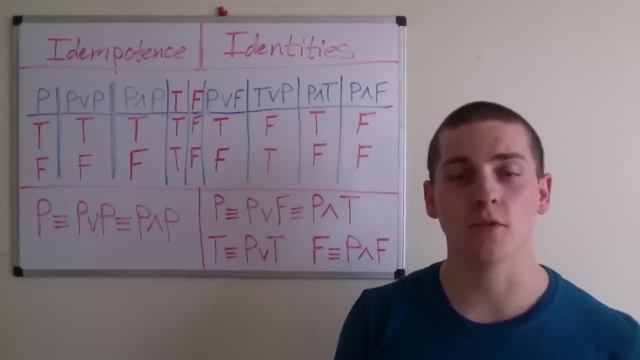 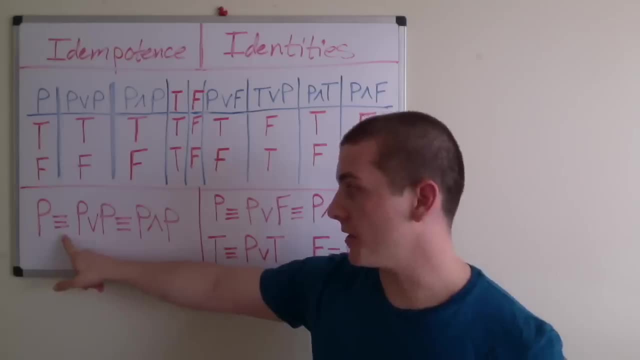 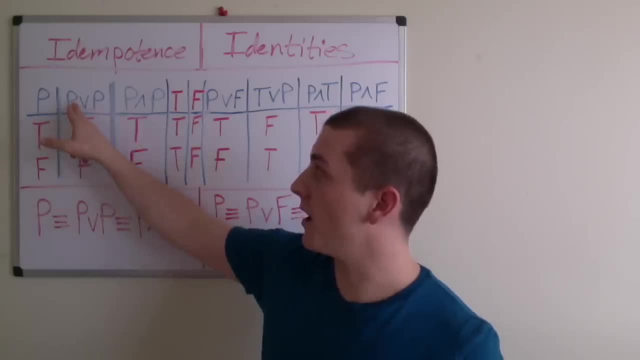 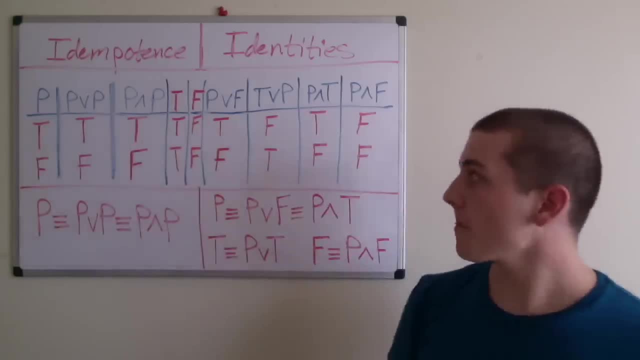 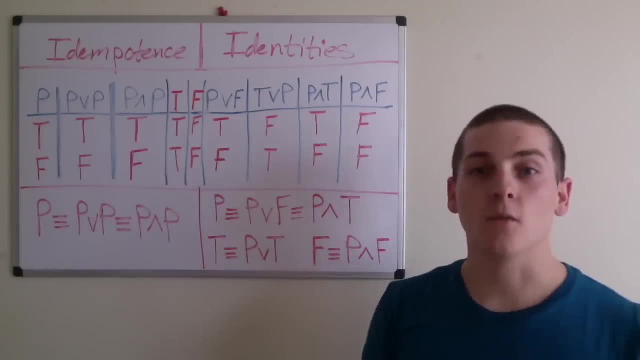 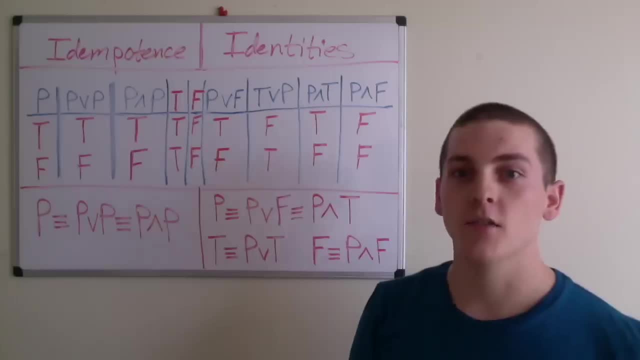 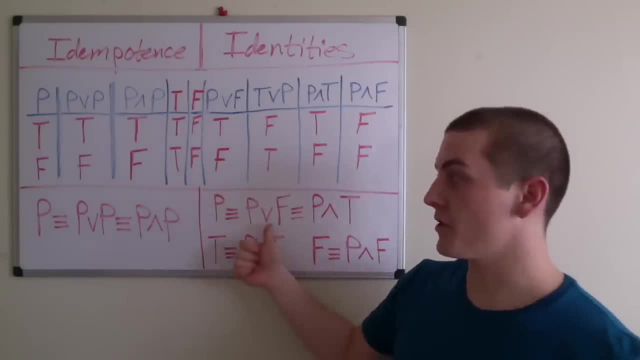 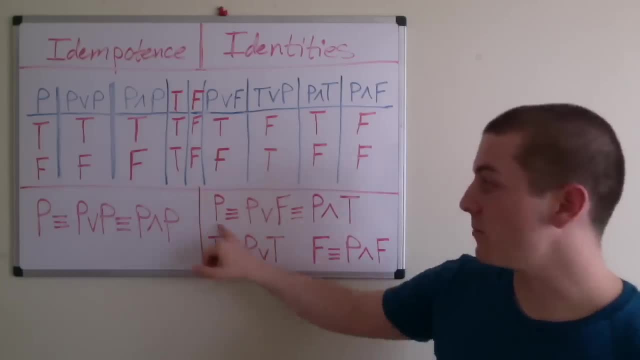 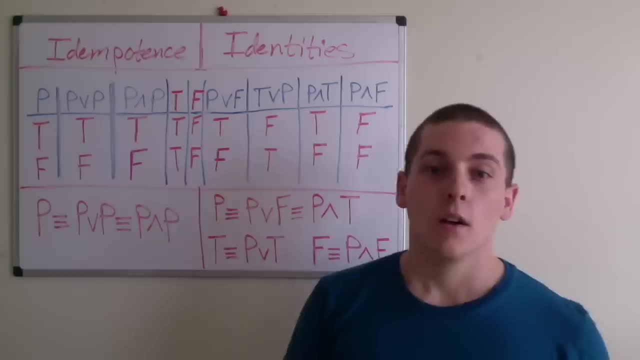 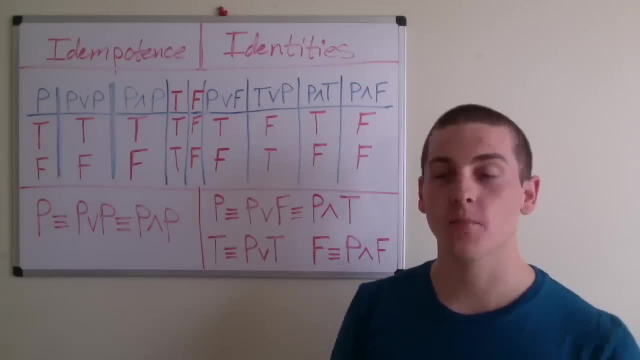 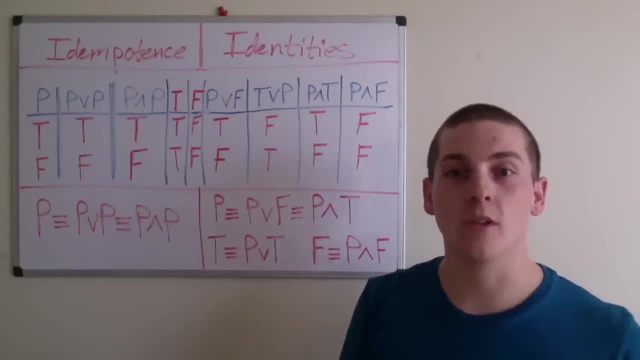 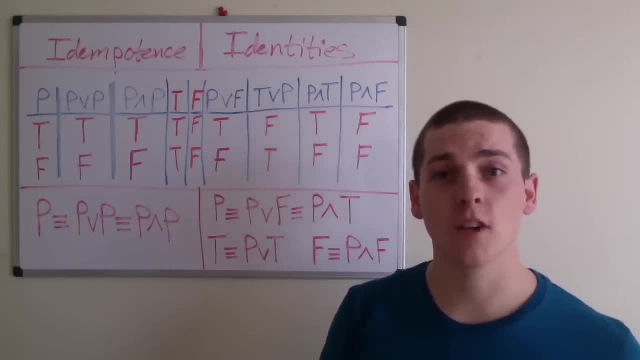 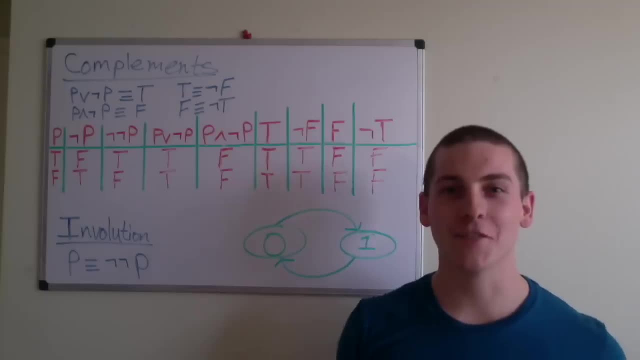 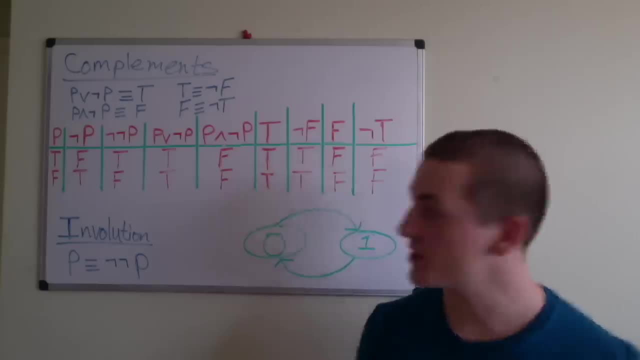 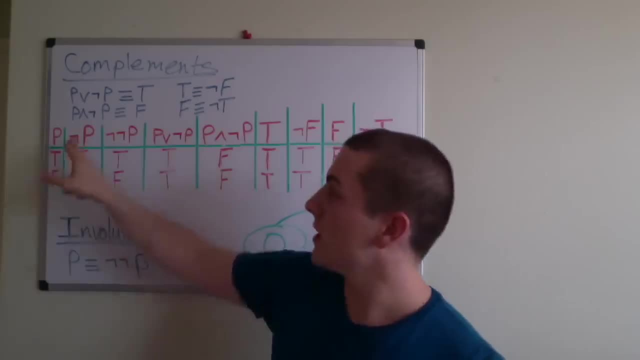 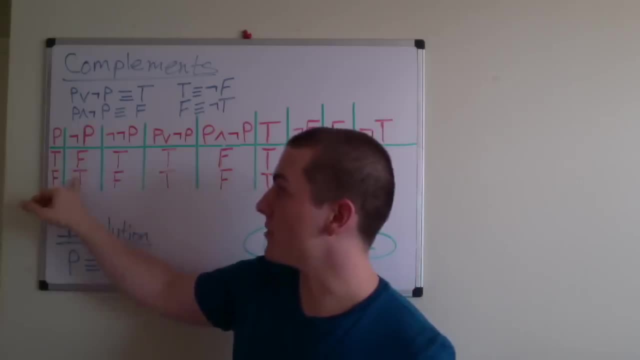 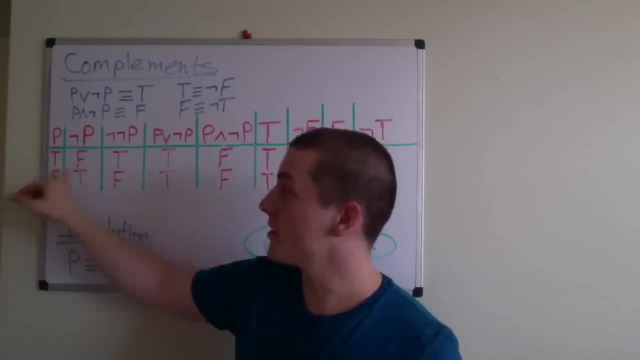 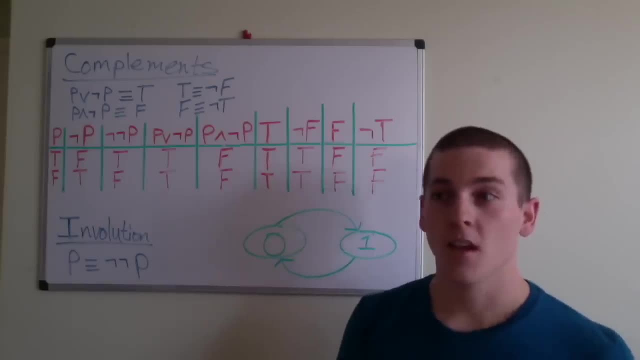 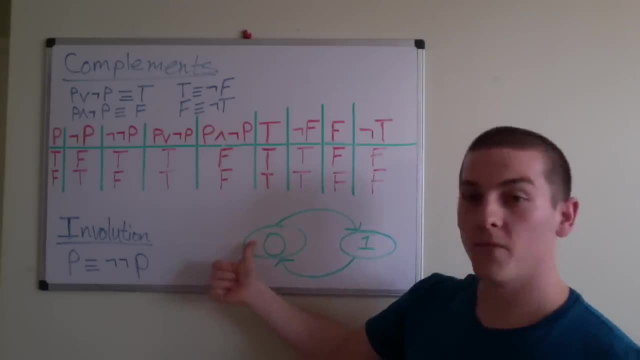 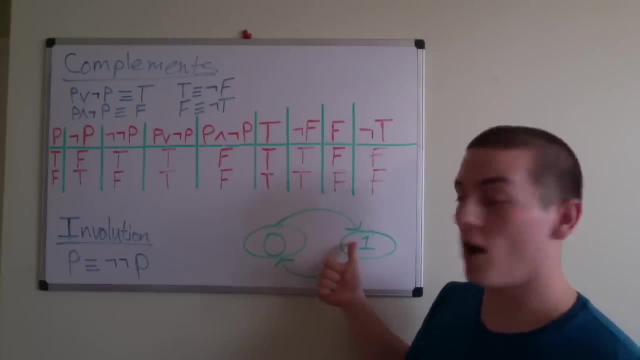 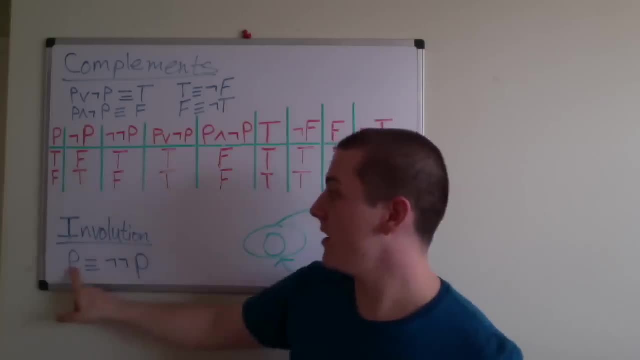 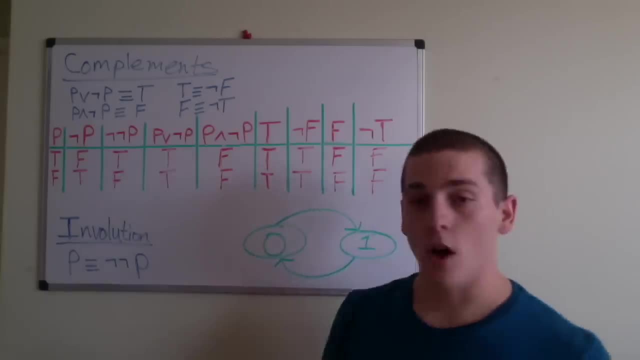 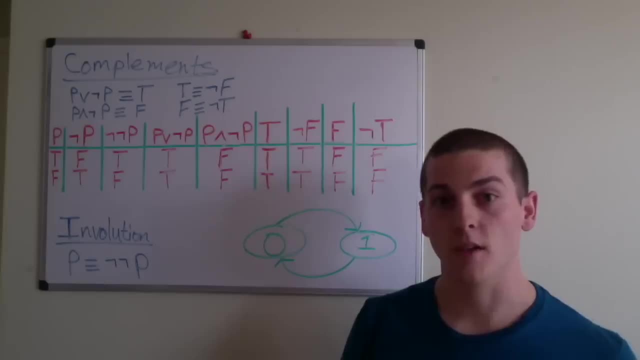 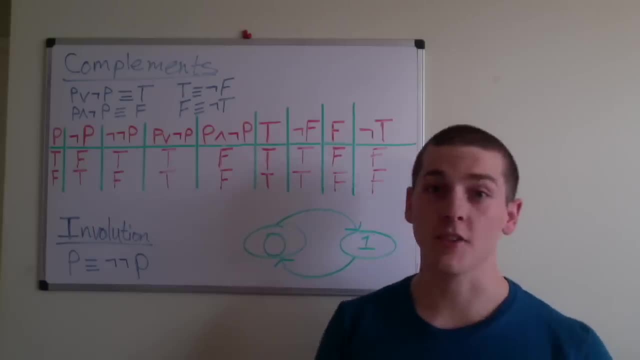 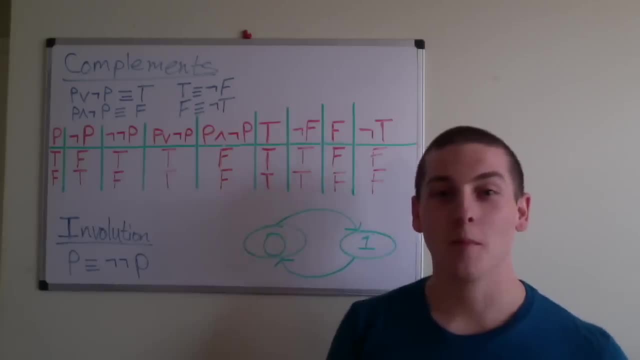 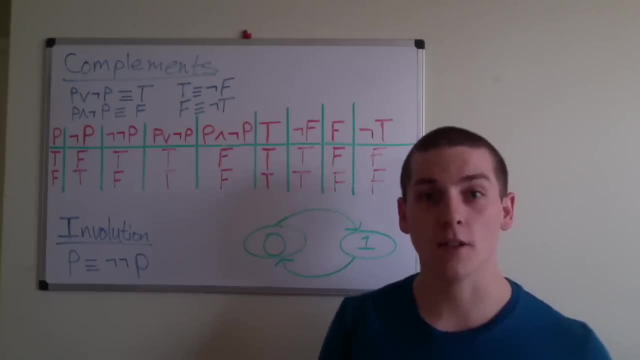 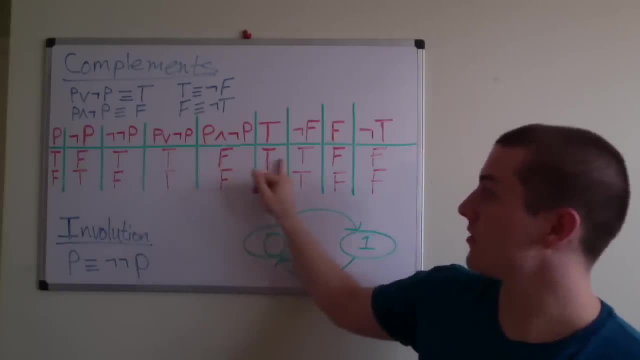 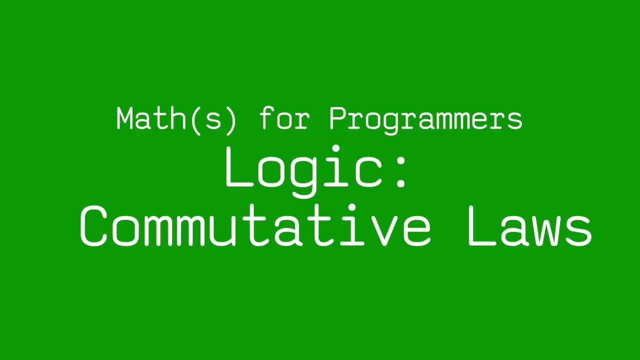 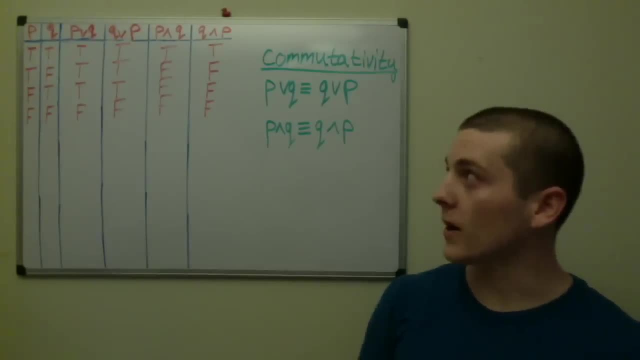 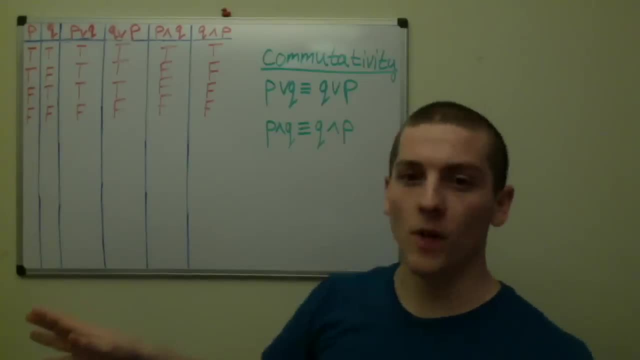 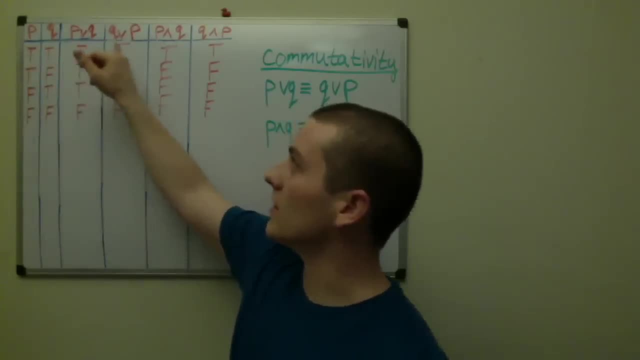 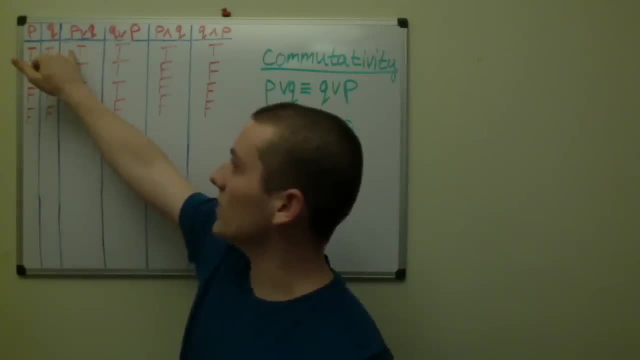 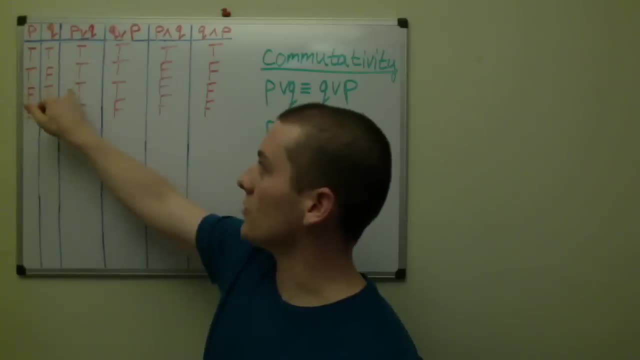 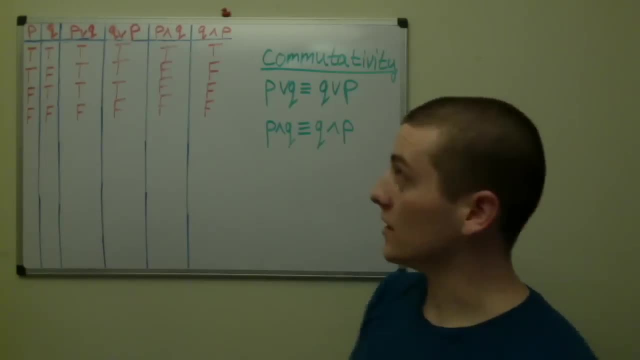 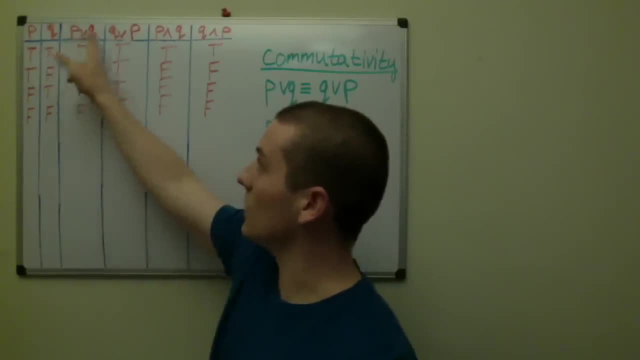 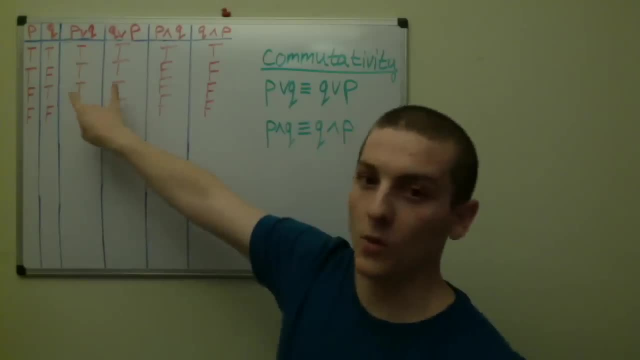 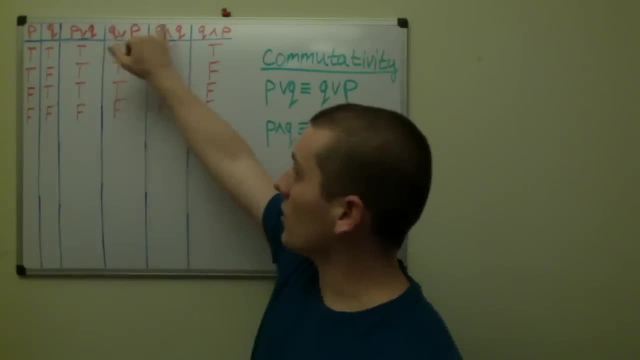 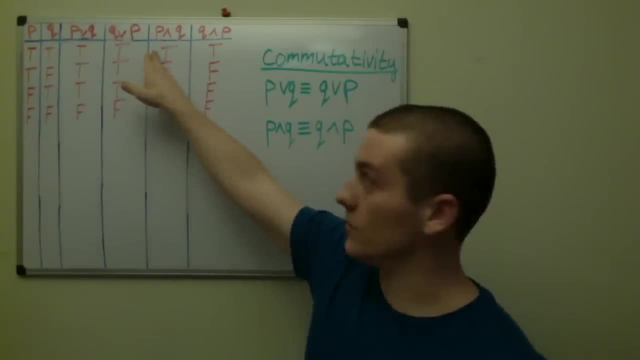 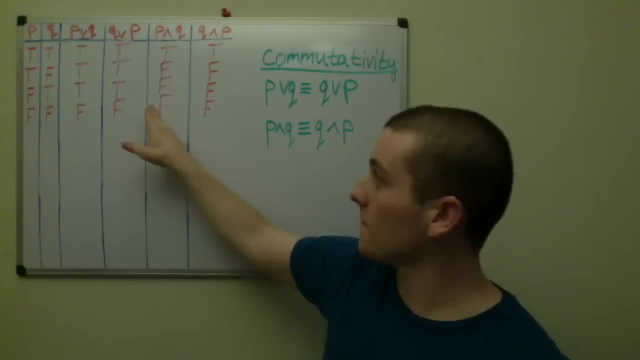 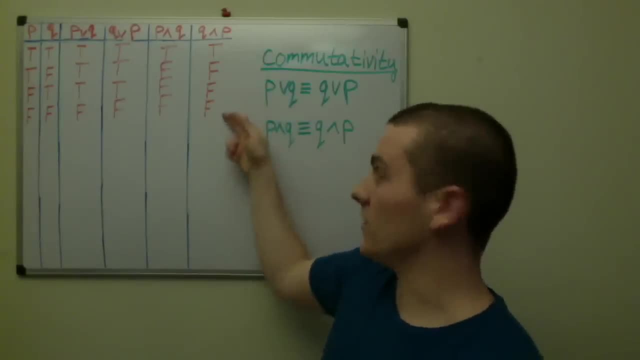 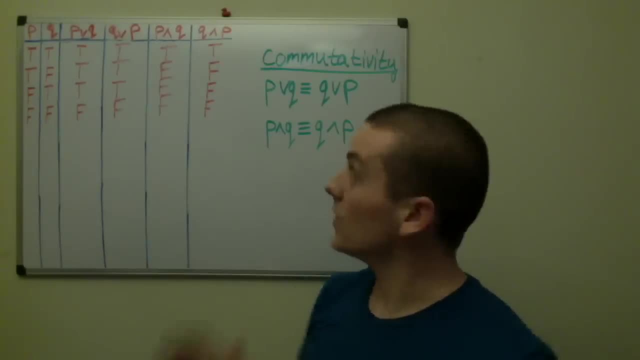 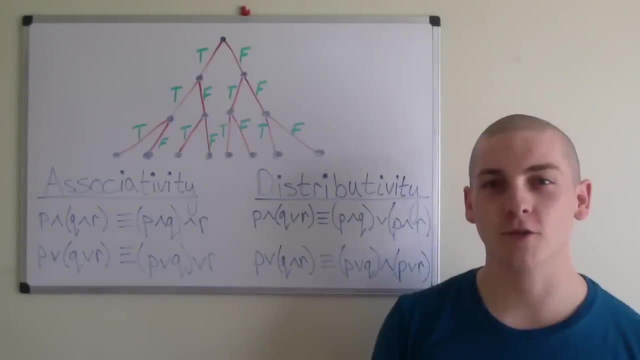 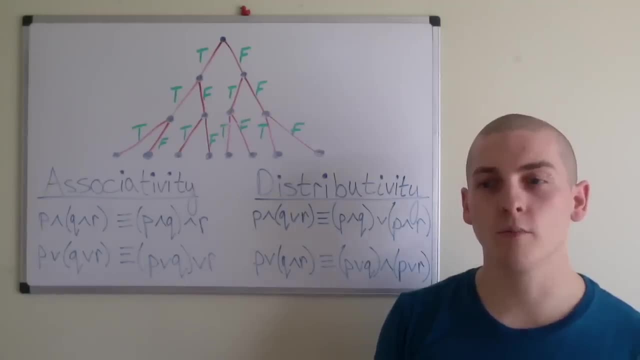 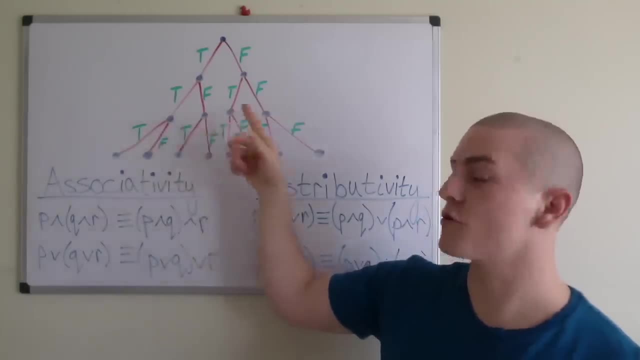 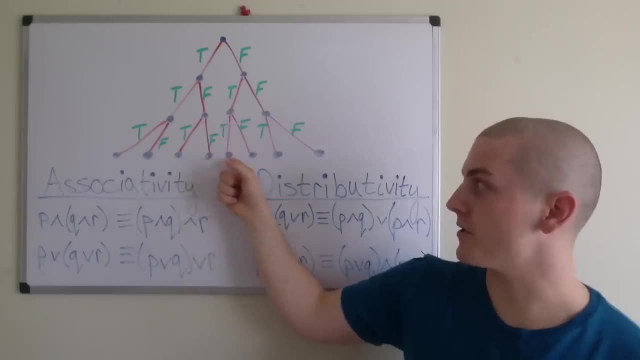 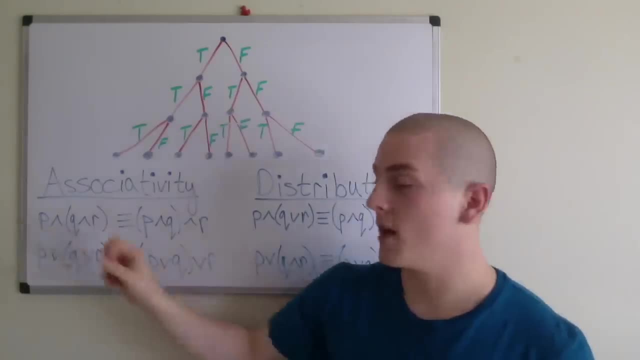 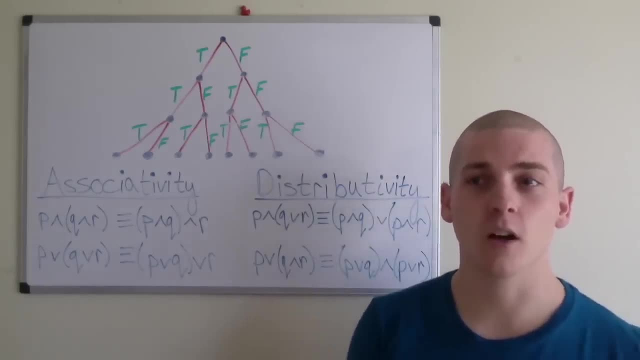 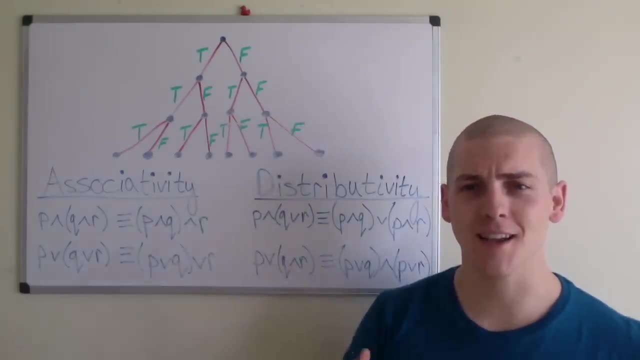 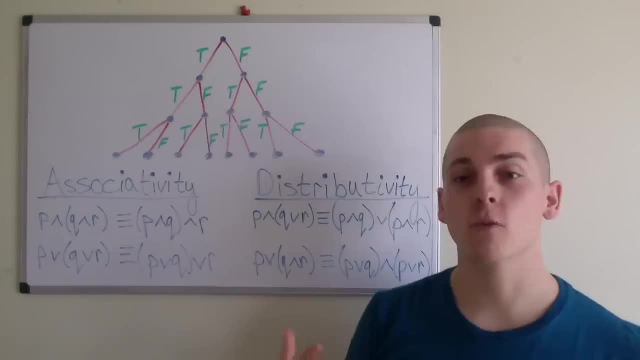 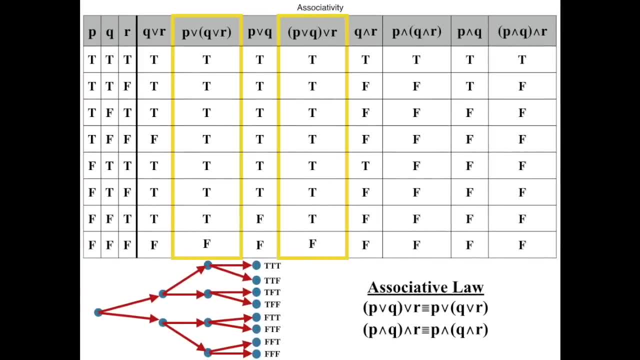 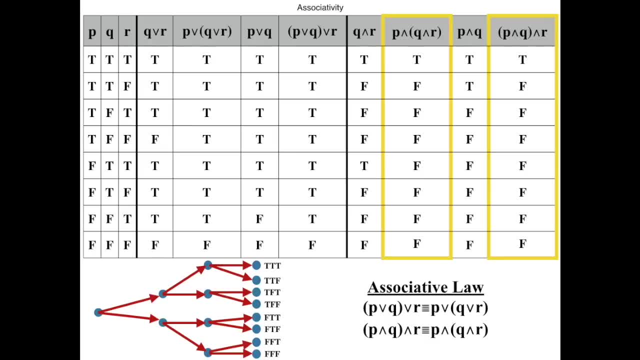 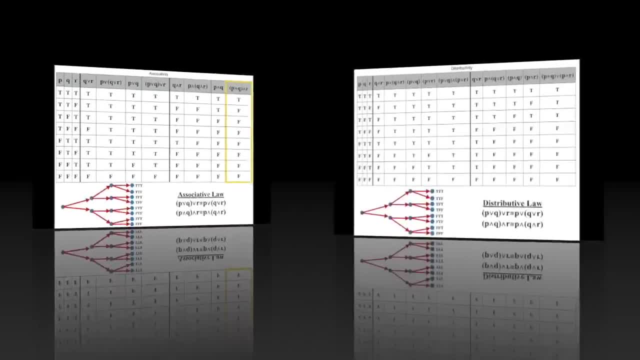 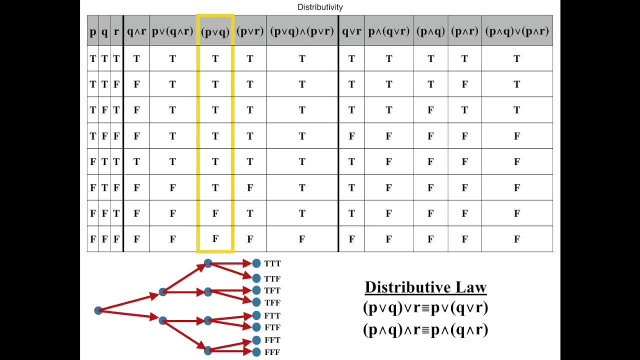 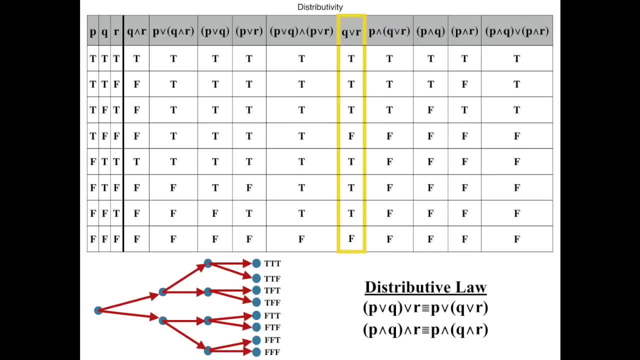 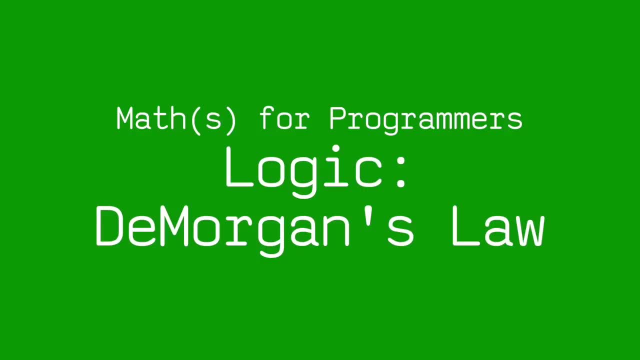 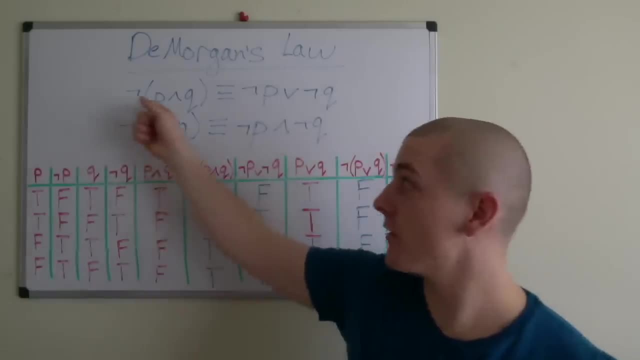 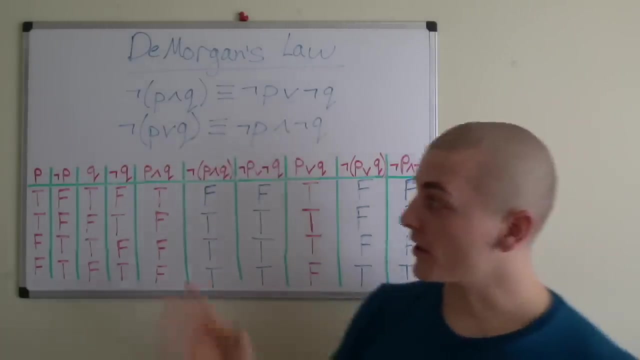 law- De Morgan's law- states that the negation of the conjunction is the logical equivalent of the disjunction of the negations and also that the negation of the disjunction is the logical equivalent of the conjunction of the negations. So if we look at our truth table, I've decomposed our propositions. 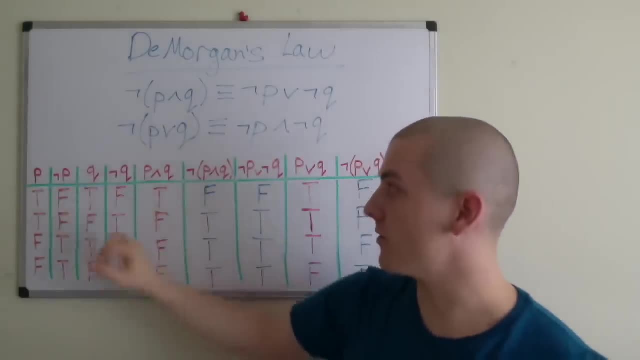 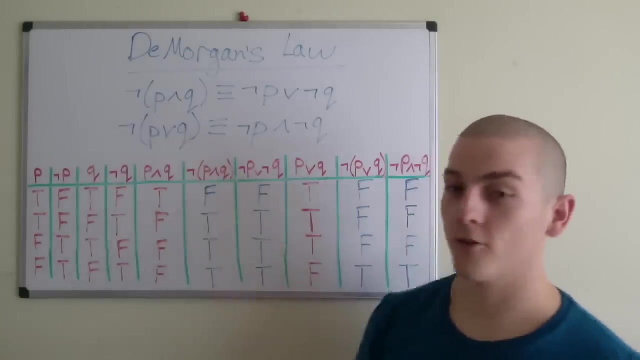 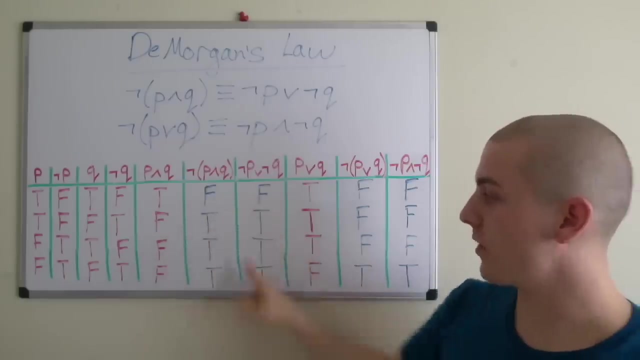 here, so that we have P, NOT P, Q, NOT Q, and I have it all out on the board, so that I can just simply look at NOT P and Q, which is our first law, and see that it is in fact equivalent to NOT P or NOT Q. So these two columns are equal, so we can. 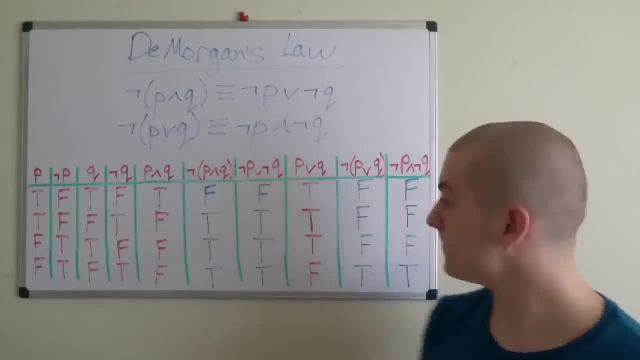 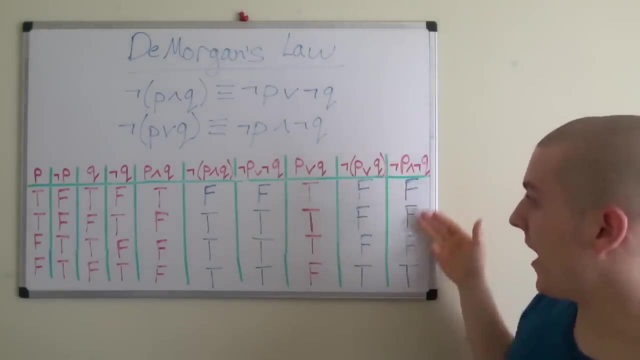 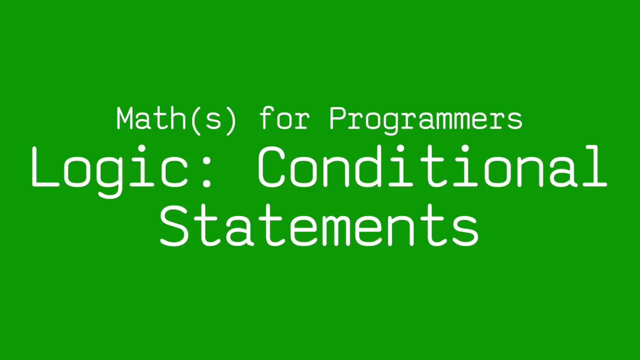 definitively say that these are logical equivalents. Also, NOT P or Q. is the is, is the? is the? in fact, not P and not Q. based on our truth table, It's 100% certain. This is logic and there's no argument against it. 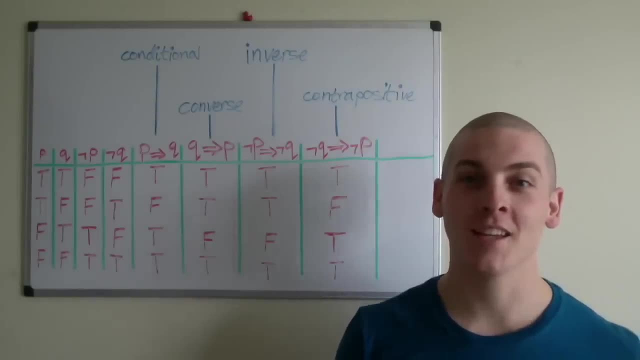 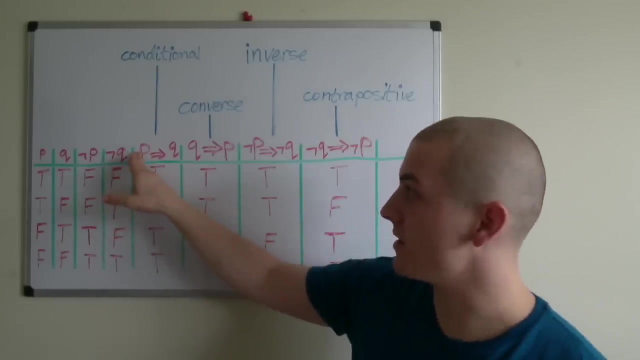 In this video, I'll be introducing the notion of conditional statements. A conditional statement contains a hypothesis and a conclusion. These are more formally known as an antecedent and a consequent. So all this is saying is that, when we look at the actual conditional, this is the 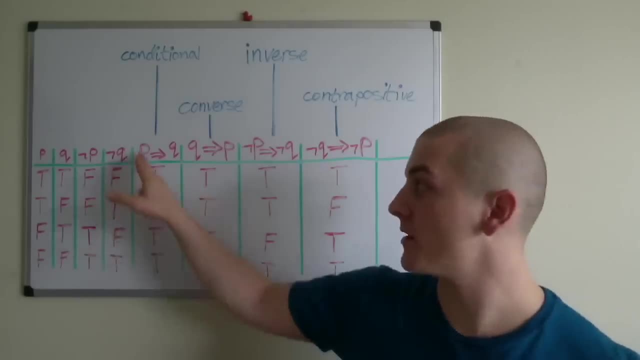 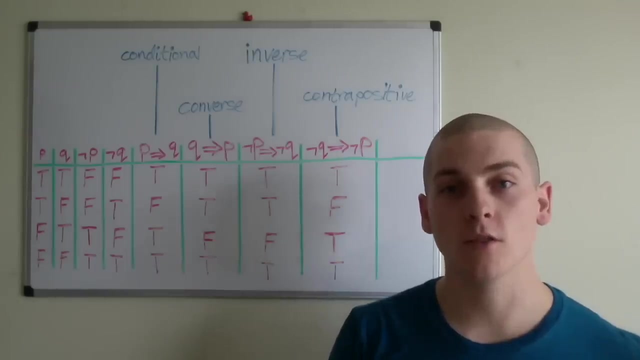 hypothesis and this is a conclusion. So this is read as P implies Q and also as if P then Q. So P implies Q is only false when a hypothesis leads to a false conclusion or an antecedent leads to a false consequence. So that's why we have 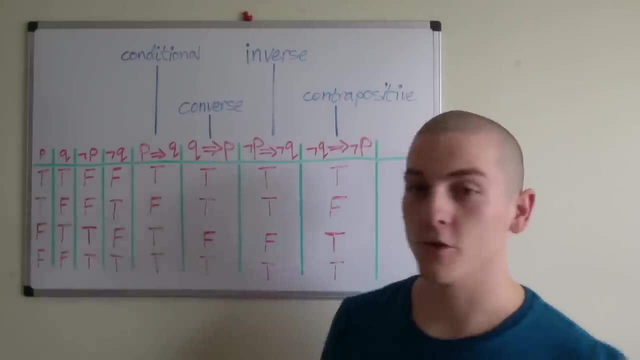 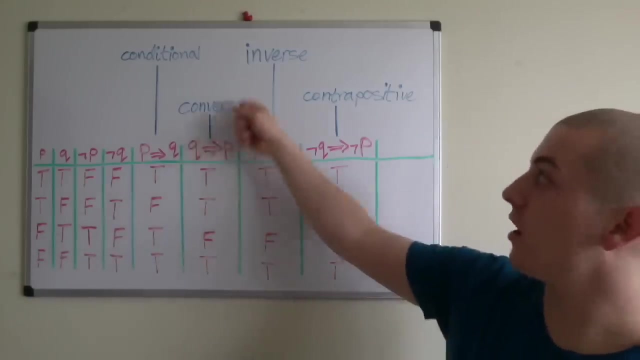 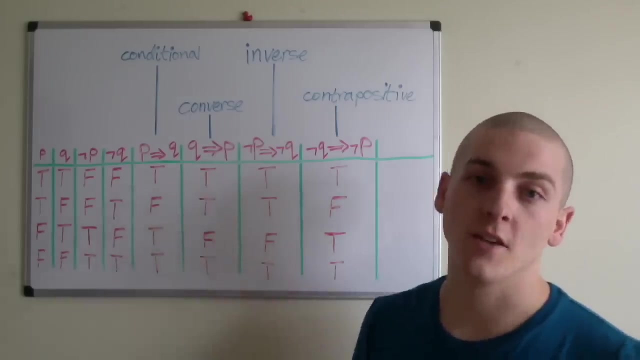 if we have true implies true, that leads to a true statement, And if we have true implies false, that leads to a false statement. These other three- converse, inverse and contrapositive- are essentially just common implications that we run into or common conditional statements that we run into. 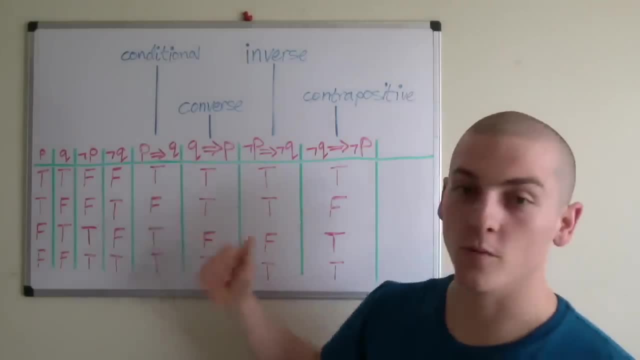 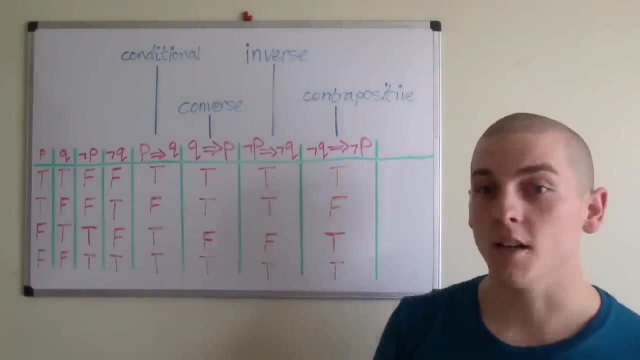 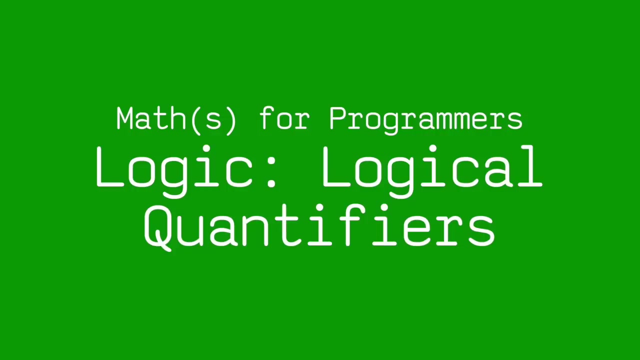 And the converse is simply: Q implies P. Inverse is not P implies not Q And not Q implies not P, which is contrapositive, is logically equivalent to the original conditional statement. In this video, I'll be introducing the universal and existential quantifiers. 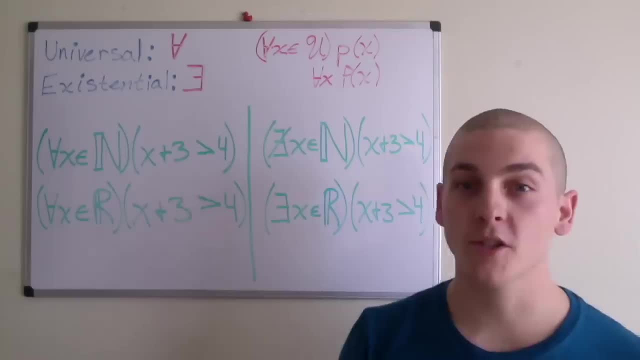 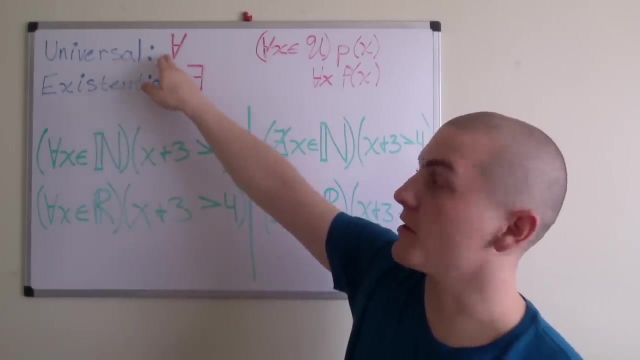 But first I have to introduce the propositional function. The propositional function denoted P of X takes on a value of true or false, But it takes on a value of true or false for everything that you feed to it. So in this case, with the universal quantifier, this is read as for every: 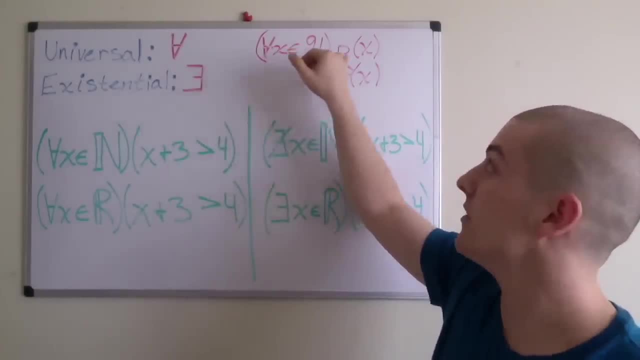 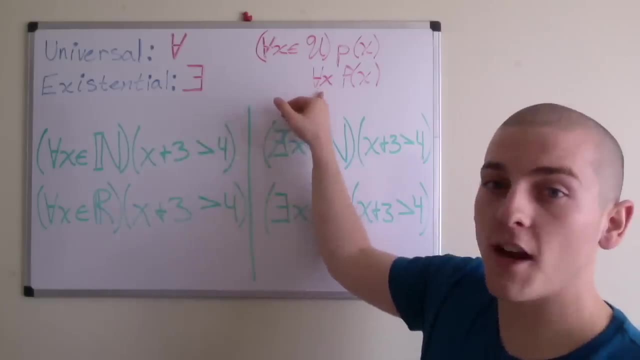 you would say: for every X. that is an element of the universe. P of X is either true or false. For every X, The shorthand for this is: for every X. P of X, You could also say there exists. that's the existential quantifier. 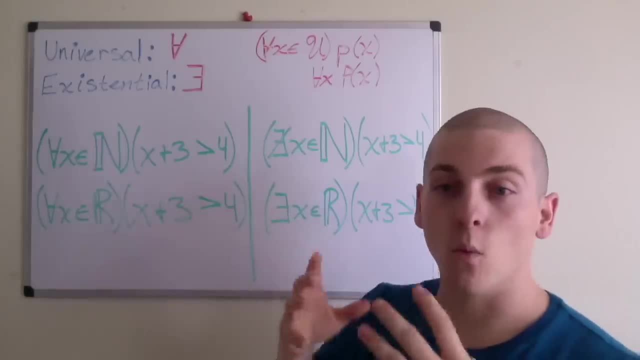 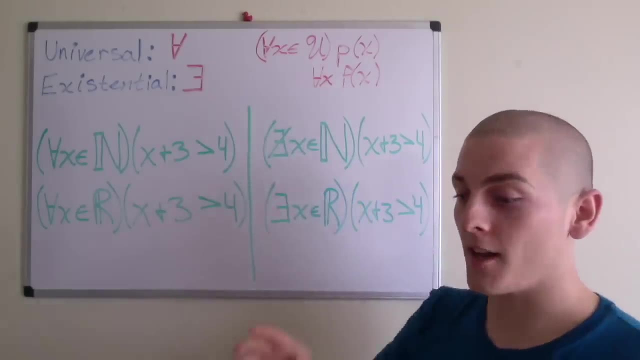 there exists is just stating that there is at least one. So if we say there exists an element, there exists an element, there exists an element, there exists an X, that is an element of the universe, we're saying there is at least one X. 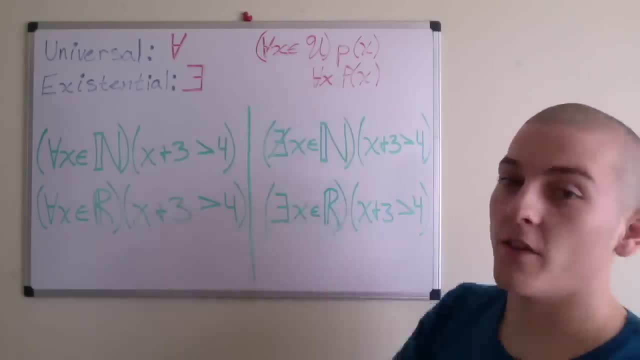 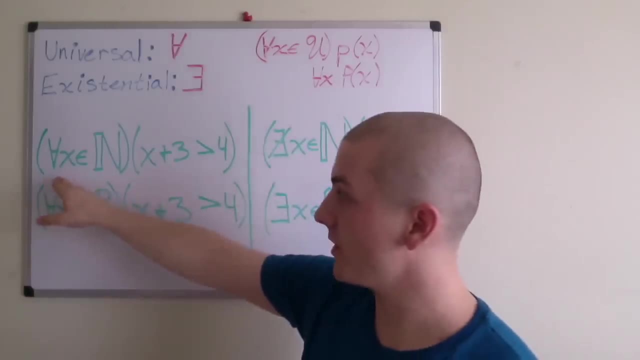 at least one X that is an element of the universe, such that P of X is true or false, And you can again use the shorthand- there exists an X, P of X. So when we look at these examples, for every X that is an element of the naturals, 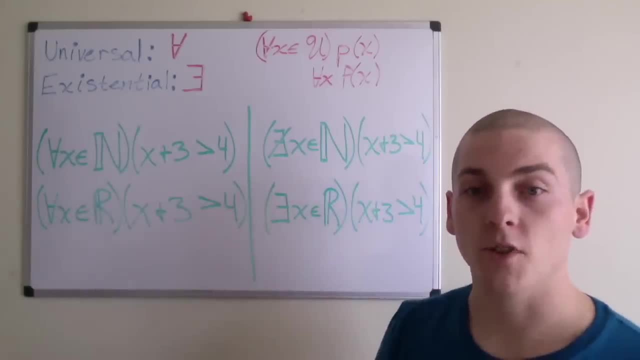 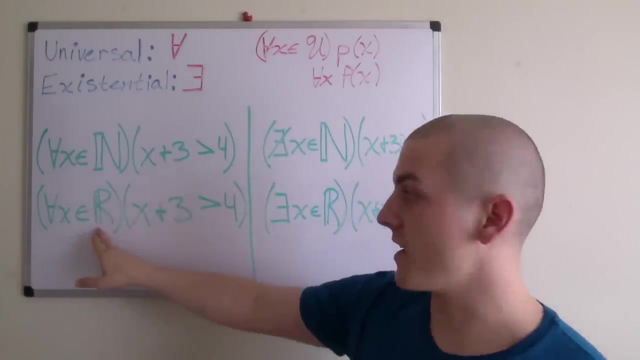 X plus three is greater than four. So that is a false statement, because the first value of the natural numbers is one. so X plus three is four, which is not greater than four. Also, for every X, that is an element of the real numbers. 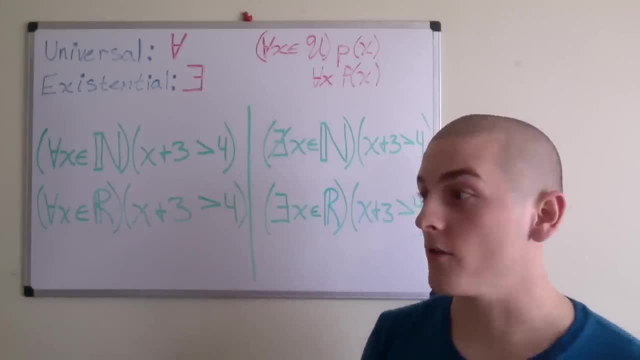 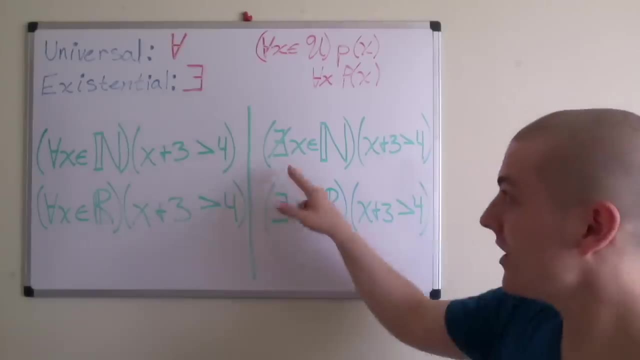 X plus three is greater than four. That is also false. I can think of. well, there are infinitely many numbers that are not true for this. And then, in this case, I said there does not exist an X. that is an element of the naturals. 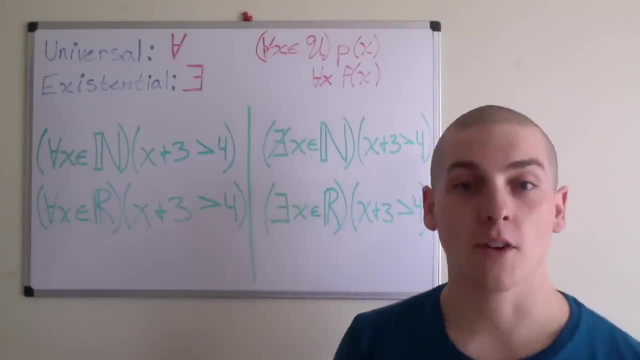 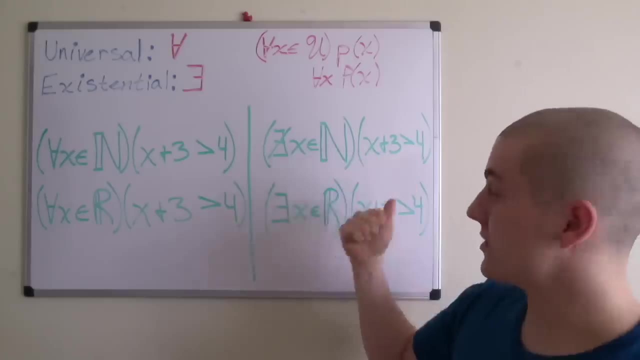 such that X plus three is greater than four. And that is also a false statement, because if I, if I let X equal two, that two is a natural number and two plus three is greater than four. So this is a false statement. 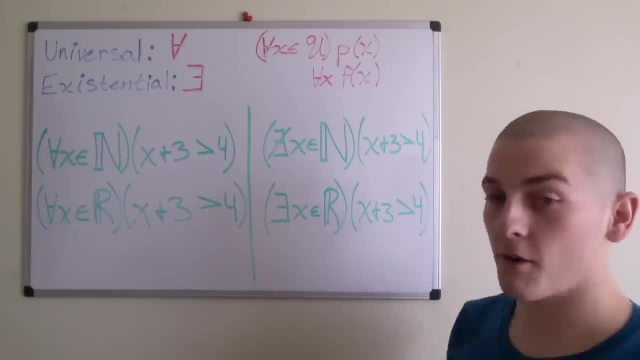 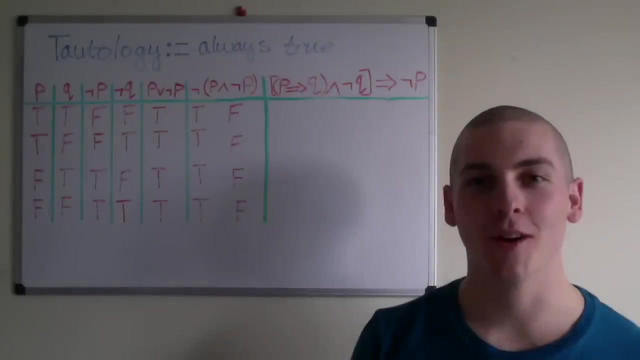 There exists an element of the real numbers such that X plus three is greater than four. That is a true statement, because any number greater than one is gonna yield a true statement. in this case, In this video I'm gonna be going over. 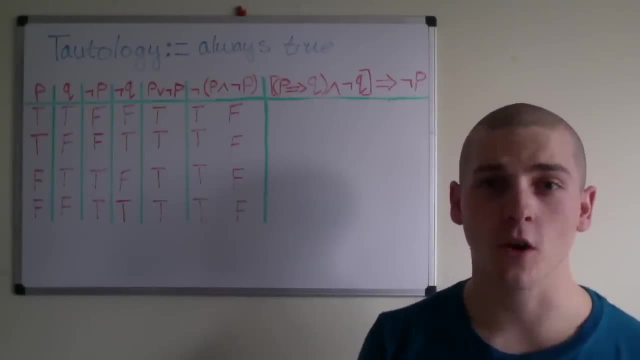 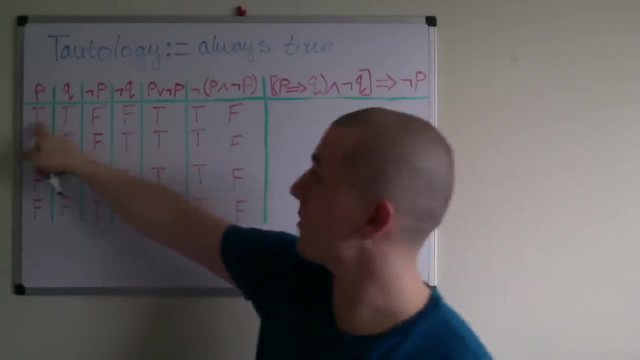 some examples of tautologies. Tautologies are simply propositions that are always true. The first one is the law of excluded middle, which is P or not P. So for here we have P or not P, So true or false, true or false. 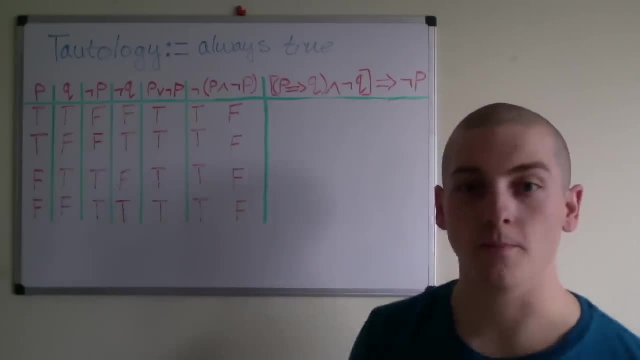 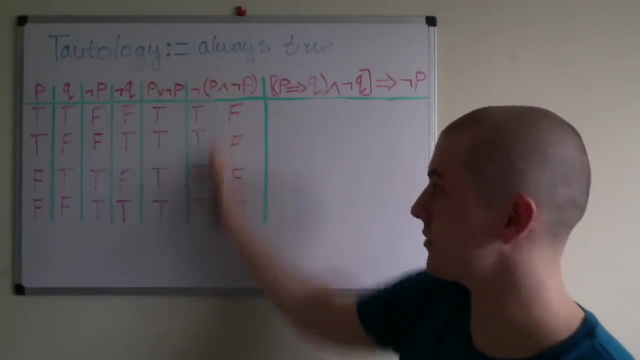 false or true, or false or true, which yields nothing but a true column. Next, we have the law of contradiction. So if you ignore this negation, here, in this column of trues, here we have P and not P. So true and false yields false. 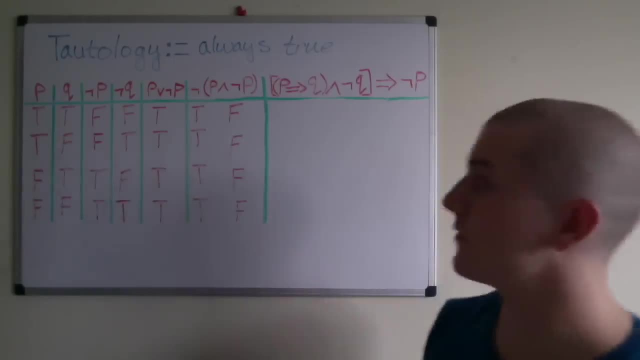 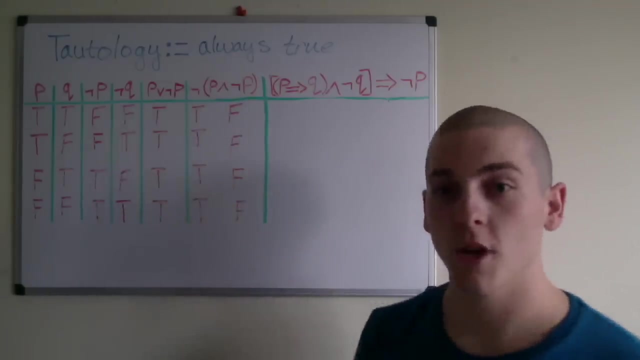 True and false yields false. False and true, false and true: all yield false. Now, when we actually apply this negation to the false column here, that yields a column of trues. So the law of contradiction is a tautology. 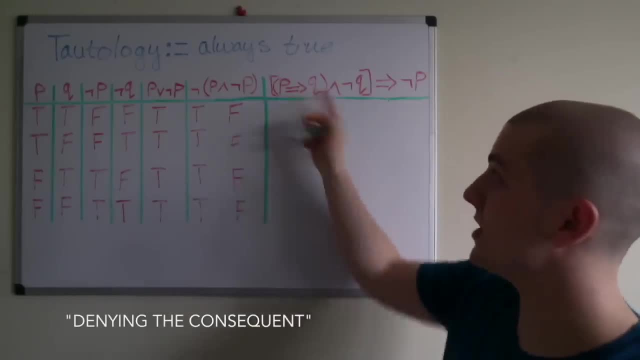 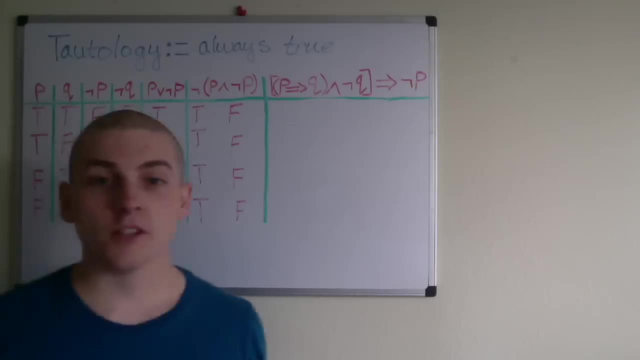 Finally, we have modus tollens. Modus tollens is P implies Q and not Q implies not P. So let's break this down: P implies Q, P implies Q is only ever negative when the hypothesis predicts true and the conclusion is false.